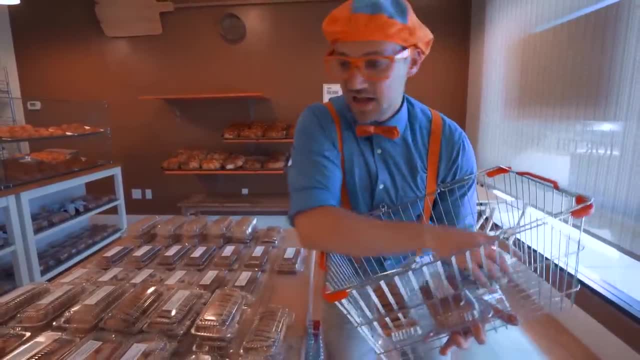 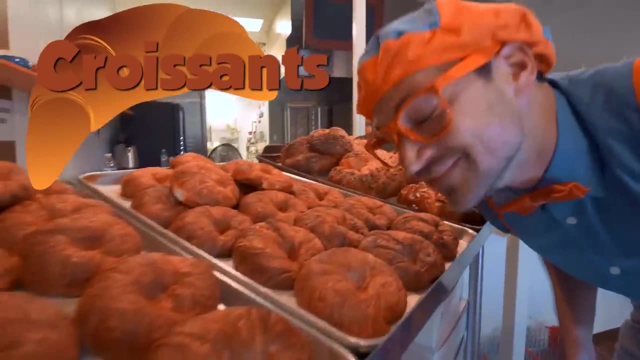 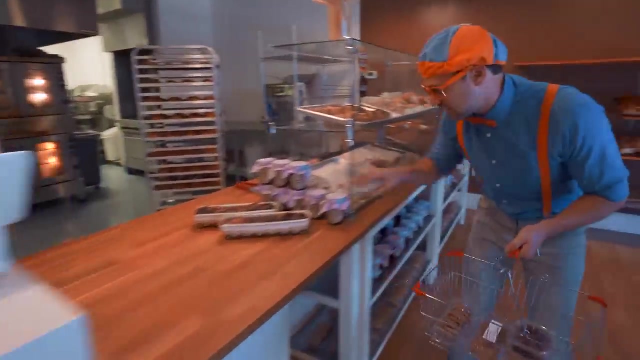 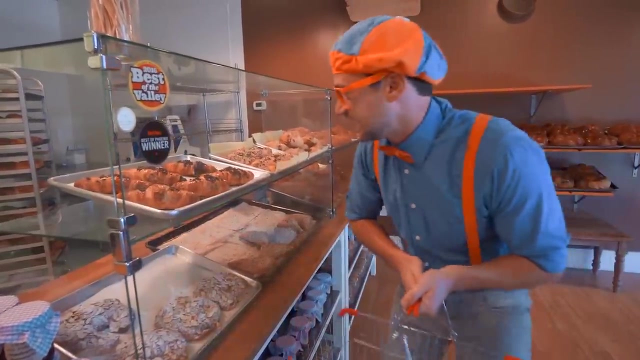 Whoa, ooh, Yeah, this all looks so good. Ooh, and croissants right here- Ah, they smell so tasty. Whoa, Whoa, check this out. Strawberry marmalade- Wow, that's really fresh and really tasty. 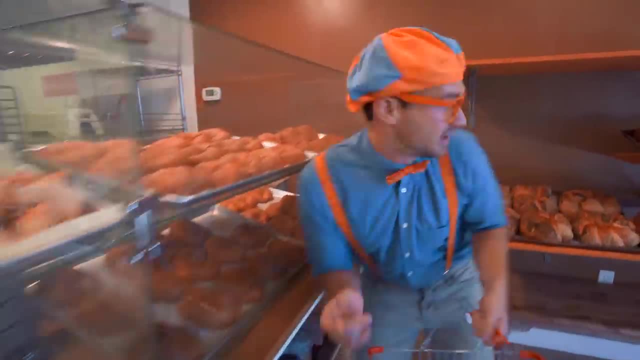 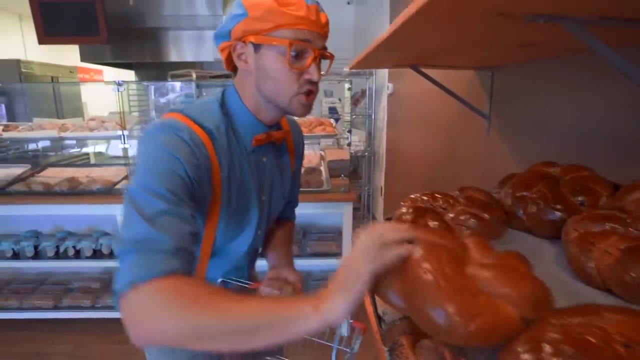 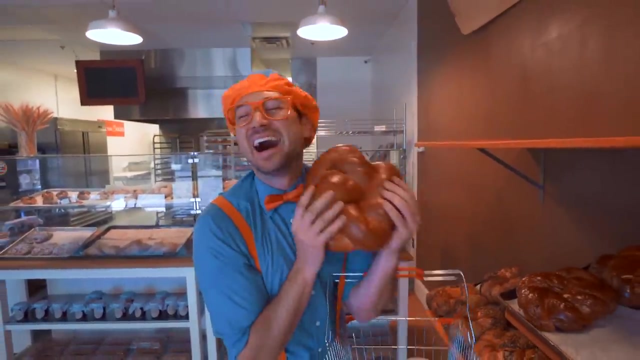 Okay, let's see what else would we like? Whoa, Look at how big these are. Geez, look at that. That is massive. We need to get this one. Ah no, Oh, okay, let's put that in our basket. 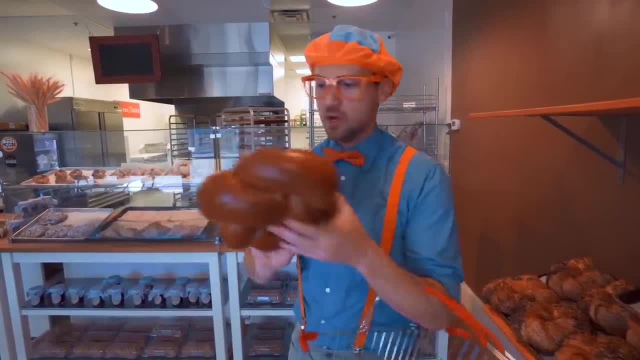 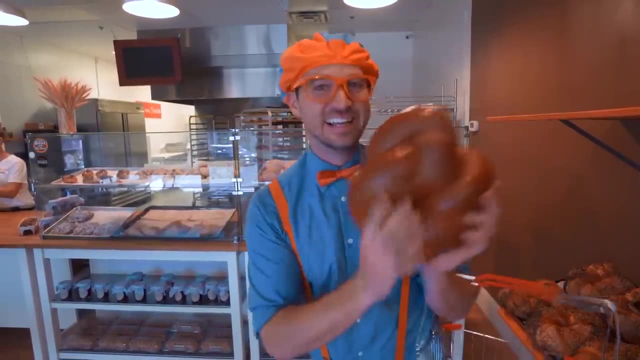 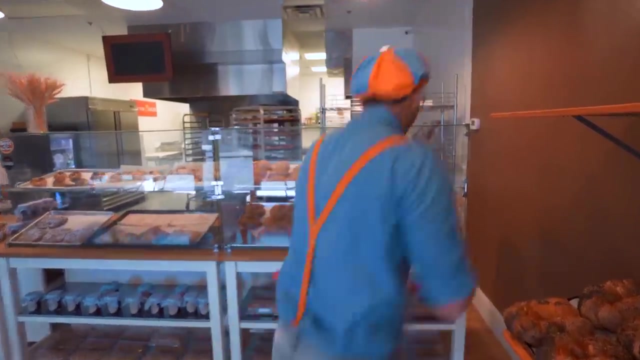 Hey, wait a second. Have you ever wondered how bread products like this are baked and made? It's so big and pretty. What are we doing out front? Let's head in the back and bake some stuff today Let's go. Ooh, now we're in the back of the bakery. 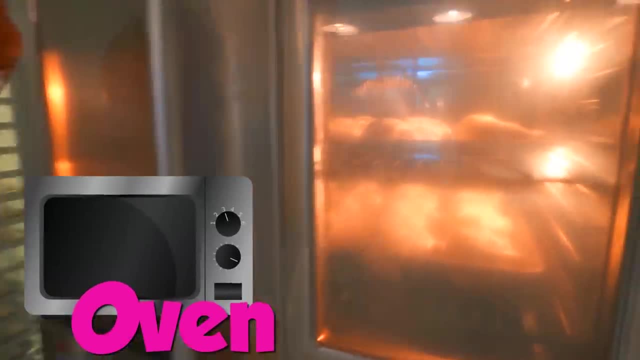 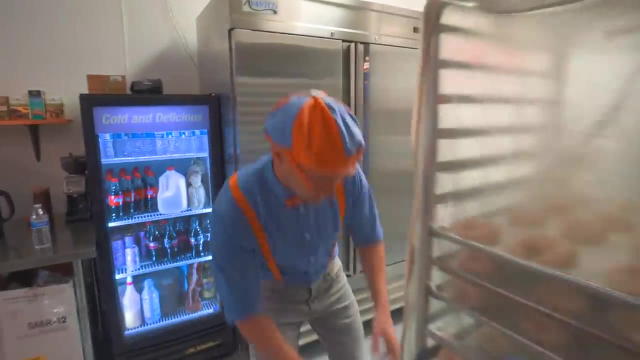 Whoa, look An oven. Ooh, Ooh, there's some tasty treats baking in there. Ooh, I'm excited, Whoa, And look at this. Let's open it up and see what's inside. Whoa. 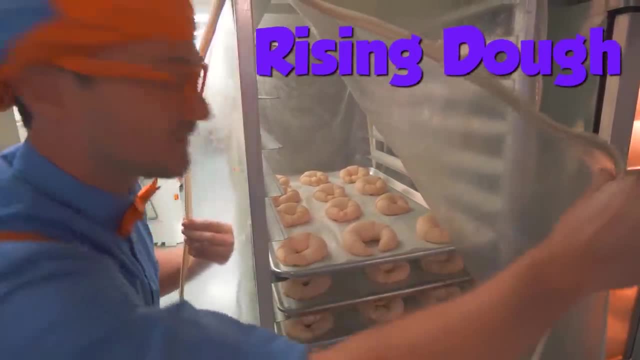 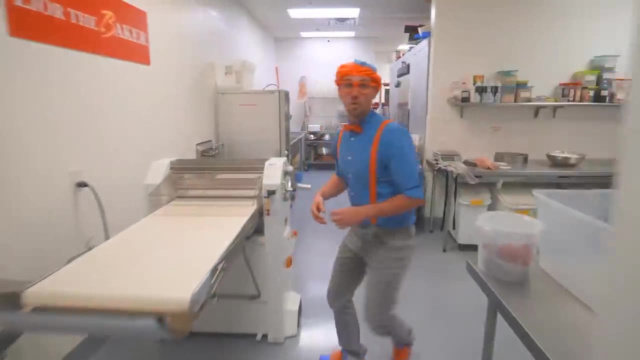 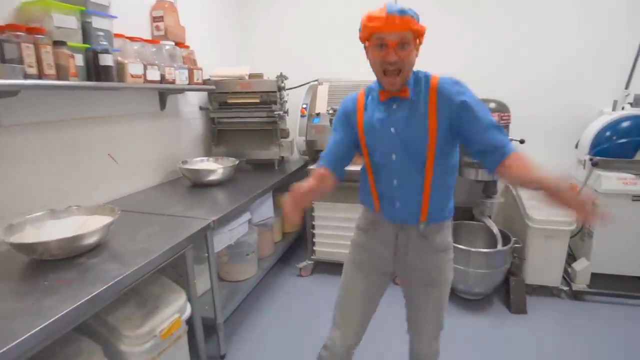 Hello, That's rising dough. Whoa, that dough looks tasty. Okay, let's close it back up. Come back here. Whoa, This room is where the baker is always at Working along. Ha, Making tasty treats, Haha. 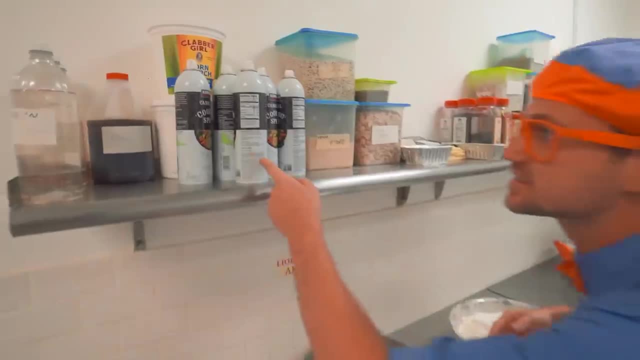 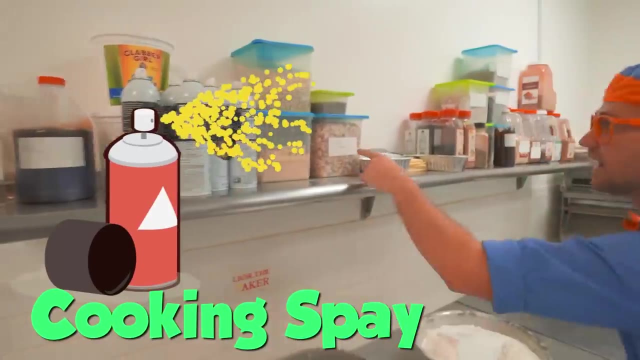 Okay, let me show you around. Whoa, look at all of these ingredients. Whoa, we have some honey. Yeah, Honey's tasty. Ooh, cooking spray. Sliced almonds- Whoa, And look, whole almonds. 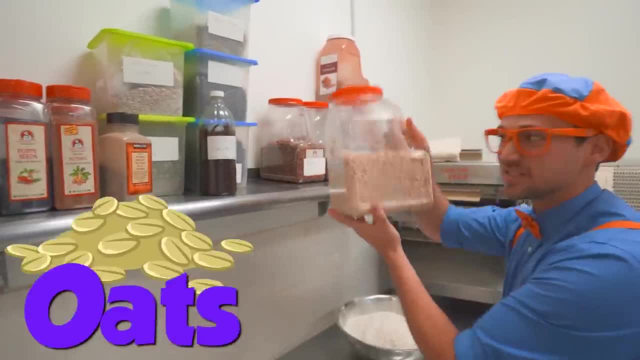 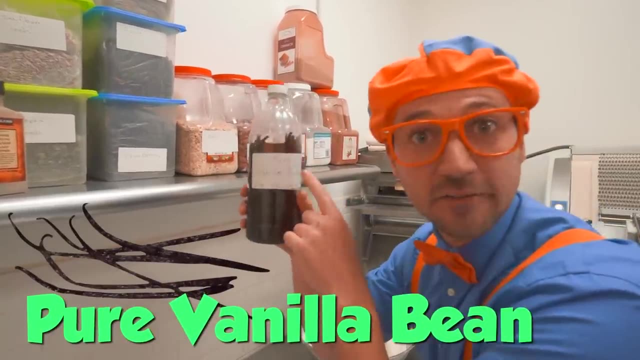 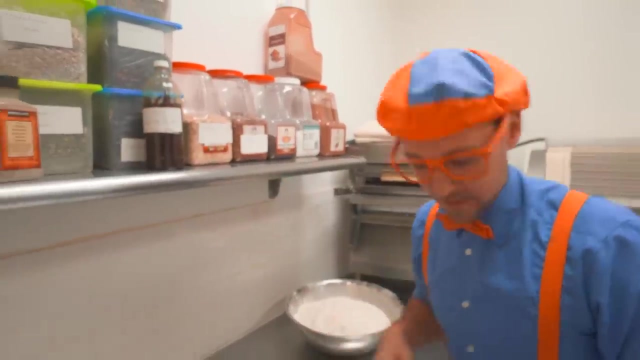 Wow And oats, Kind of like the stuff you have in the morning sometimes. Haha, Whoa, Oh, pure vanilla bean. No way, this stuff takes like two years to make. That's crazy. Oh, and down here, check it out: it's flour. 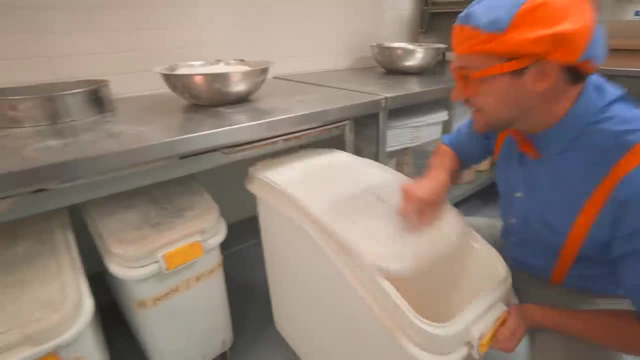 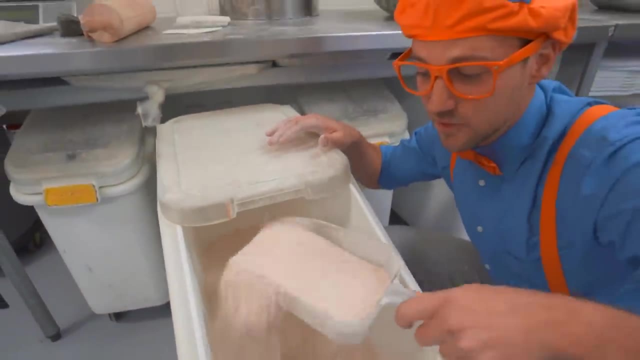 Whoa, it's so soft And there's other kinds of flour. check it out. See, this is a lot darker than the other one. The other one was white and this one kind of looks brown. Interesting, okay, let's put that away. 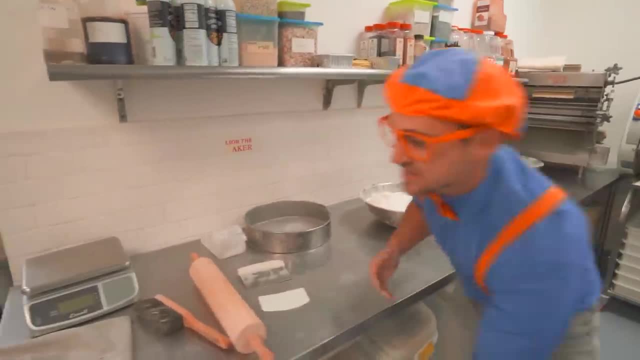 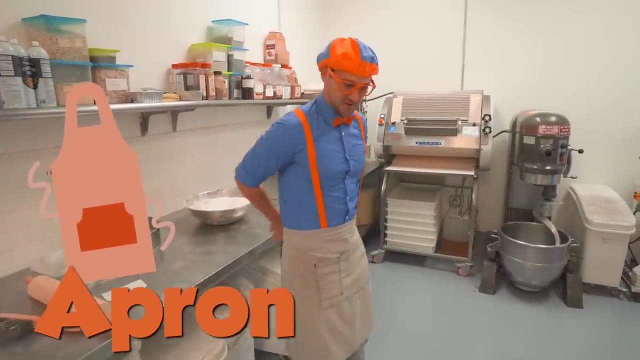 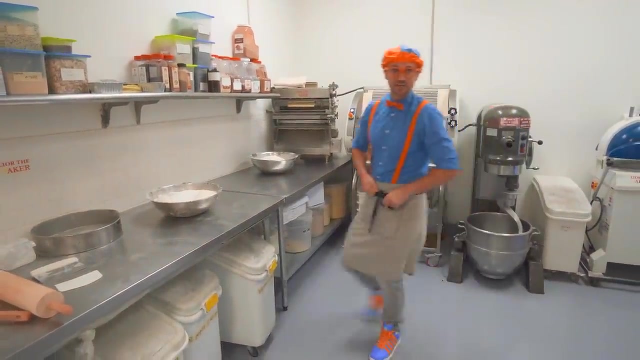 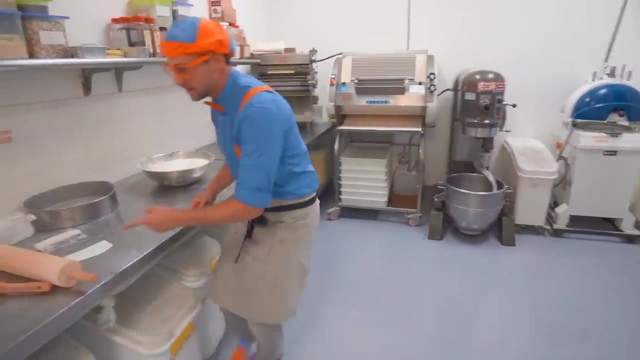 and let's get to baking. Okay, first things, first Glamoriness. let's put on our apron. Okay, all right, How do I look? Yeah, Let's do the baker's dance. Yeah, ooh, check out my tools. 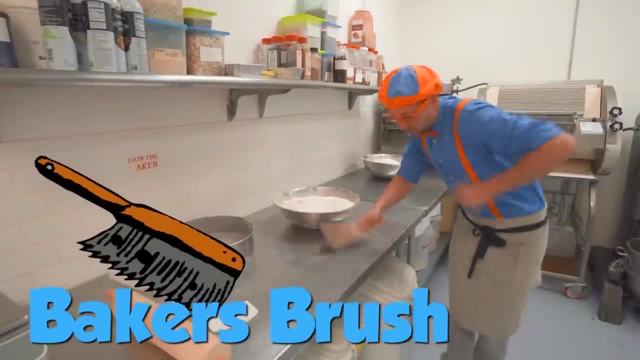 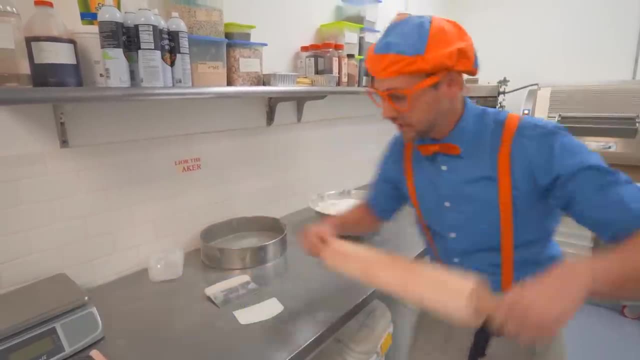 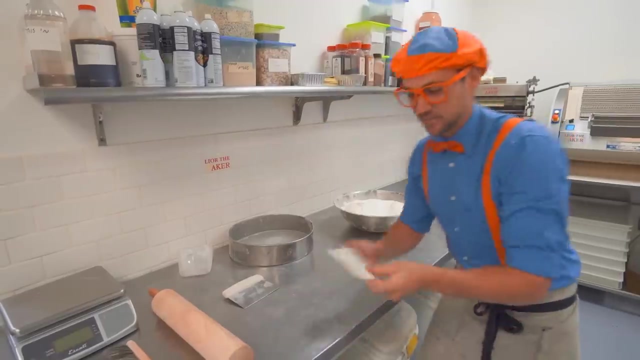 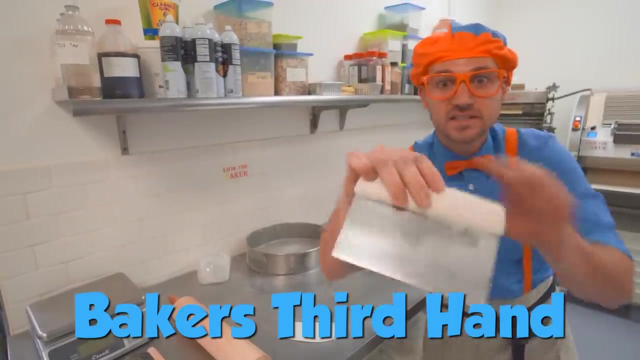 Ooh Brush, Yep, Ooh the roller, Wow, a giant rolling pin. So then you can flatten out the dough- Whoa, And a scrape, Ooh. and the baker's third hand, Whoa. doesn't that look interesting? 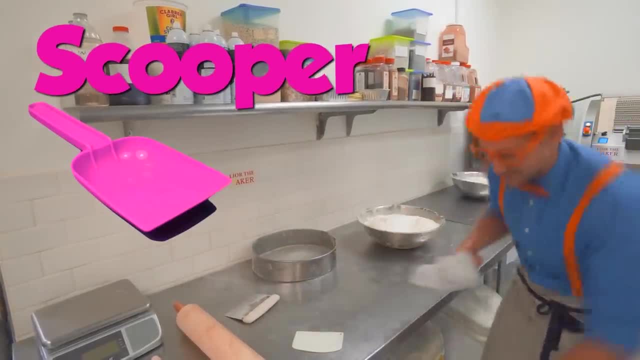 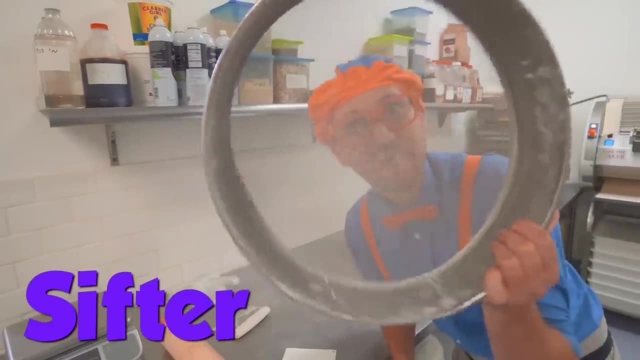 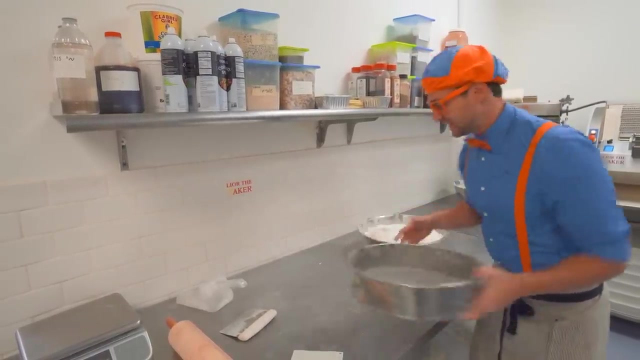 Whoa and a scooper: Yep. So then you can get a bunch of flour. Oh, a sifter. Whoa, hello. You put the flour in there and then it aerates it and then it makes it nice and fluffy. 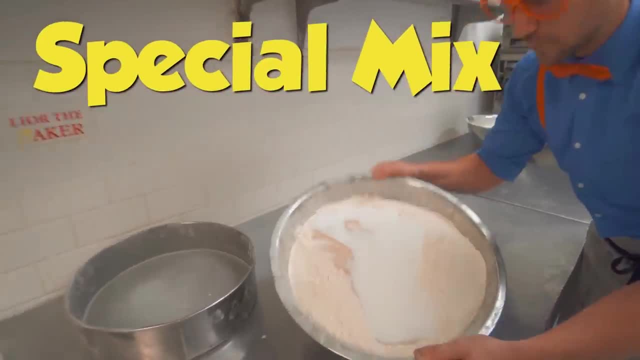 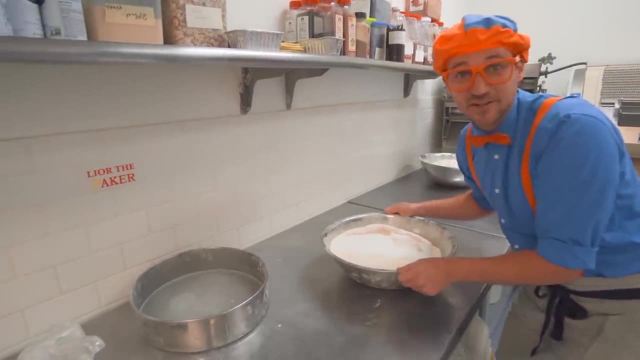 Okay, check this out. This is special mix, Whoa. I can't tell you what's in there. You'll have to come here and check it out and taste it for yourself. All right, let's mix it up, Whoa. 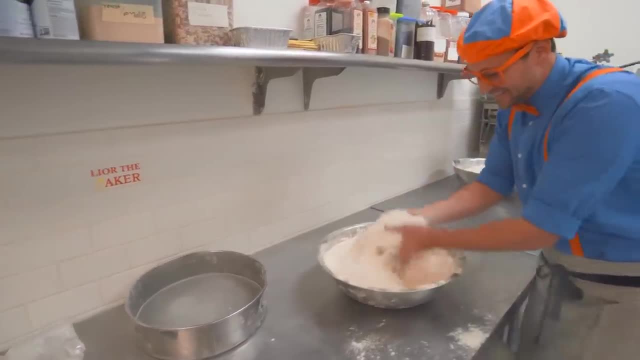 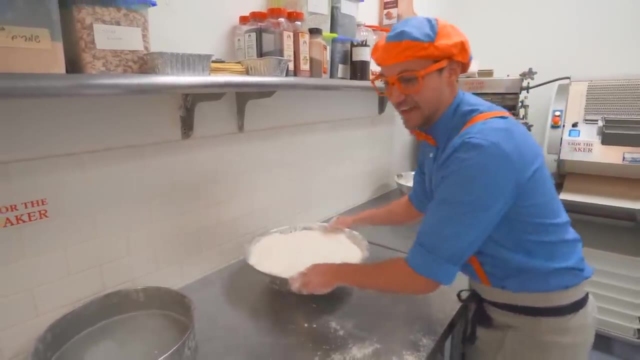 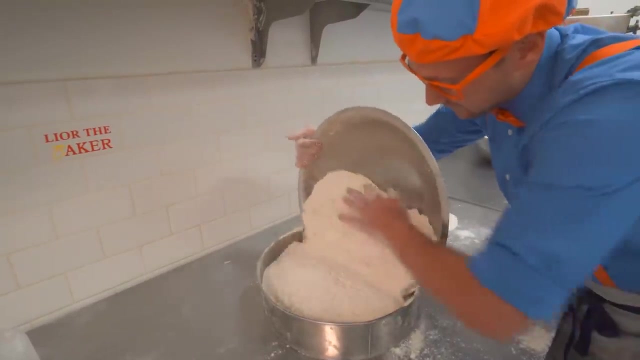 Whoa, Whoa, Whoa Feels so good. Whoa, my hands are all floury. Okay, check this out. Okay, let's put it right in the sifter. Let me show you this: Whoa. 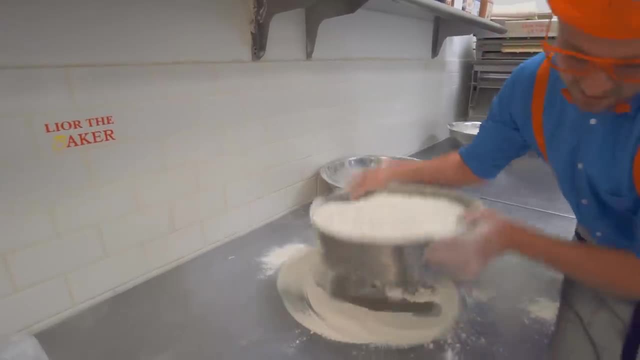 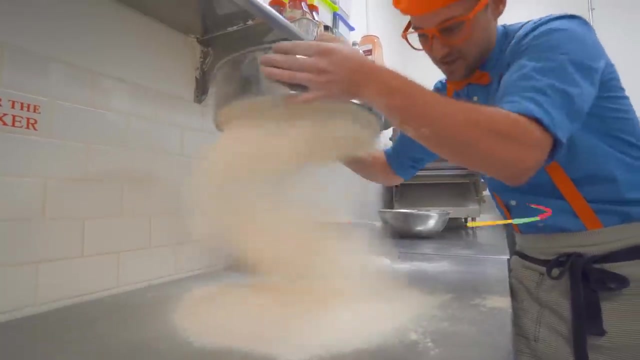 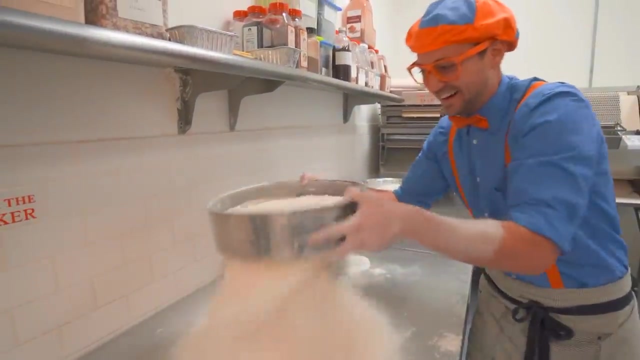 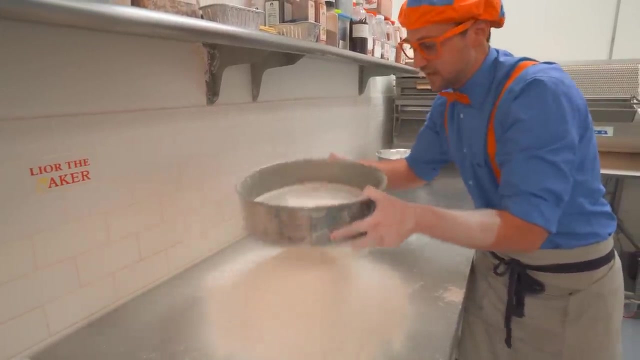 Wee. All right, watch this Whoa. It's like it's raining special mix: Whoa, whoa, whee, whoa, just a little bit more whoa. all right, now it's nice and fluffy. 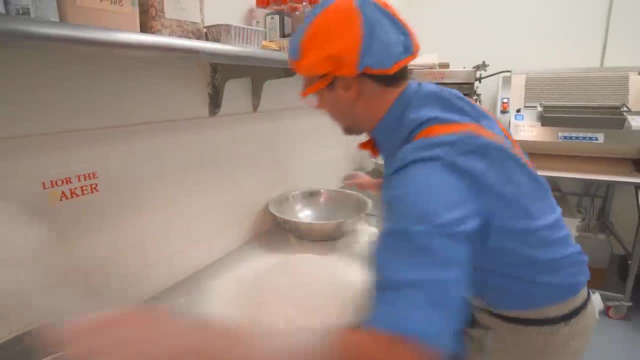 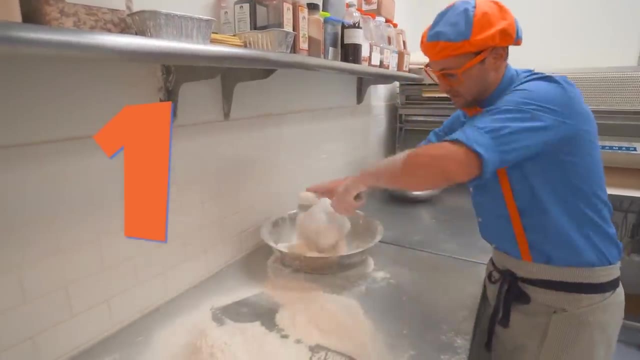 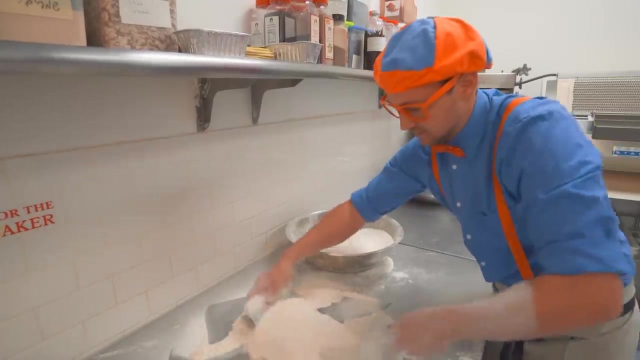 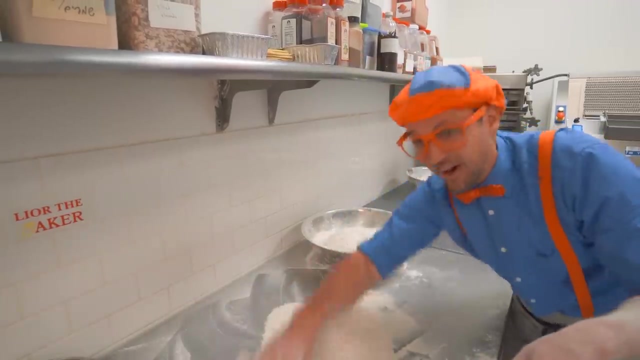 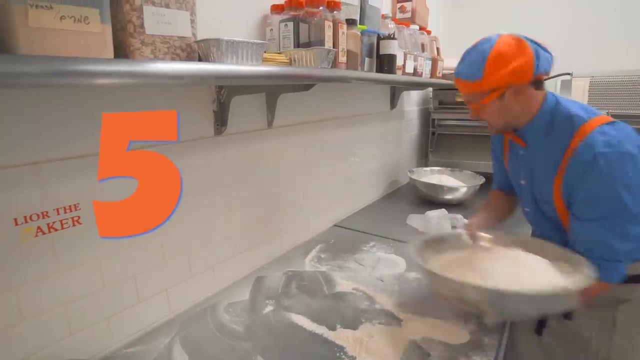 there we go. so let's put it back in the giant bowl. all right, there we go. one scoop, two scoops, three scoops, four scoops, five scoops, five scoops and a little extra. so let's. 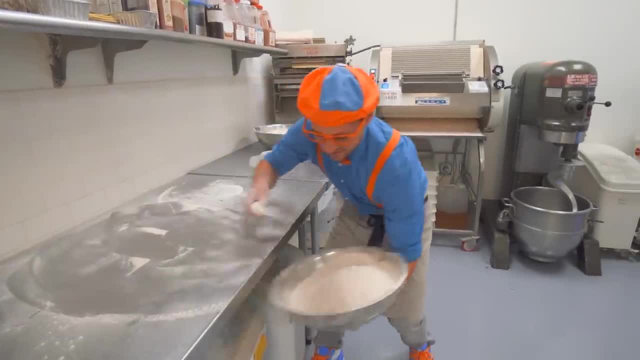 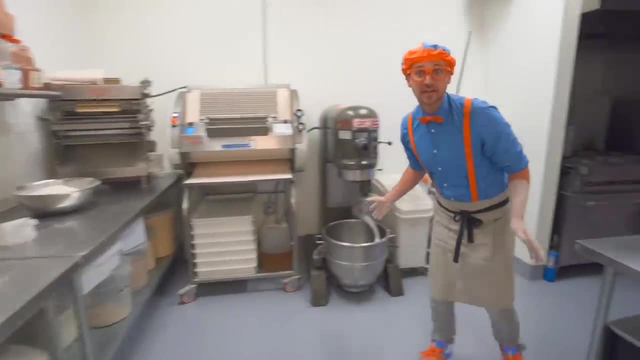 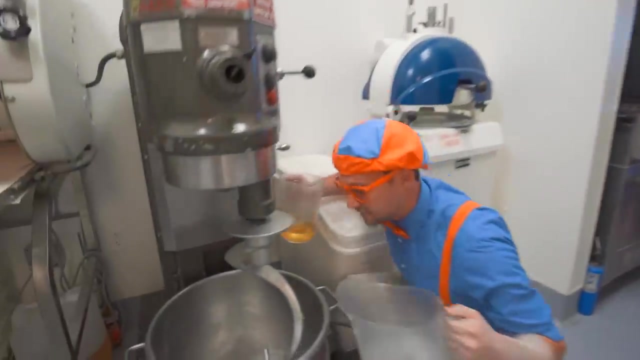 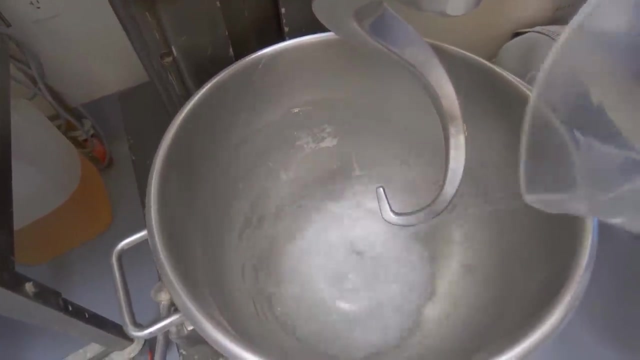 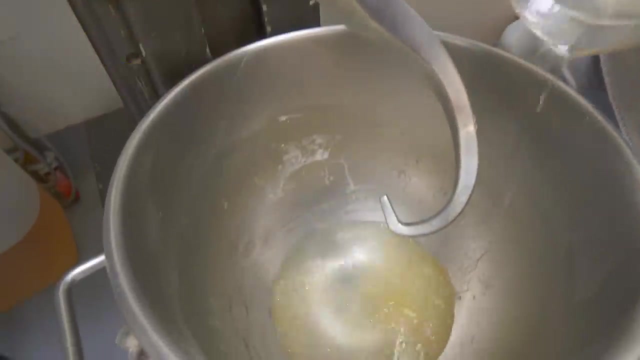 call it five and a half scoops. all right, now that it's nice and fluffy, let's put it back in the giant bowl. all right, now, it's nice and fluffy, let's put it back in the giant bowl. all right, now that it's nice and fluffy, let's call it five and a half scoops. 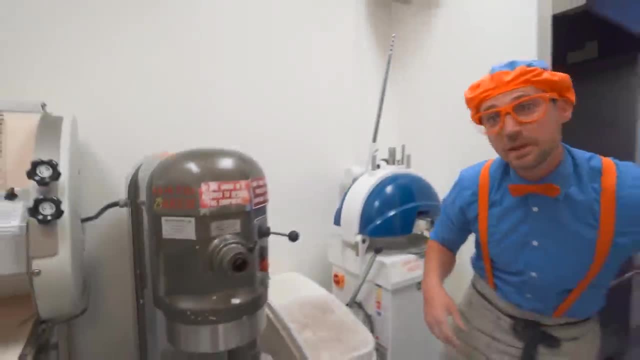 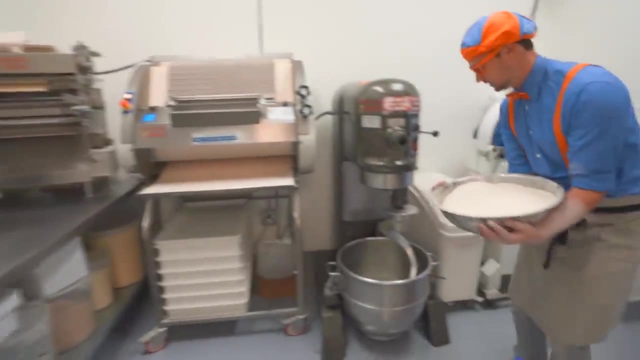 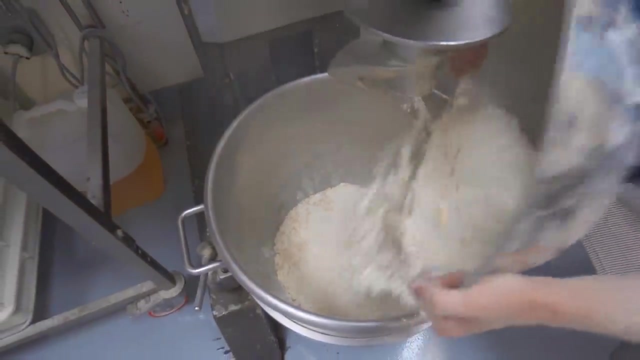 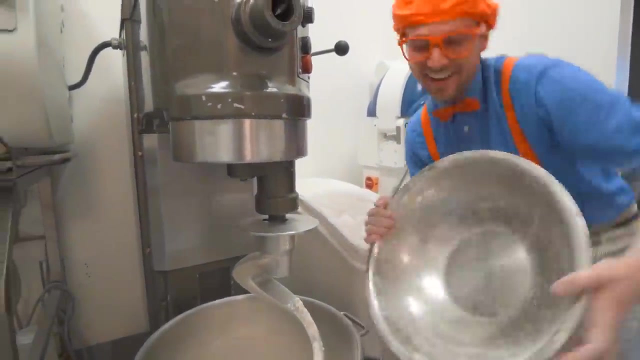 that looks silly. okay, now let's get the special mix. okay, here it is whoa, it's really heavy. okay, all right, let's put it in there. here you go. okay, all right, let's. 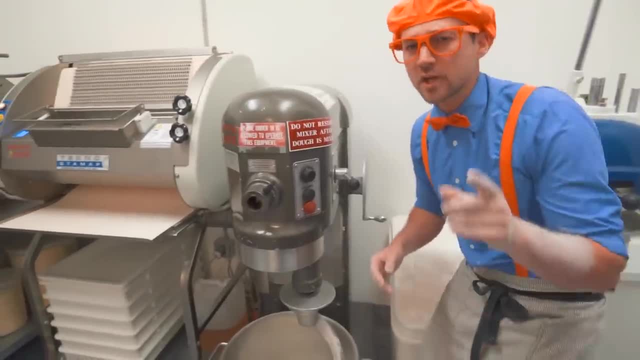 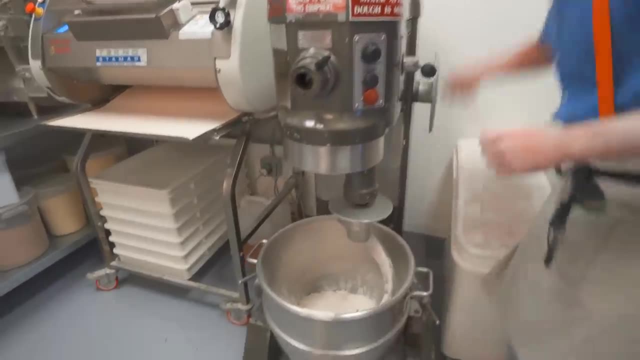 get the special mix. okay, we need to roll it up and pick a speed. do you want to go slow or fast? I think fast. okay, first let's roll it up. perfect, now that it's at the top. 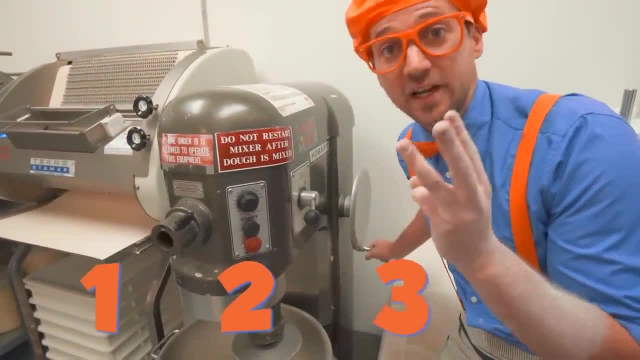 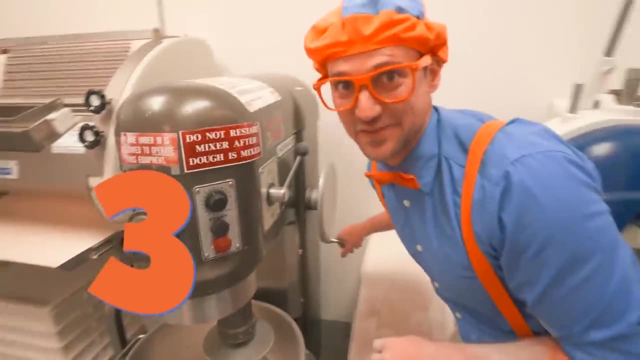 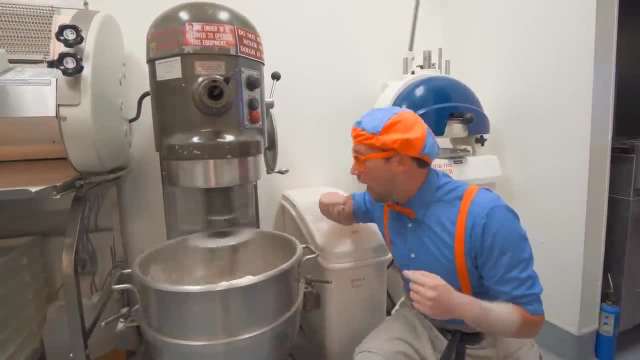 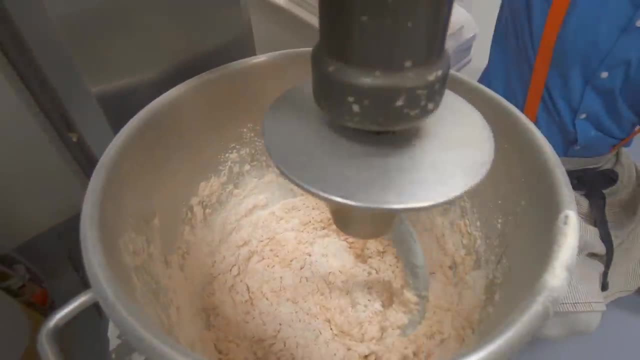 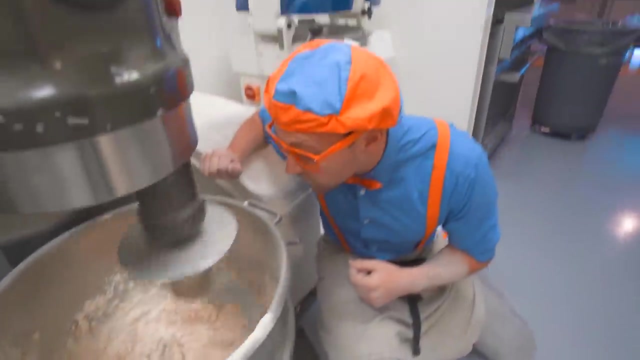 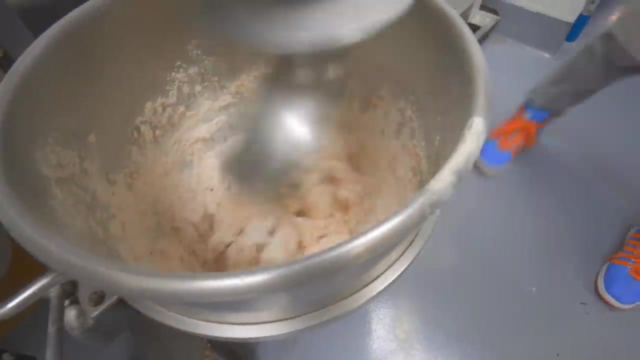 Three, two, one. whoa, look at it go. Whoa check it out. whoa, that looks so tasty. Whoa check it out. get a closer look. Okay, now the dough is all done, so we need to take it out. 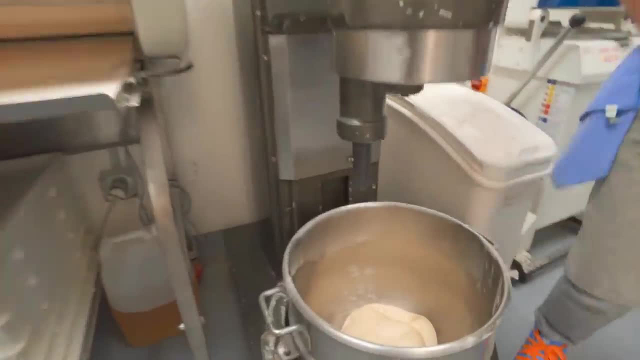 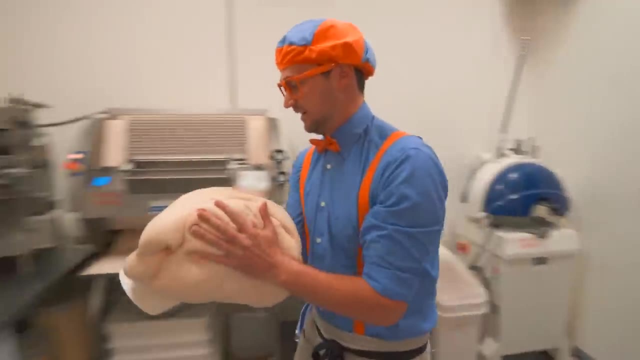 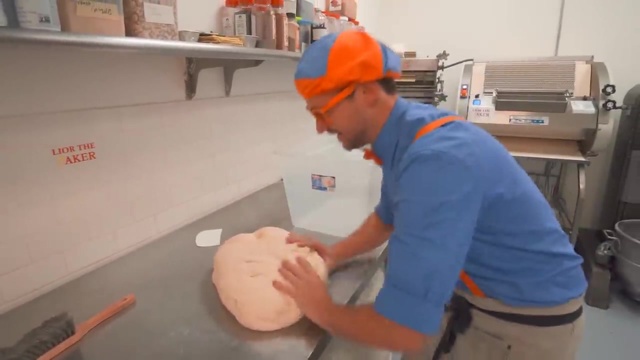 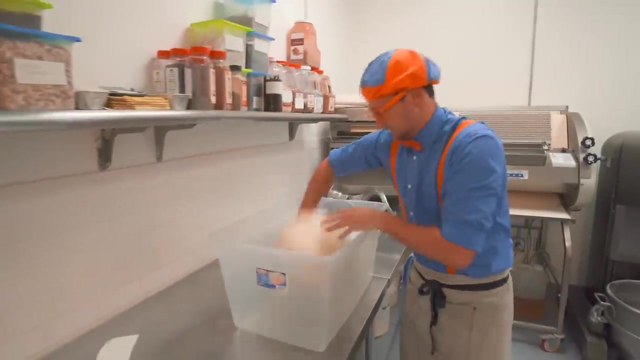 Put that big thing right there, and then let's grab our scraper. Whoa, look at it. okay, All right, knead it a couple times, perfect. Okay, now let's put it in this tote and then put this right there, perfect. 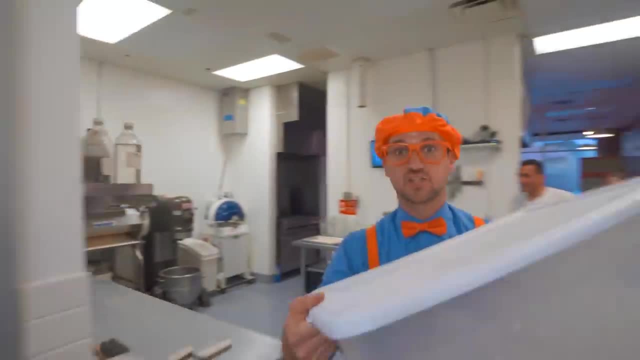 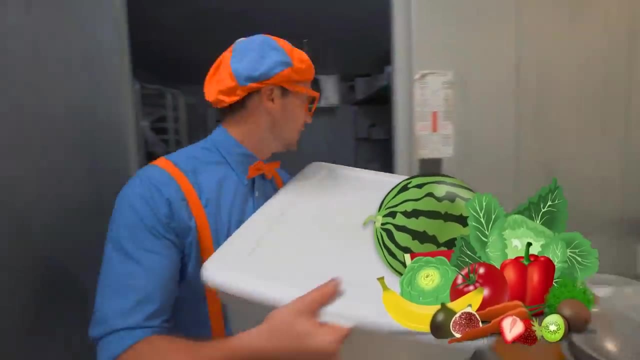 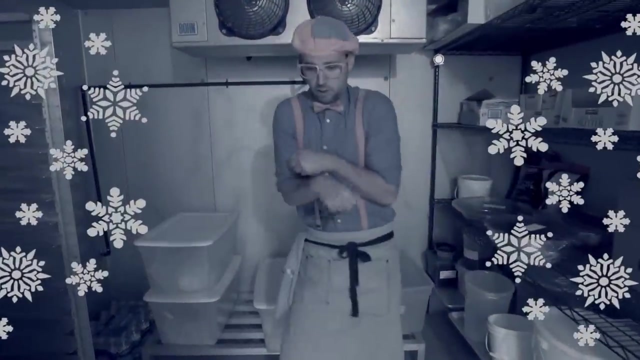 Now we need to put it in the fridge. and the fridge is this spot right here, Whoa, just like where you keep all of your foods, your cold foods. this is a fridge. It's really cold, brr, brr, oh, it's so cold. 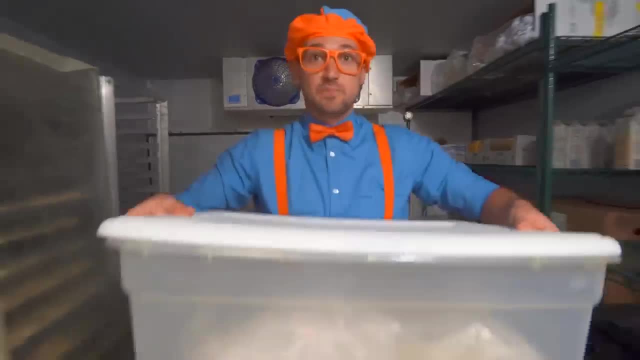 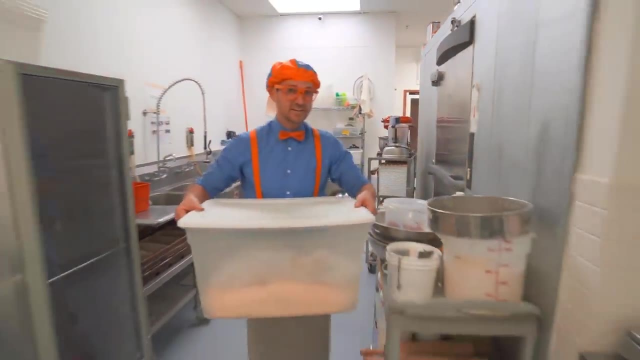 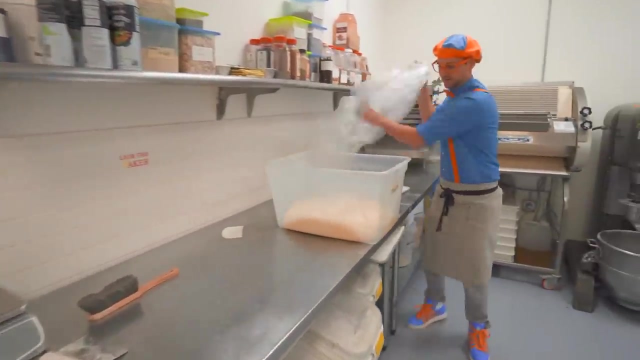 Okay, this one is ready. so this one has been in here for a little bit. so now, okay, make sure the door shuts. Perfect, and here you go, Ready, Yep, All right. okay, so ready, I'll take it out for you. 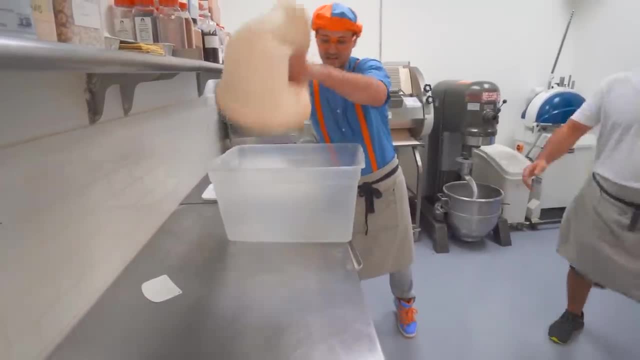 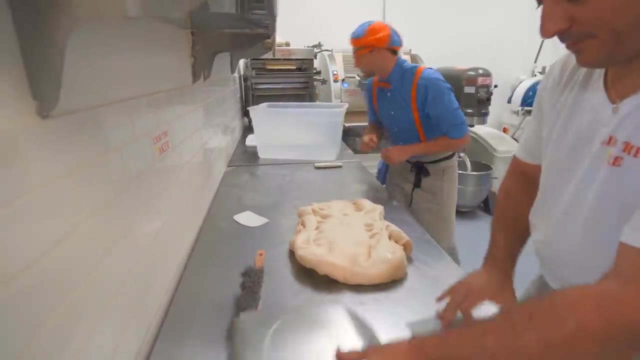 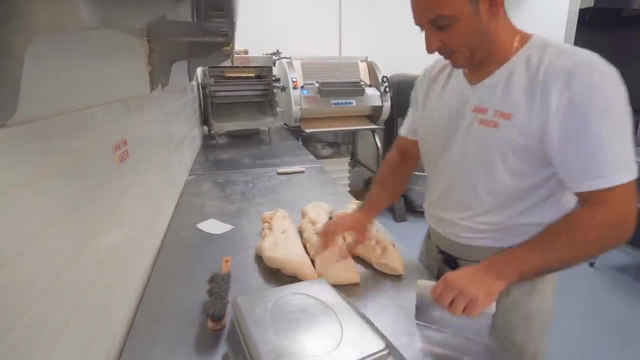 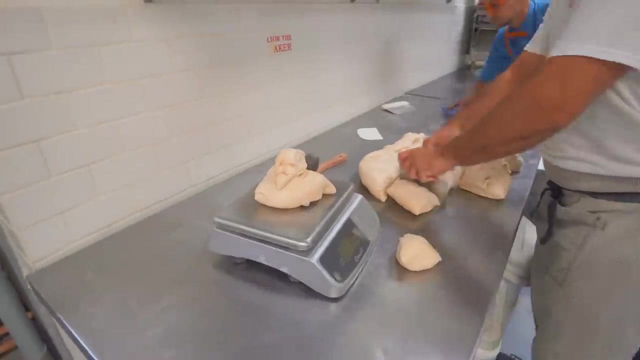 There you go, you're welcome. Okay, now he's gonna cut it into small pieces. Watch him. I'll organize in the meantime, So check it out. it's a little bit bigger. it's a little bit bigger. 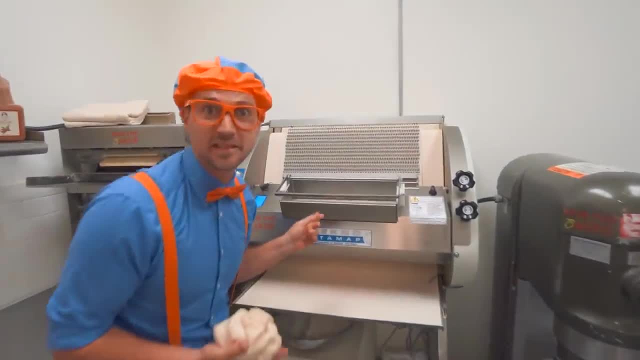 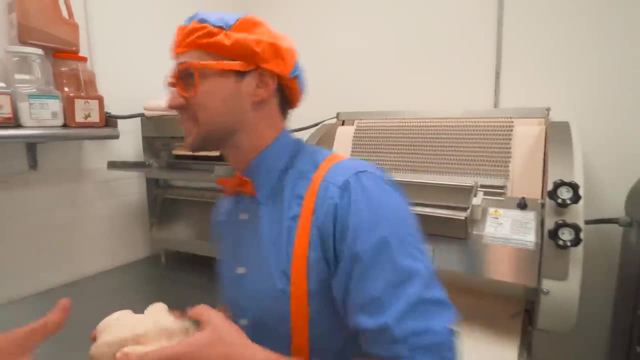 Now this one's ready, And now we're gonna put it in this machine. Okay, here we go. Uh-oh, baker, sir, can you help us? Yes, Okay, I don't know how to turn it on. 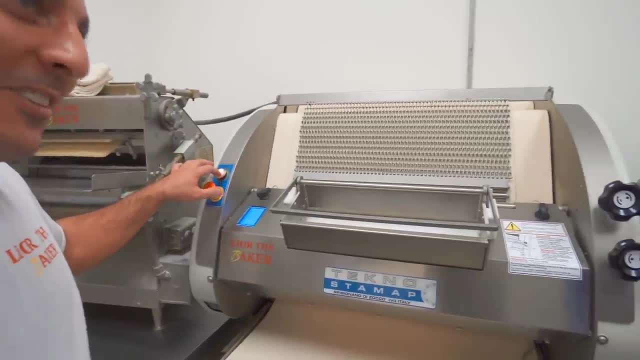 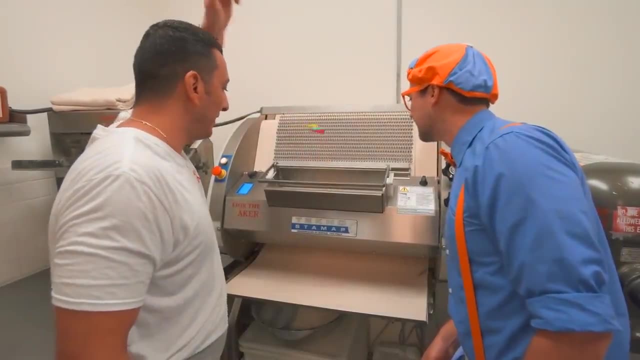 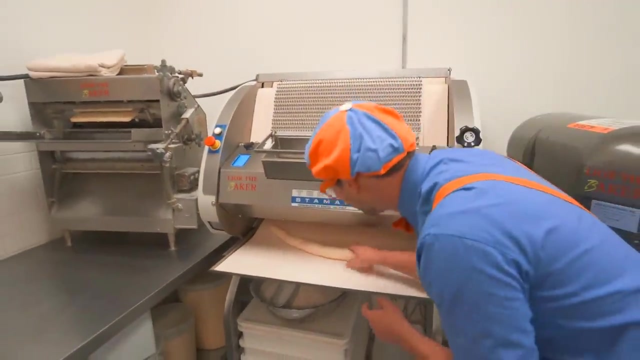 First day. Yeah, Ready, One, two, three, Whoa. okay, Now we're gonna be sure we don't put our hand inside. Ready, Okay, Oh, Oh, okay. now let's give this to him. 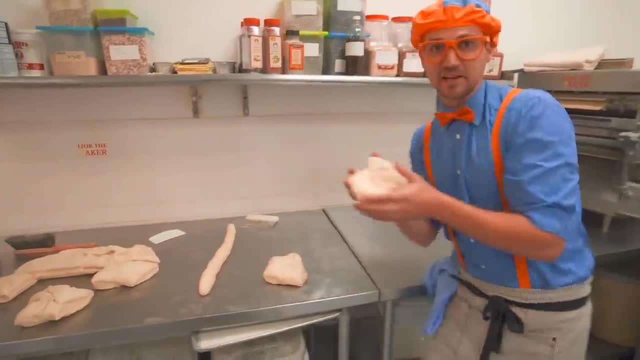 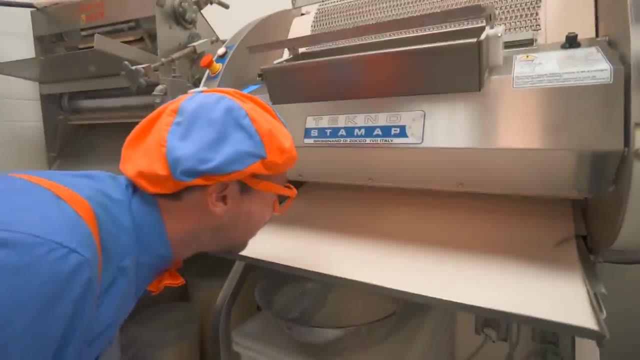 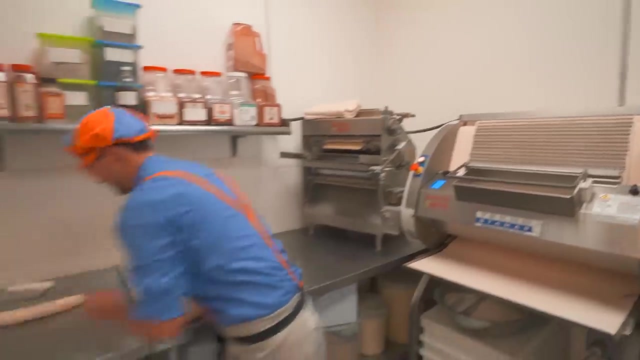 Do you want it right here? Yes, Okay, there you go. Thank you, baby, You're welcome. Okay, let's do another one. Ready, Hello, where are you? Okay, here's another one. Whoa, here's another one. 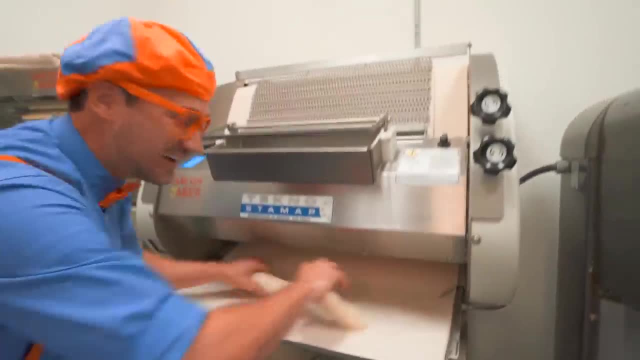 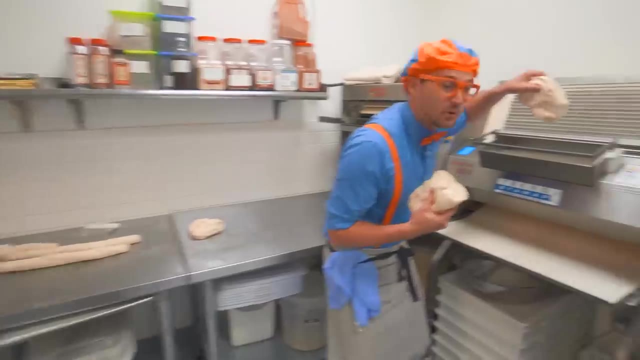 Get ready. Here's another one: Whoa, Whoa. Okay, we've done three, but it looks like I'm falling behind. I need to go quicker. Let's put one in. Let's wait a little bit. Okay, let's put another one in. 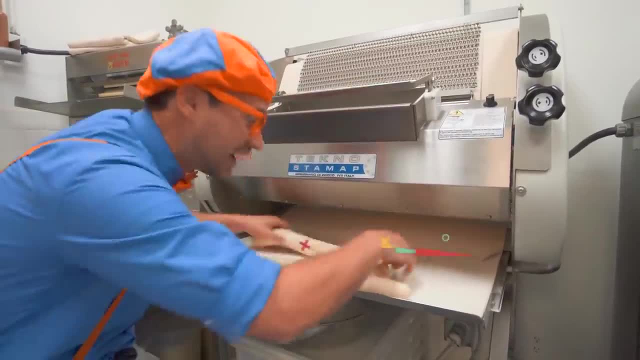 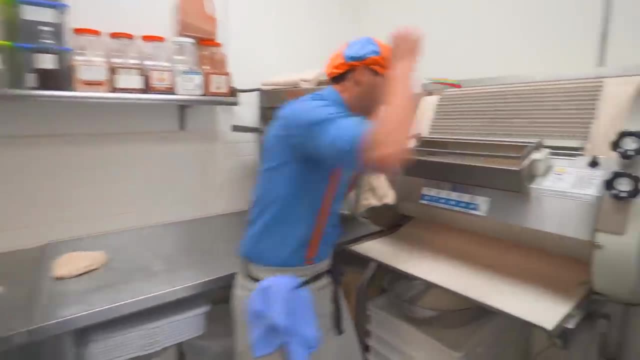 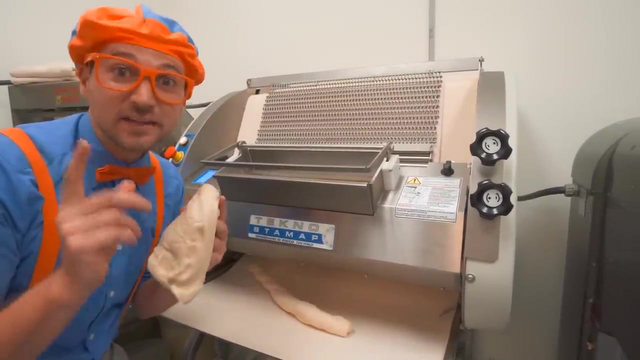 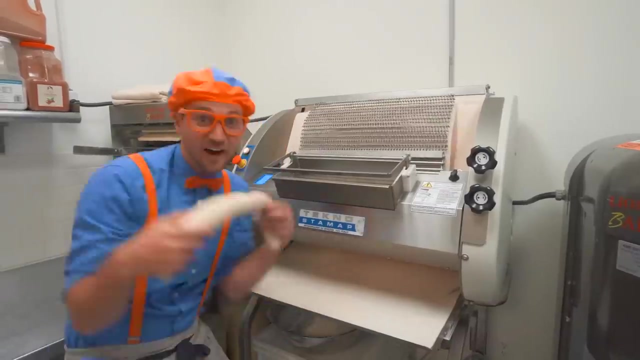 Okay, perfect, Here's one, And here's two. Okay, here's one, Here's two. Okay, here's some more. Okay, three, two, one, Three, two, one, Three, two, one. Oh jeez. 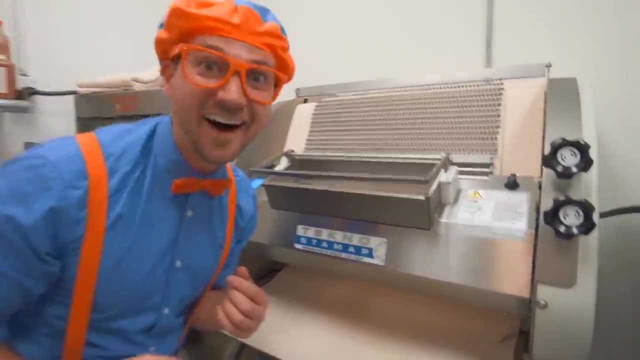 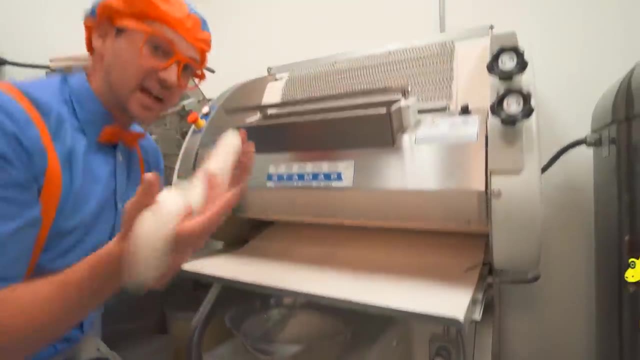 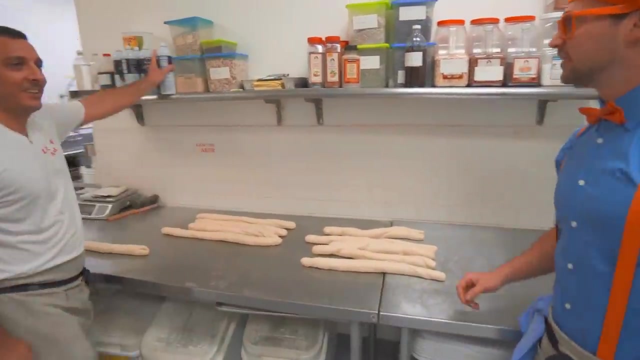 Okay, last one: Whoa, this is so much fun. It was like this size. And then it comes out kind of like a snake. Whoa, Okay, here we. are You ready? I'm ready. now what? 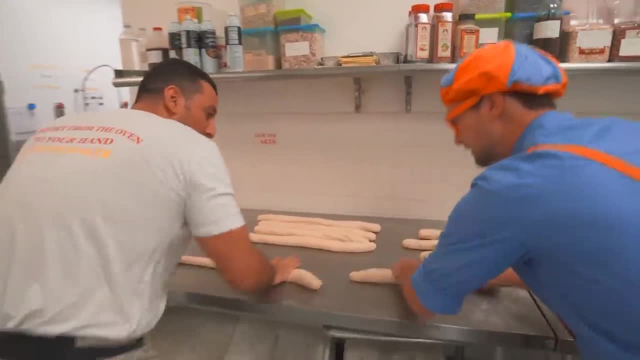 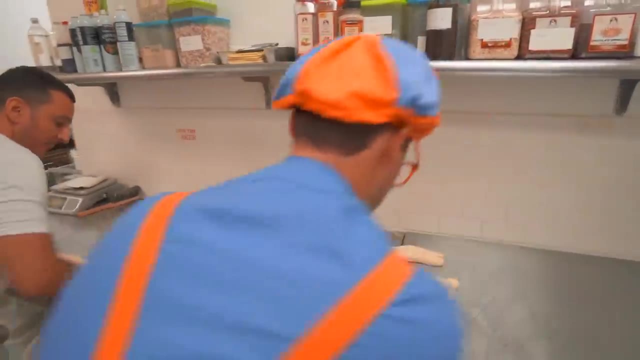 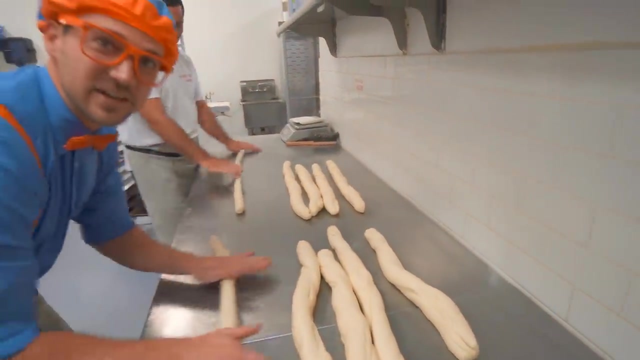 Now we're gonna roll it. We're gonna open the dough Slowly, slowly. Okay, open the dough. It feels good, right? Yeah, it feels nice and good. It's getting really long, do you see? Okay, you're a lot better than me. 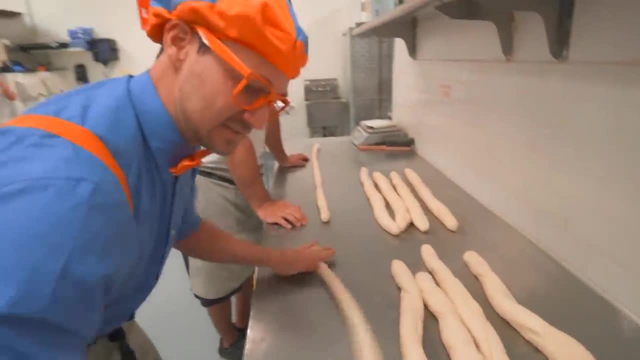 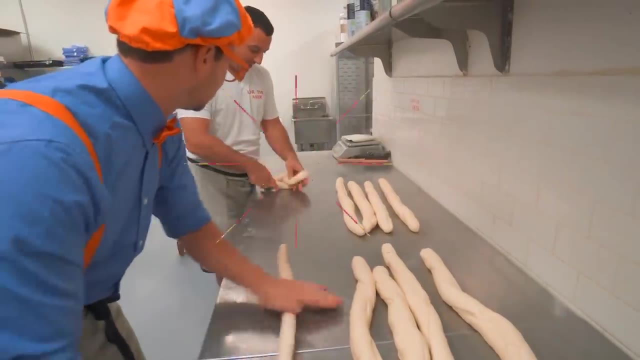 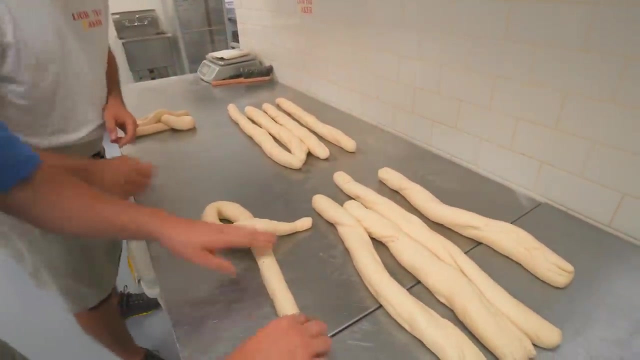 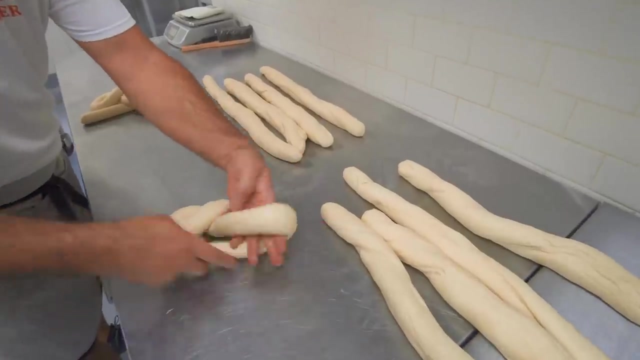 Okay, like that. Yeah, a little bit longer. Are you ready? We're gonna shape this. Okay, We're gonna do it. Eight, Okay, Okay, Now twist this one. Twist this one down underneath Number eight, right, Ooh, number eight. 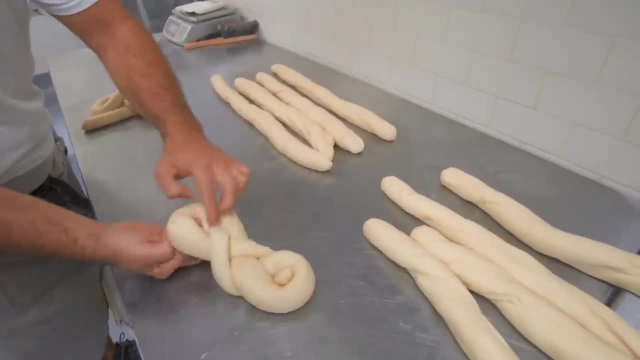 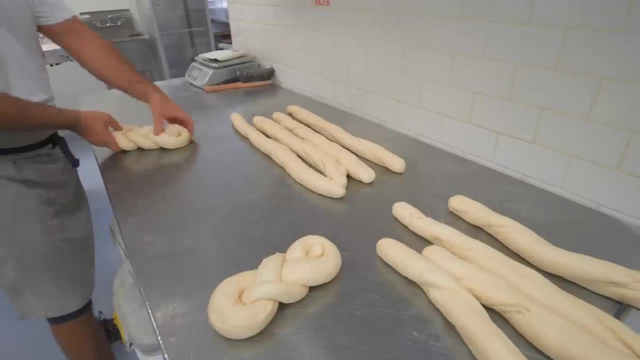 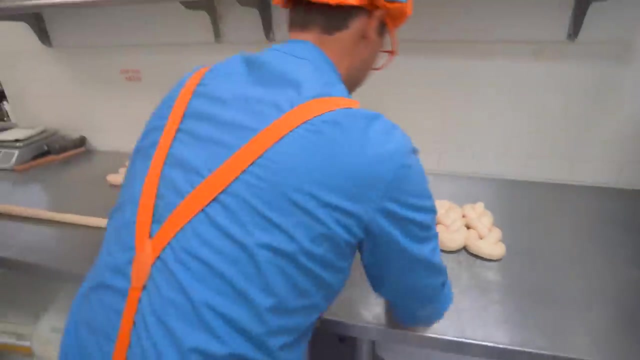 Now he say hello Blippi. and he say good night, Ooh, hello, good night. Okay, there we go. Okay, whoa, Okay, let's do another one. All right, here's another one. 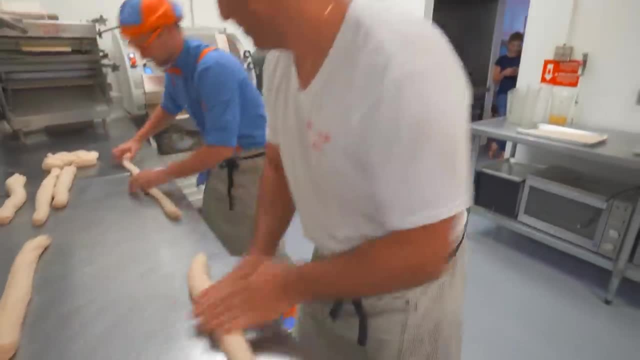 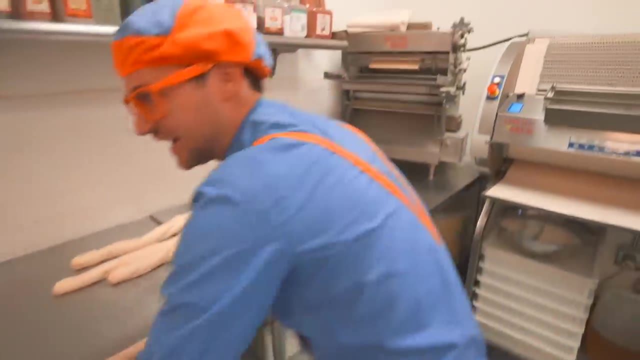 One, two, three, four. All right, we're gonna do another one. Okay, Are you ready? Are you ready? Let's get it started. One Good. Two, Three, Four, Five, Six, Seven, Eight. Nine, 10., 12., 13., 14., 15., 16., 17., 18., 19., 20., 21., 22., 23., 24., 25., 26., 27.. 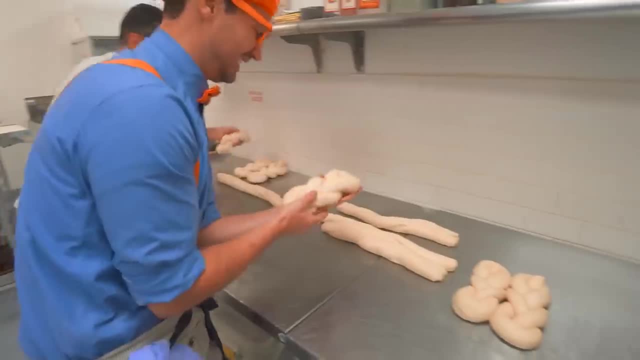 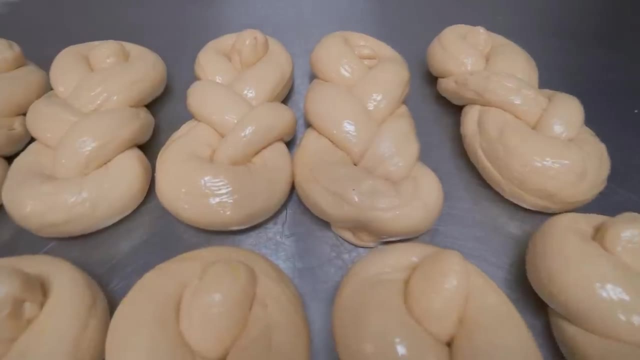 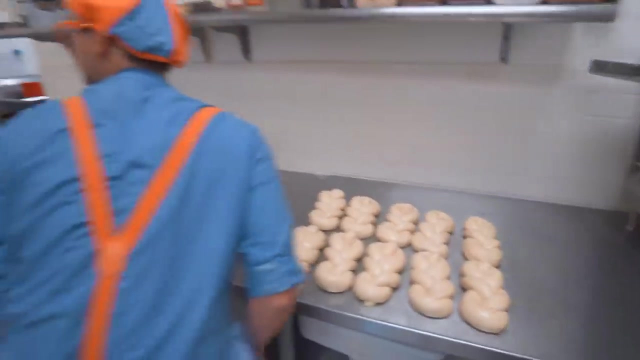 Yes, Very good. Ooh, they look so tasty. Now, what do we do? Hey, Pippi, shall we go and bring the seeds? Okay, You grab the pumpkin seeds, I'll grab the sesame seeds. Ooh, yum. 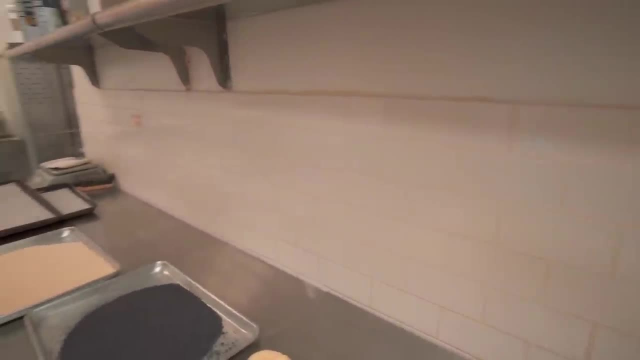 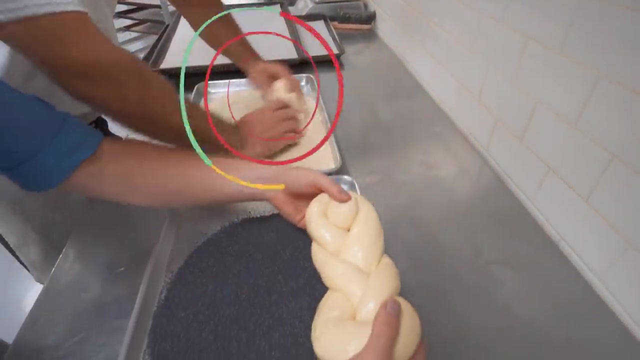 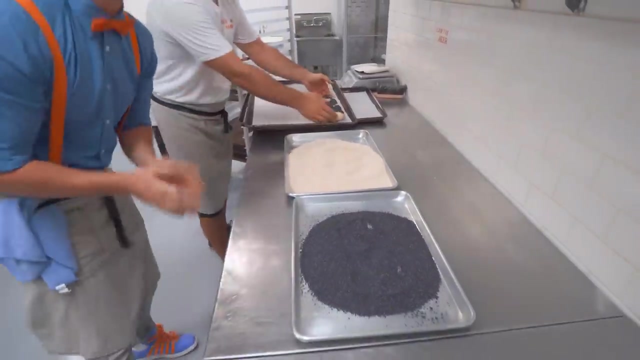 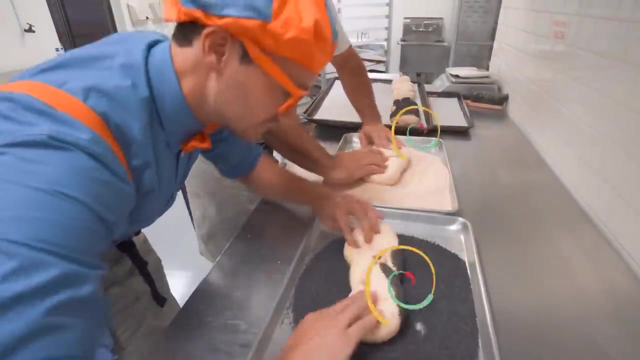 Alrighty, perfect, Good huh, Okay. so we grab one Okay Ready, We flip, We flip, Whoa, That looks good. One more Okay. one more Okay. One, two, three Ready. 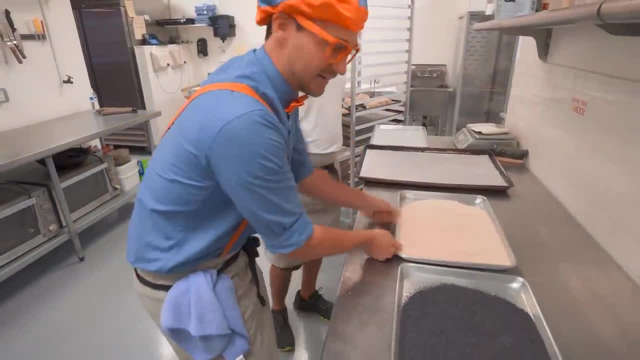 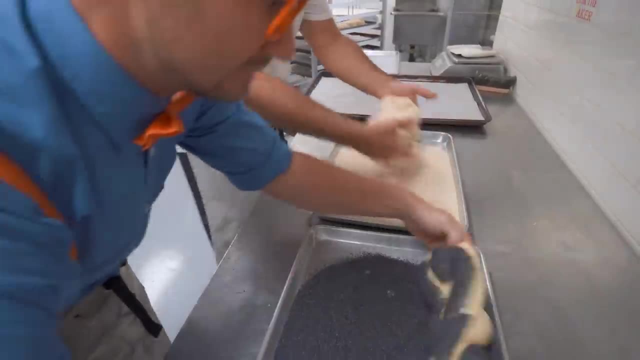 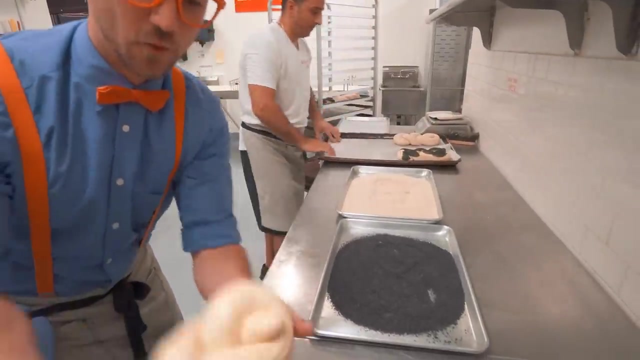 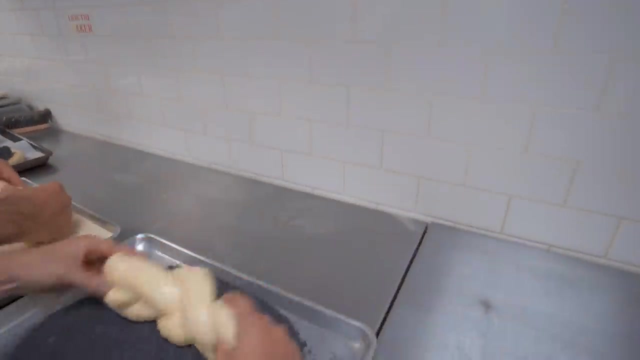 That looks yummy. Okay, let's do a couple more. Okay, It's yum. Ooh, this is fun. You get to roll these in the seeds. Okay, Alright, I'm ready Ready. One, two, three. 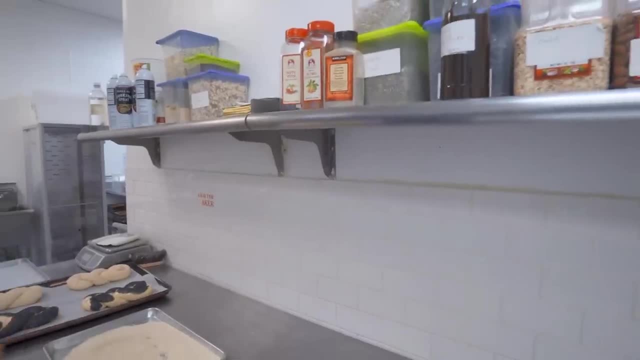 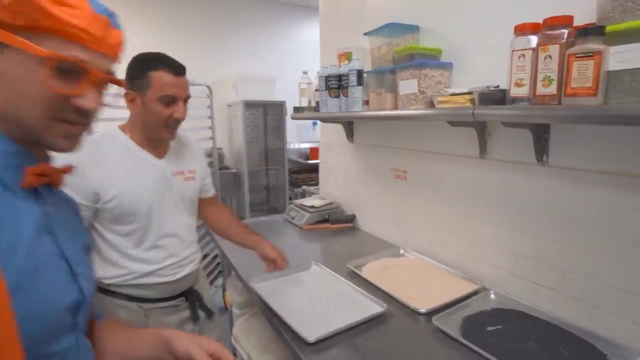 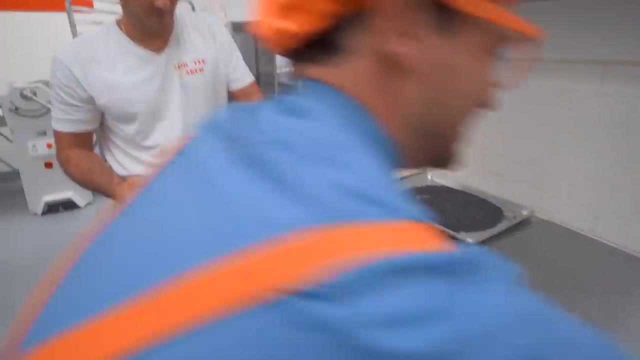 Oppa, Oppa, There we go. Oh, Oh, Okay, Can we leave the last two plain? Exactly, Okay, Alright, There's one And here's two. Perfect Okay, now Put this in the proofer. 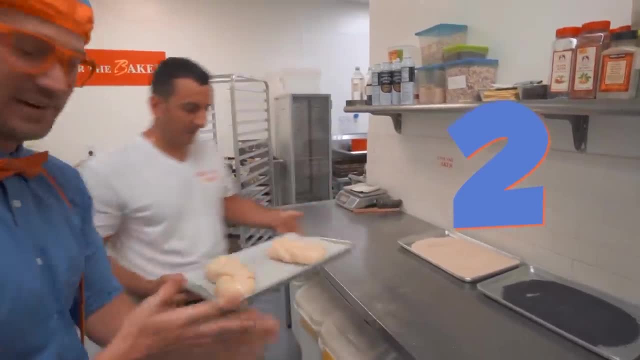 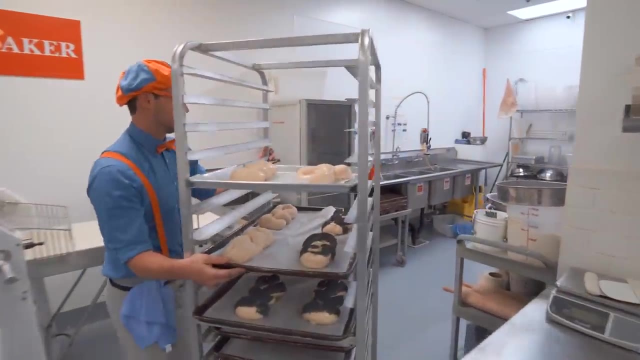 The proofer. Okay the proofer. Yep, Let's go. This is the proofer. It's pretty humid in there And it lets the dough rise. Oh, Oh, Oh, Oh, Oh, Oh. 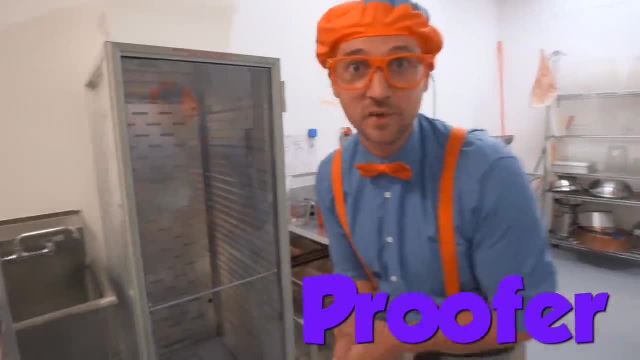 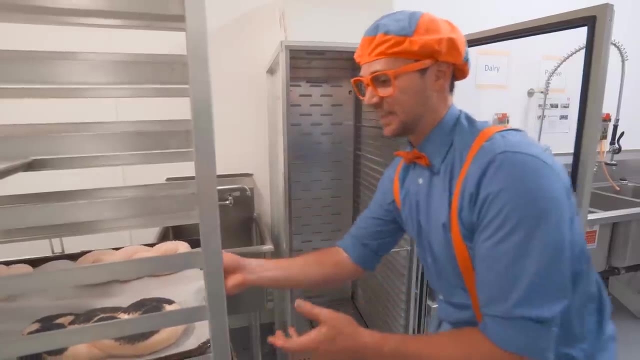 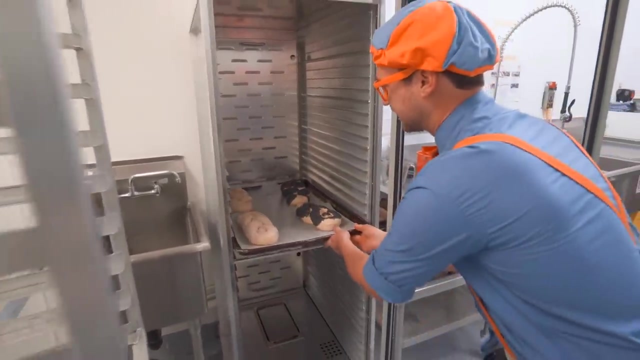 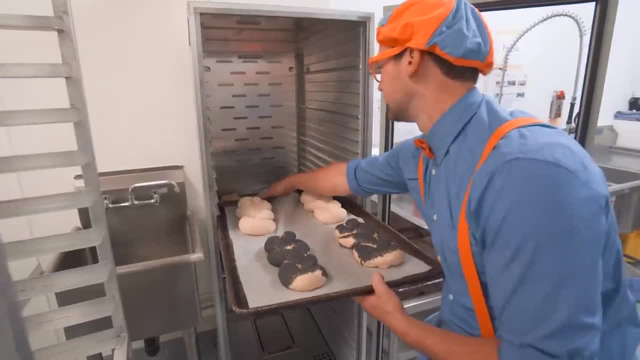 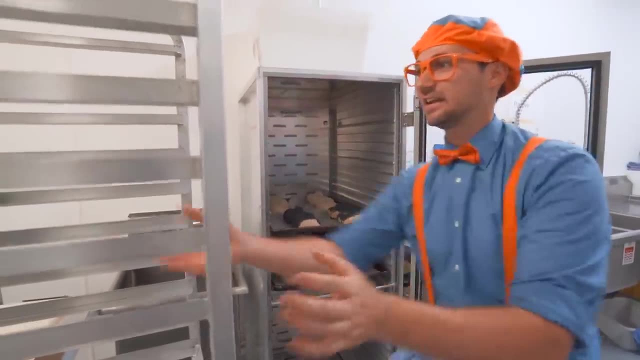 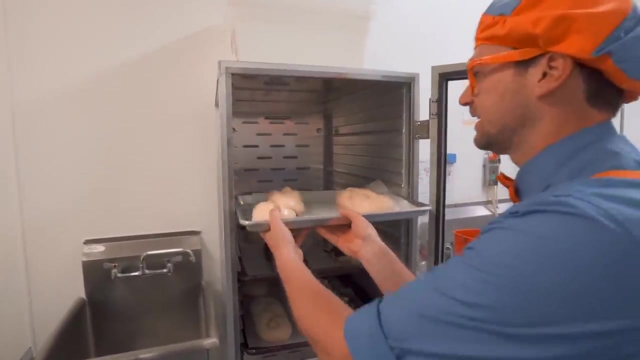 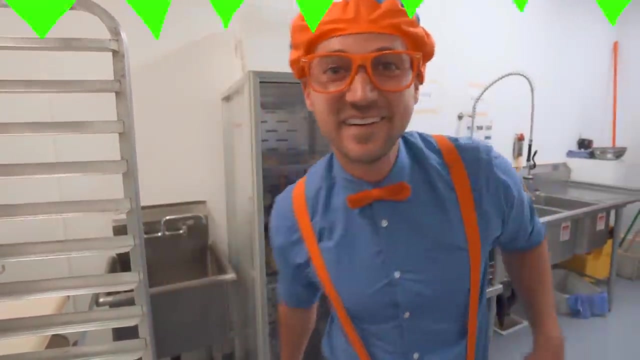 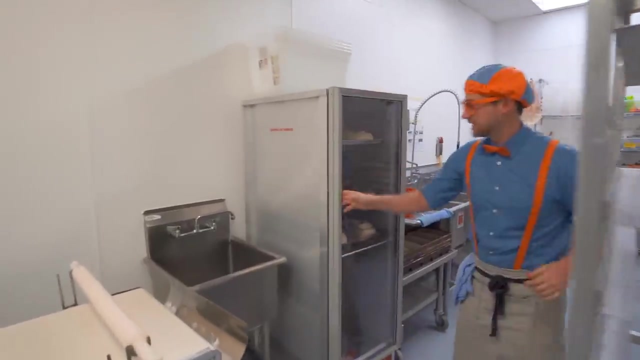 No, Nobody's talking. Uh, Ah, Okay, you're right. Okay, Woah, two plain ones let's put right here and then we get a wait. good job, okay, now we need to get the holla out of this thing. okay, remember whoa, the plain ones, and. 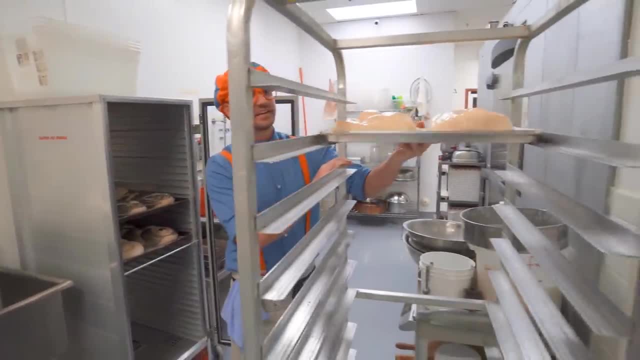 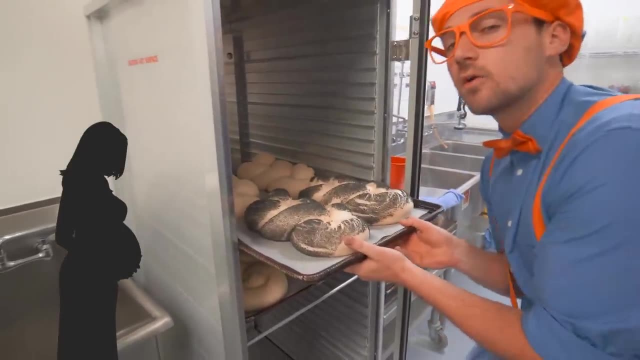 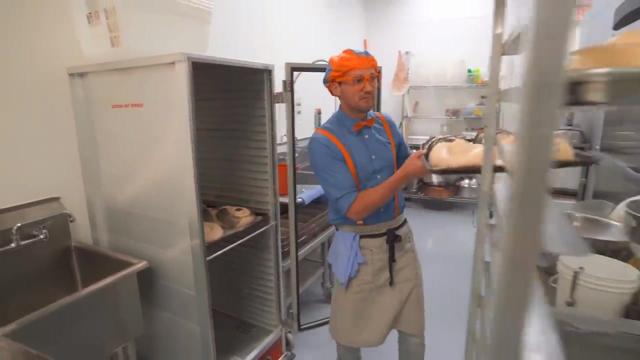 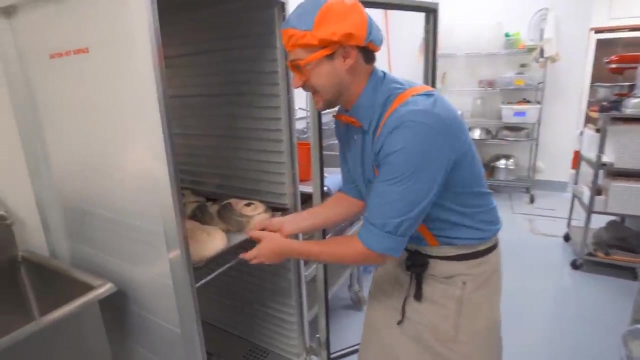 they're bigger. they're bigger than before. yeah, perfect. this is kind of like the mama's womb: they grow really slowly. it's nice and warm. wow, they're way bigger than before, but don't worry, when we cook them they're gonna get even bigger and then they're gonna be nice and golden color. 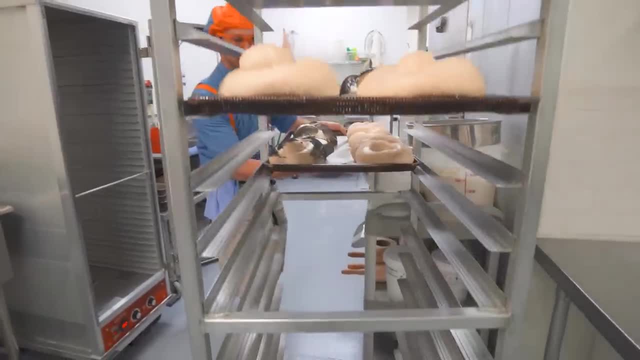 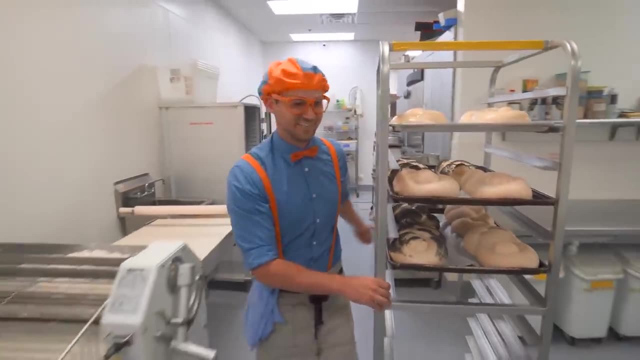 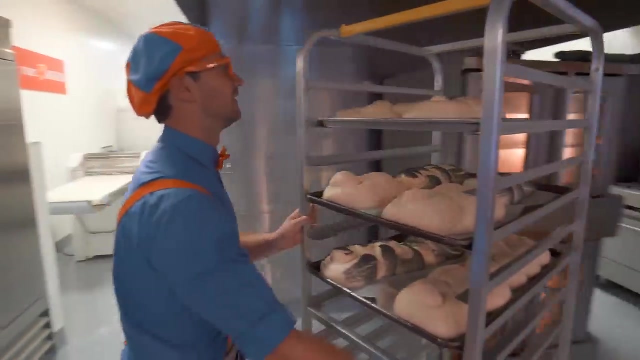 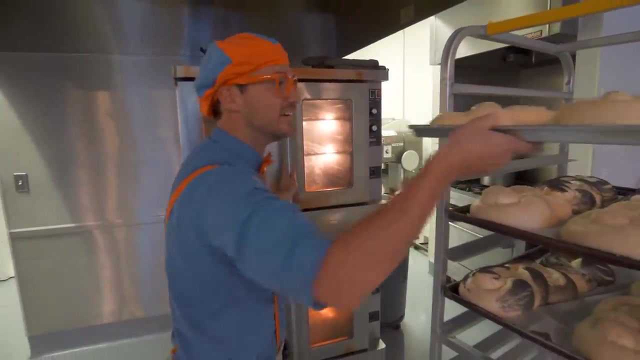 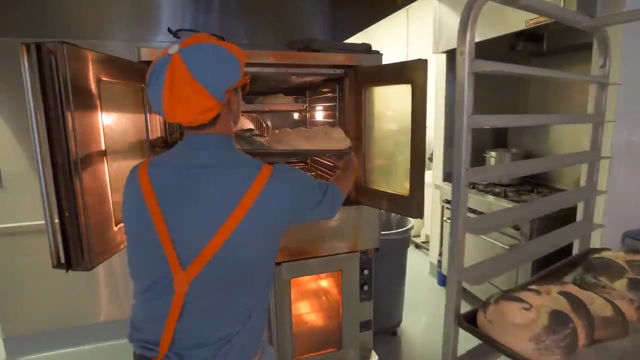 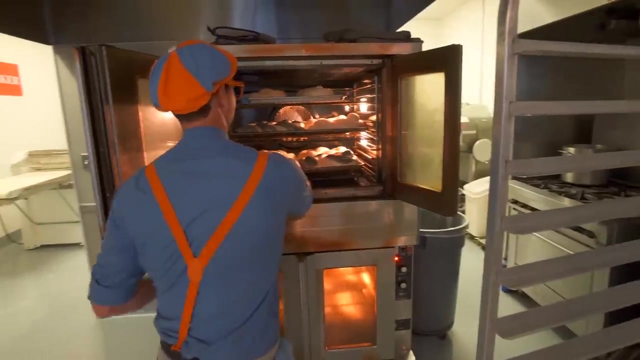 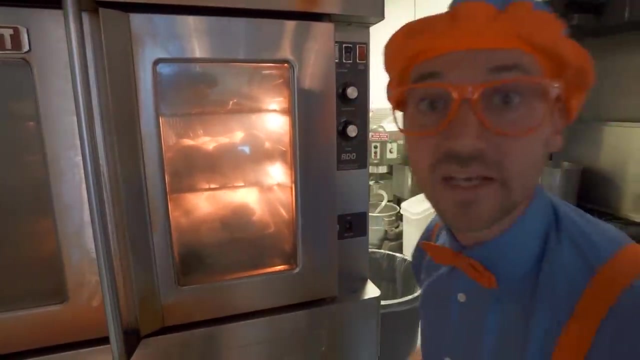 okay, last one. all right, do those look tasty, or do those look tasty? okay, all right, let's bring them to the oven. okay, here we go, all righty, hey, let's open up the oven and put them in ready. one tray, two trays, three trays- okay, now we need to wait for 20 minutes. now, we just wait. 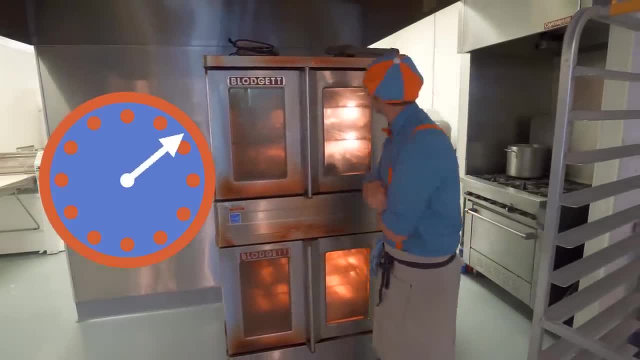 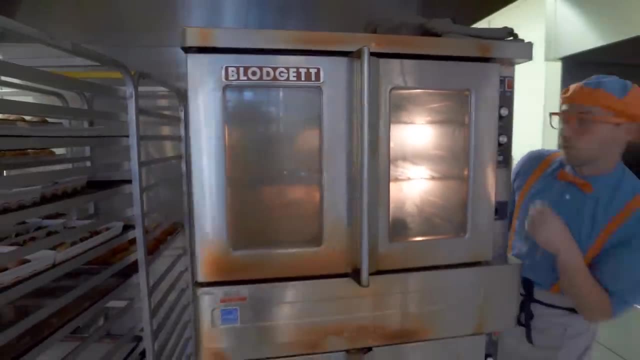 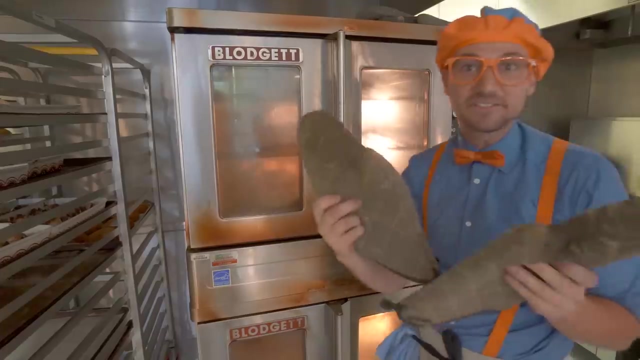 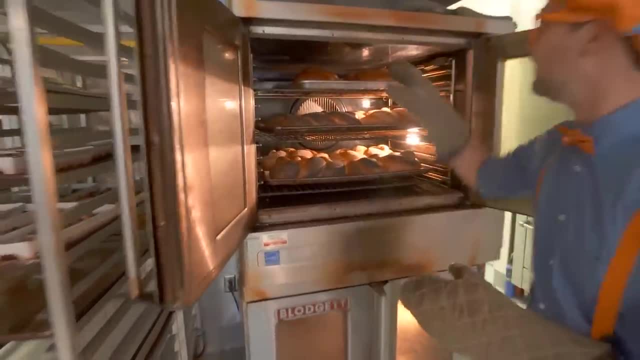 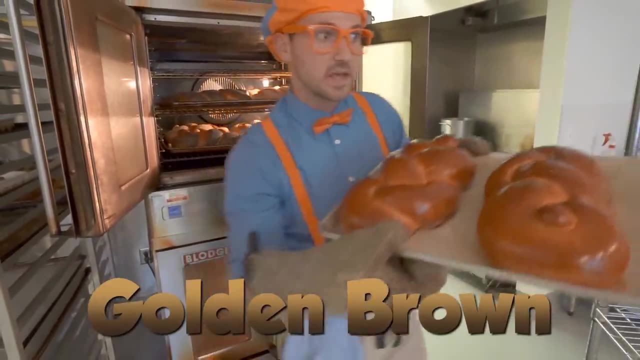 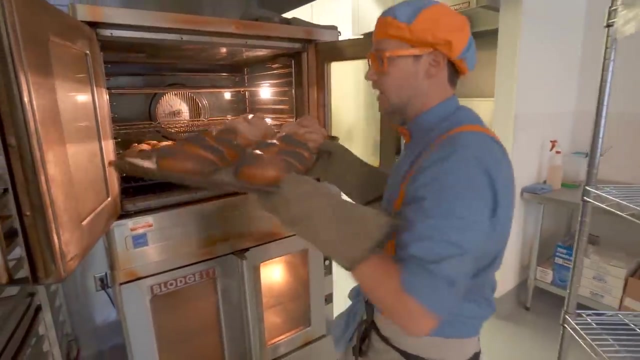 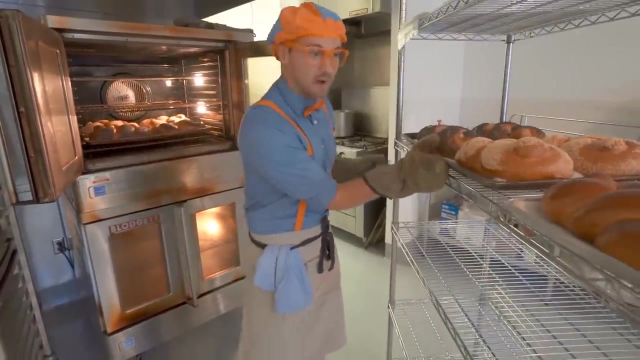 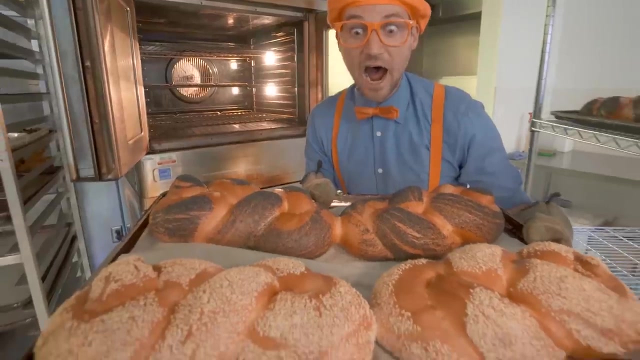 whoa, let's take them out. WHOA big they are and they're golden brown. that looks so good. good job, okay. grab this tray. whoa, these are colorful. whoa, remember making these. very good job, okay. and the last one. okay, let's put that right there. let's close this up. let's take off the. 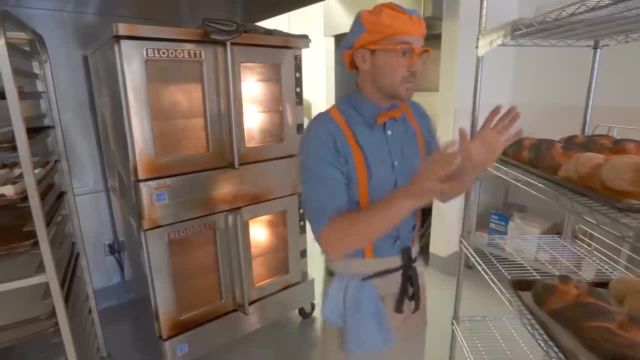 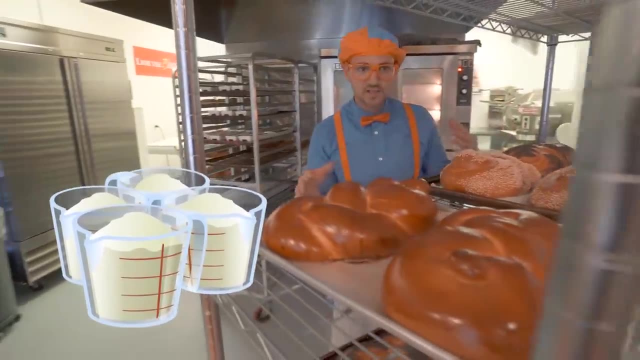 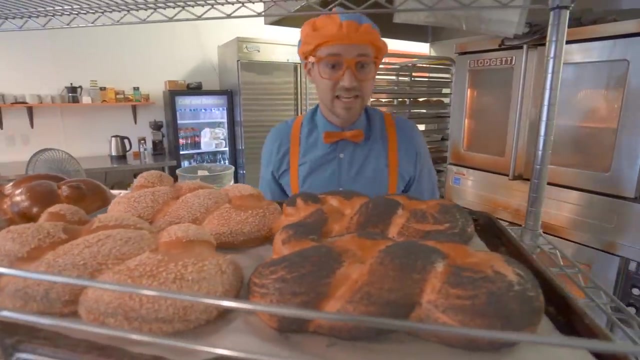 mitts. Wow, wasn't that cool creating these from scratch. yeah, it used to be flour and some other dry products, and then we added some liquid. and now, with all these other things, it grew into some tasty baked bread. and now, with all these other things, it grew into some tasty baked. 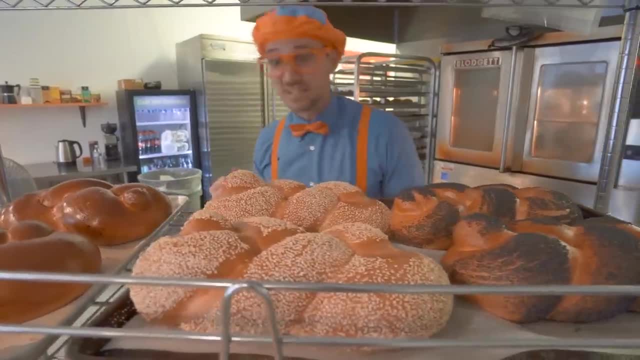 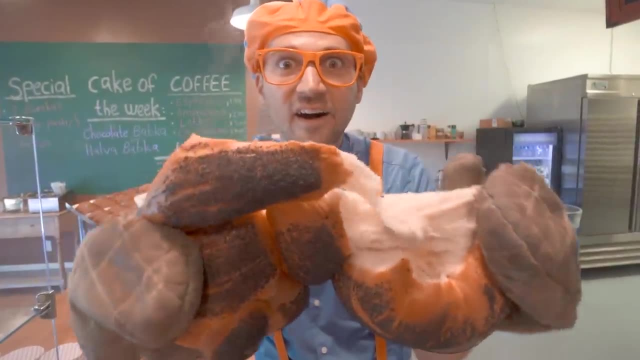 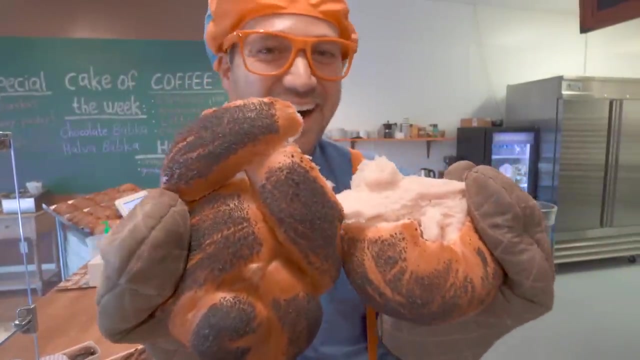 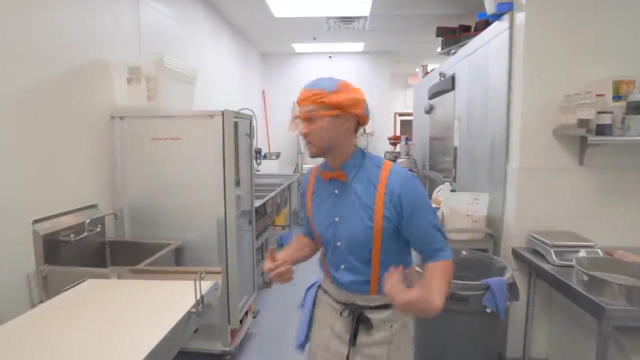 bread, and now, with all these other things, it grew into some tasty baked goods. I'm so excited to eat these. did you hear that the boss said we need to bring him the croissant? come on, okay, let's open it up. okay, let's take one of these out. 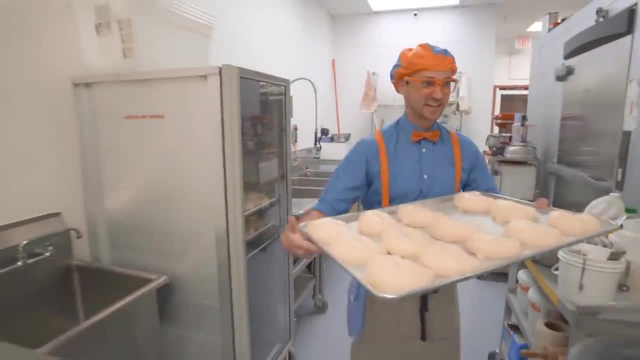 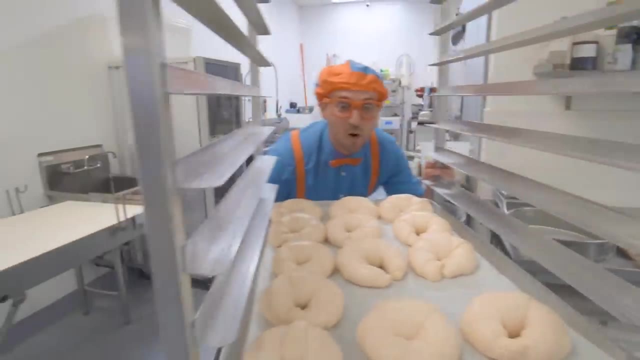 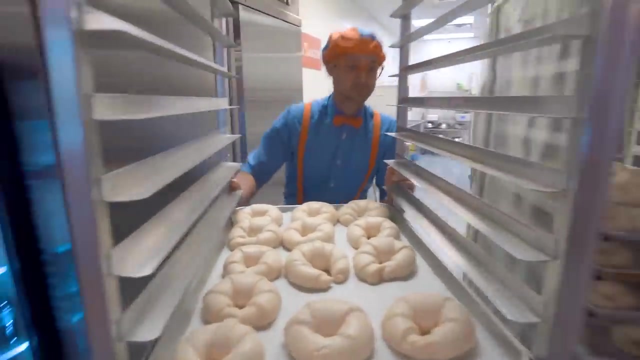 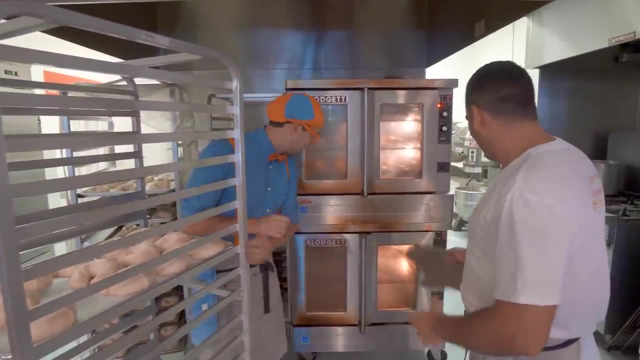 whoa, those look tasty. okay, then we put it right on the tray right here. whoa, check it out. whoa, okay, okay, let's go bring them the croissants. okay, all right, here you go, here's the croissant. oh, thank you, Blippi, you're welcome. now what do we do? put this in the oven in 15 minutes, okay, so. 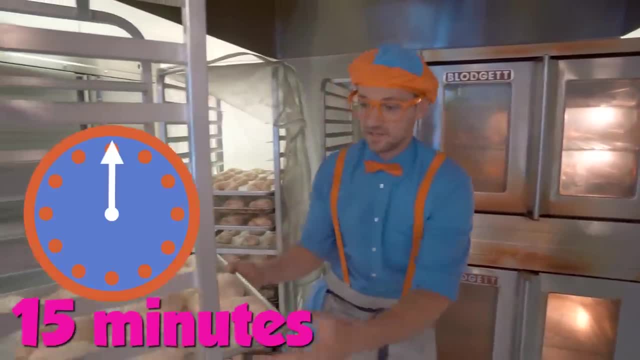 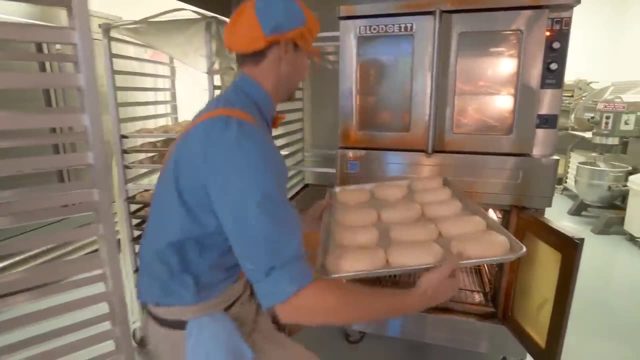 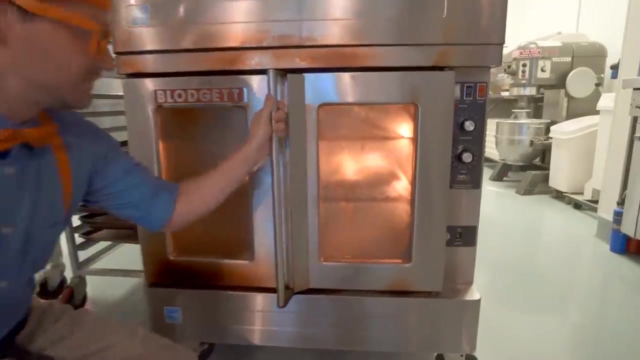 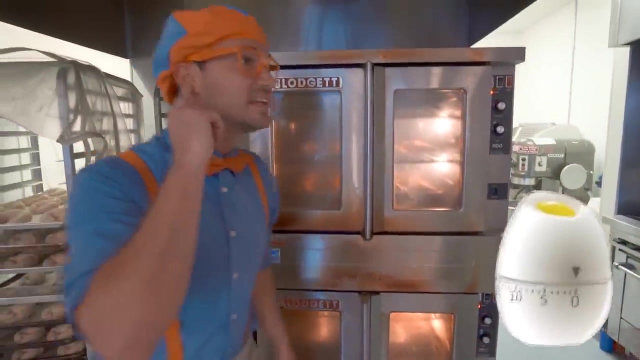 now we need to put these in the oven for 15 minutes. okay, let's open it up. whoa, it's so hot in there. okay, here we go. perfect. good, okay, close it up, okay, okay, do you hear that? what does that mean? the croissant is ready. okay, so take this out, okay. 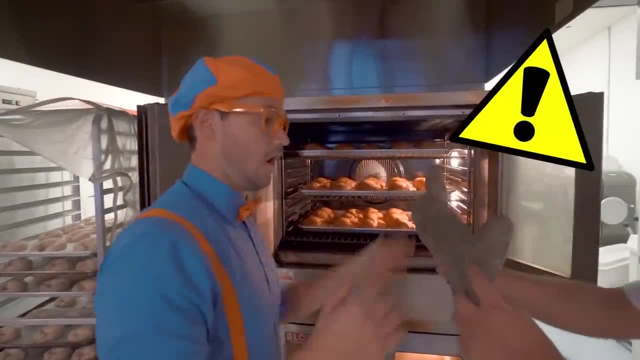 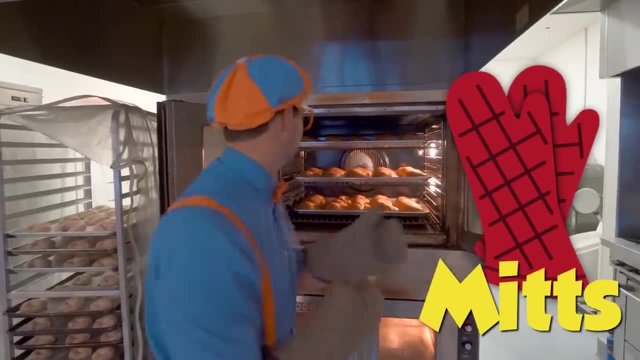 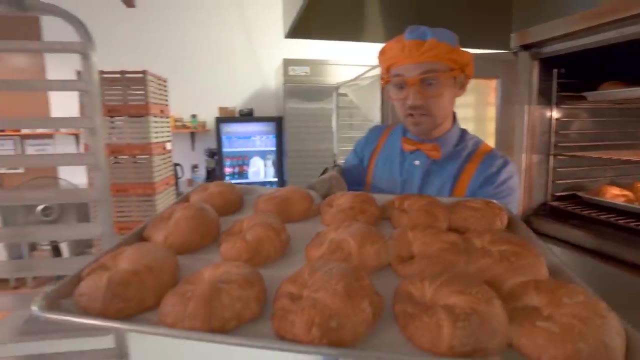 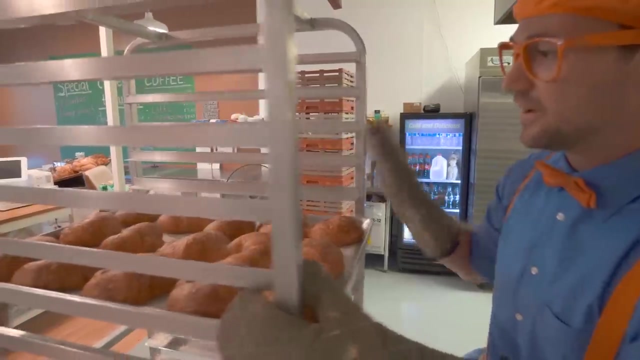 okay, let's take out the hot croissants. hey, Blippi, safety first, oh, safety first. these are mitts, and they keep your hands really warm. okay, this one looks really good. check it out. whoa, that looks so tasty. okay, let's put it right on the rack. okay, now we can pick one. let's spin it around. 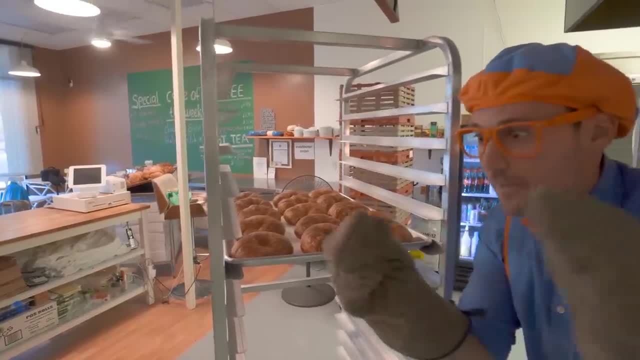 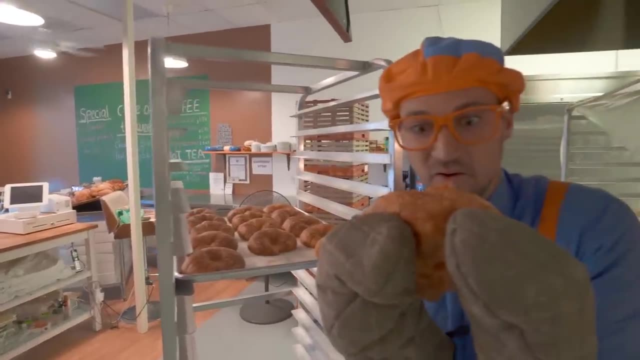 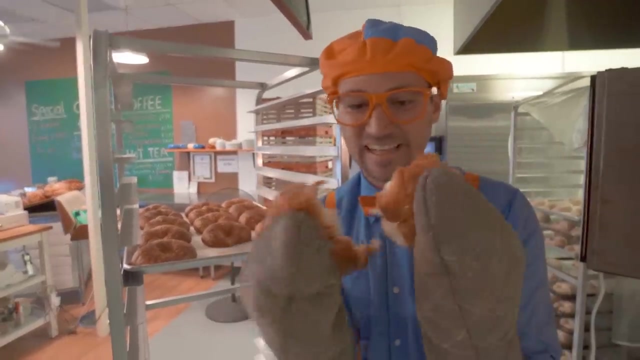 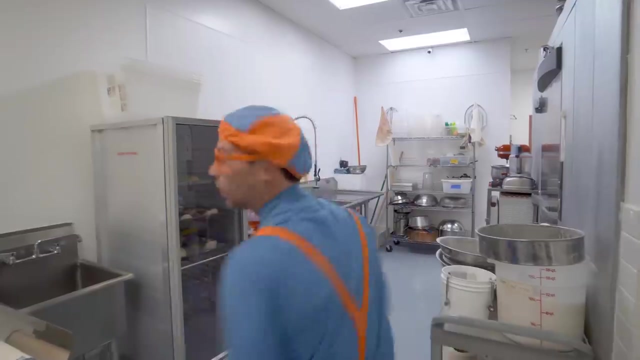 check it out. now. we can pick one up, rip it open and see if it's cooked. I'm using the gloves because it's really hot. oh, it smells so good and it's so flaky and soft at the same time. yum. now that everything is baking and also other things are rising, let's see what else is in a bakery. 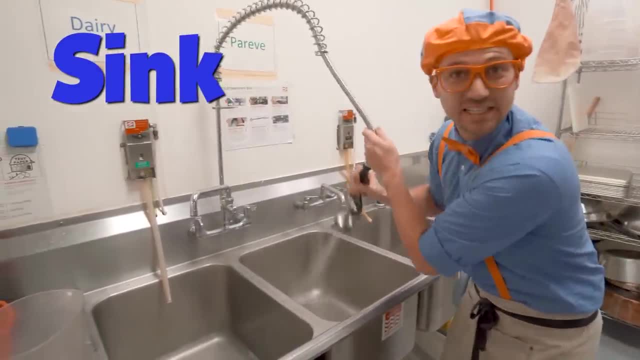 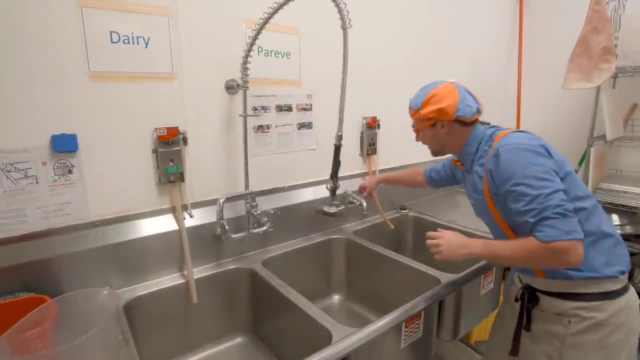 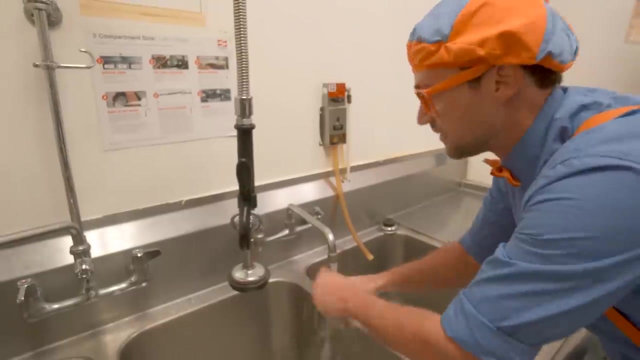 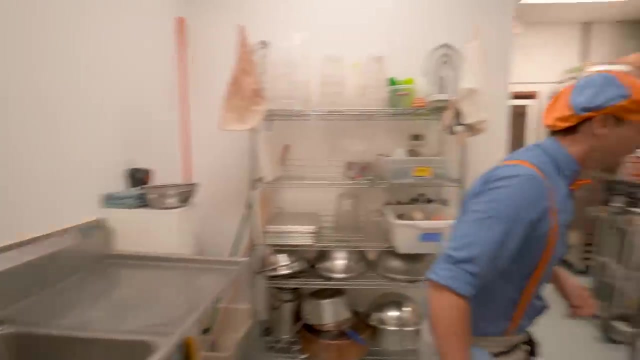 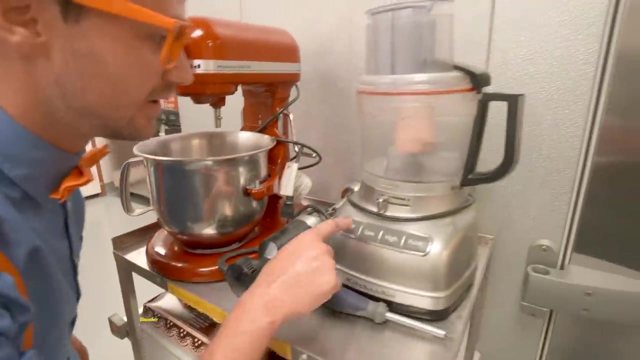 yeah, check it out- a place where you can even wash your hands. yep, washing your hands is really important when you're dealing with food. okay, let's turn that off. okay, whoa, check it out like a miniature mixing bowl. whoa, Whoa, and it kind of looks like a blender. 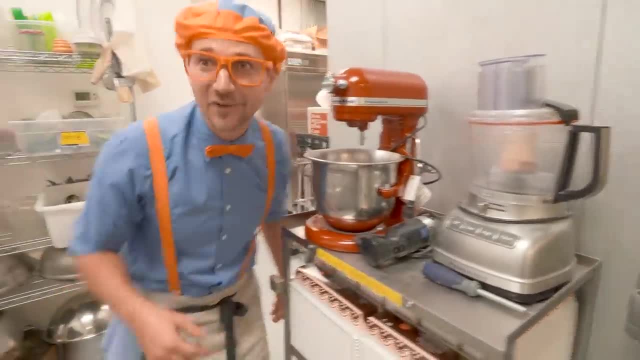 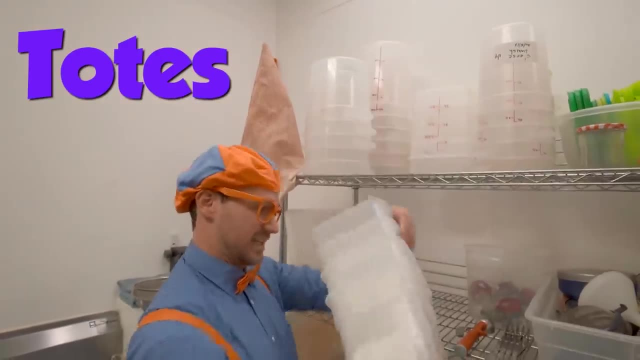 Whoa, but? or a food processor, I don't know. it's cool, though. Whoa, look at all of these things. Whoa, a bunch of totes and containers. Let's count them. Okay, we have one container. 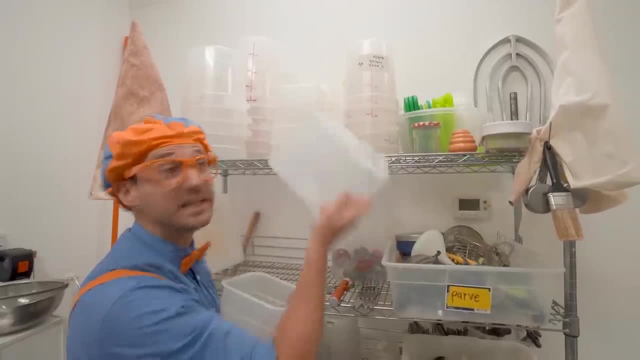 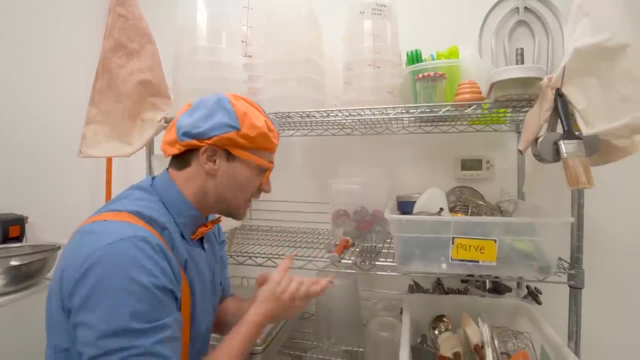 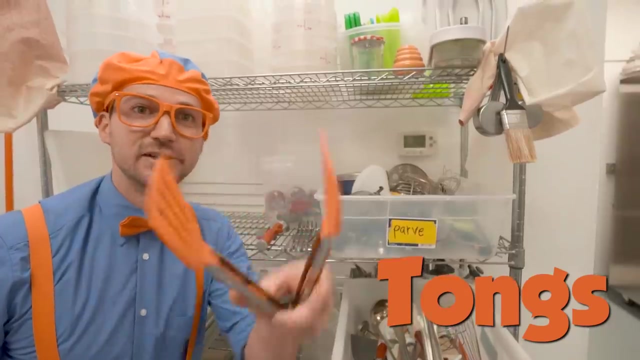 two containers, three, four and four containers in that stash. Ooh, whoa a spatula, some tongs that kind of look like spatulas. Ew ew, ew, ew ew ew Whoa. 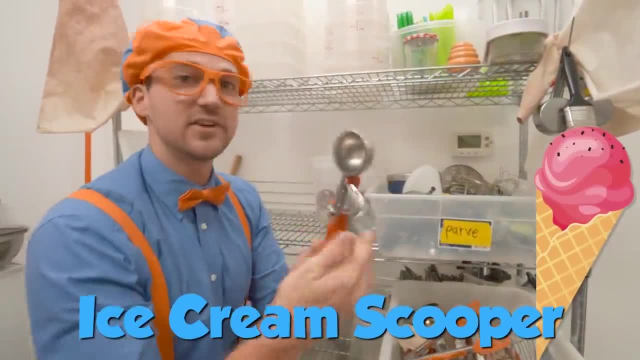 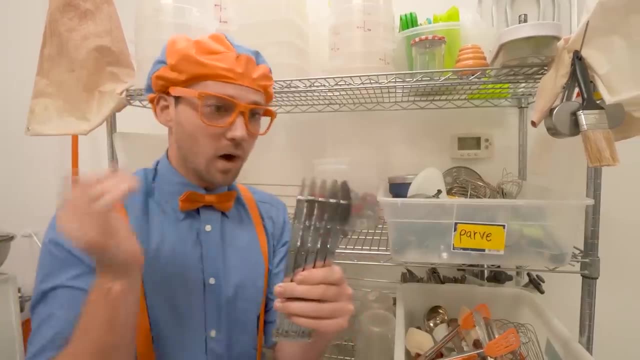 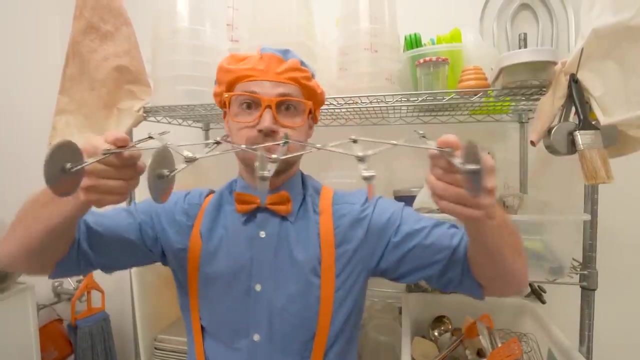 Whoa, a little ice cream scooper. I bet you can scoop and measure a bunch of cool things with this Whoa. look at this Whoa, that's sharp. Whoa, Whoa. you can make some nice even lines with that. 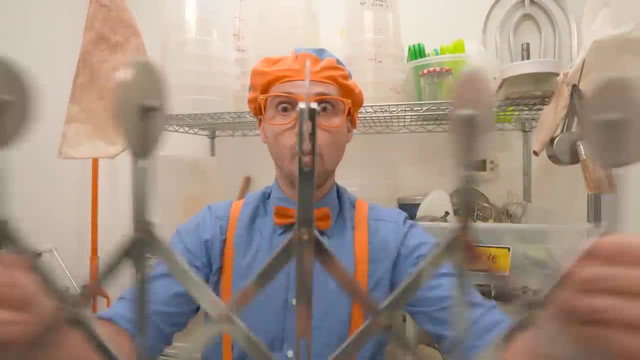 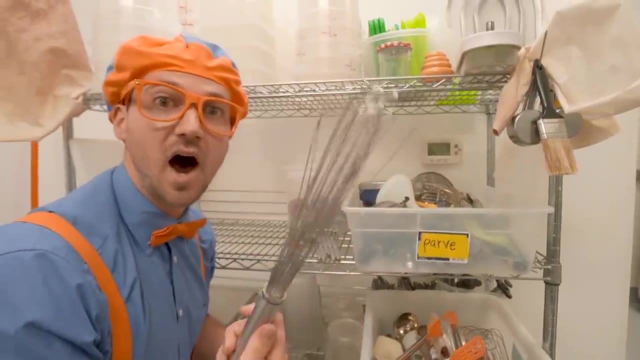 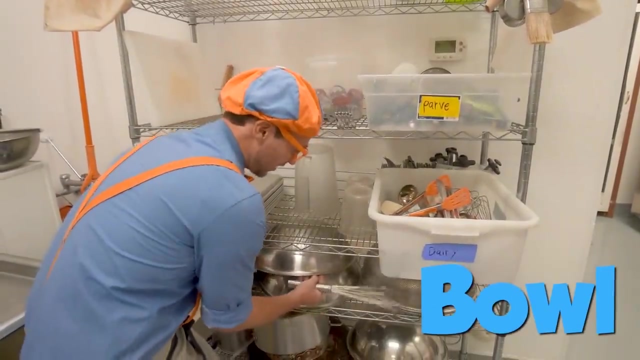 Ooh, and you cut a bunch of dough. Whoa, whoa, whoa, whoa. Okay, let's put that back. Ooh, a whisk, No way, Oh, and a giant bowl. Check this out. 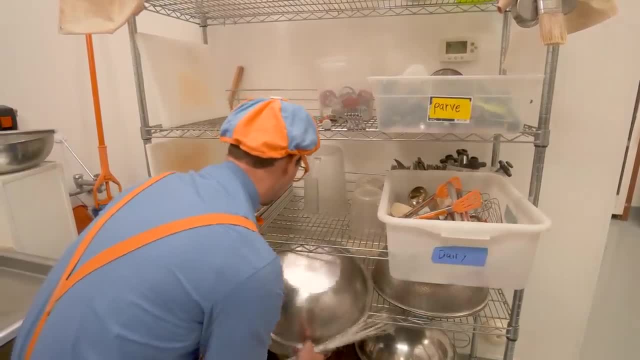 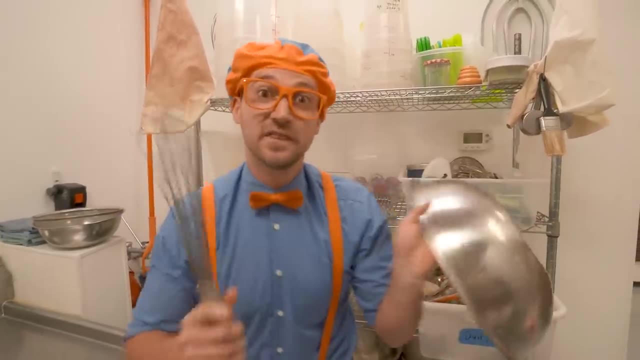 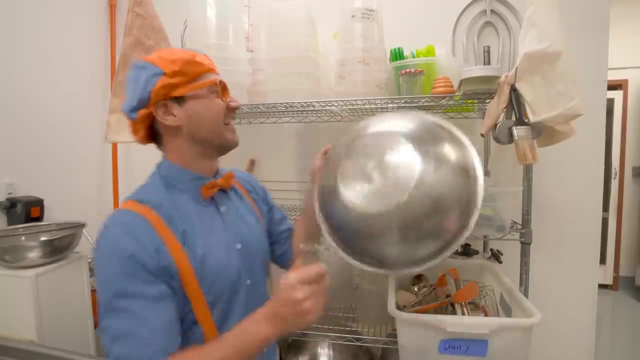 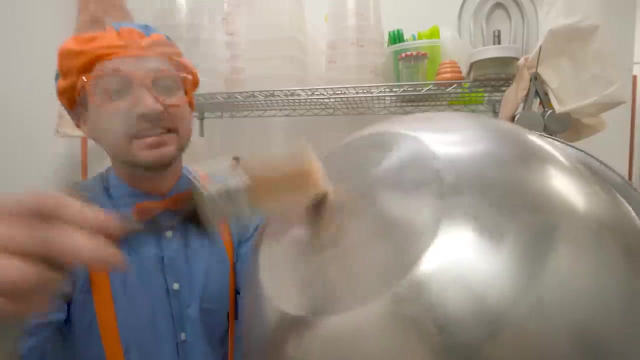 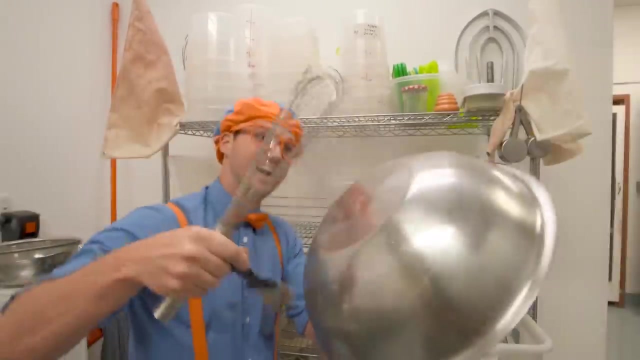 I have something fun to show you. This is called the baker's drum. Yeah, the baker's drum. Ooh, listen to this. I love making music with things that I find like around your house, around your house and around your house. 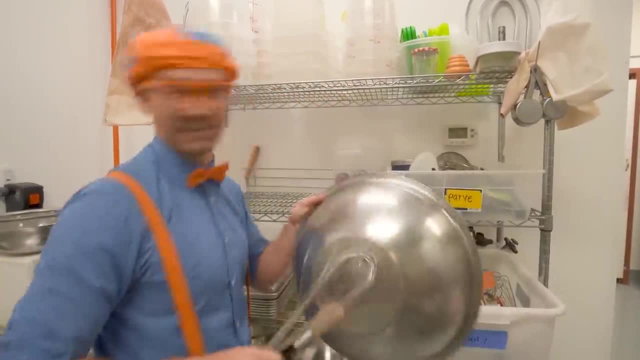 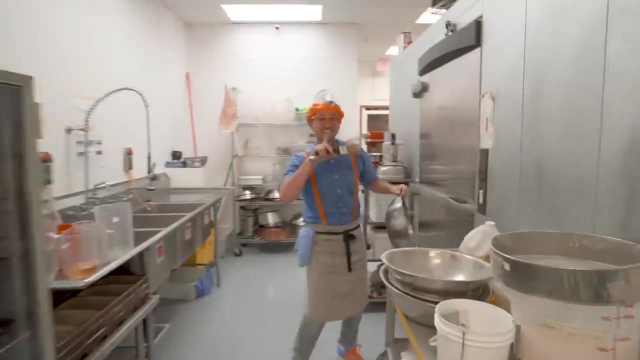 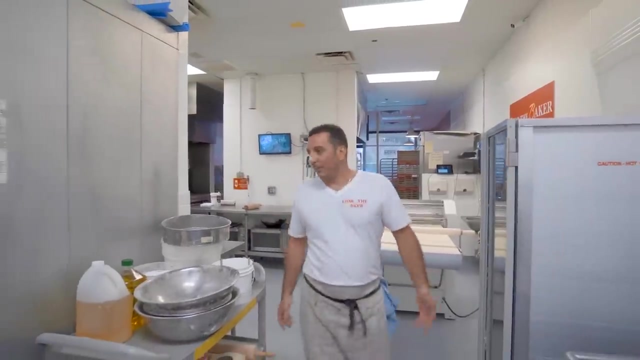 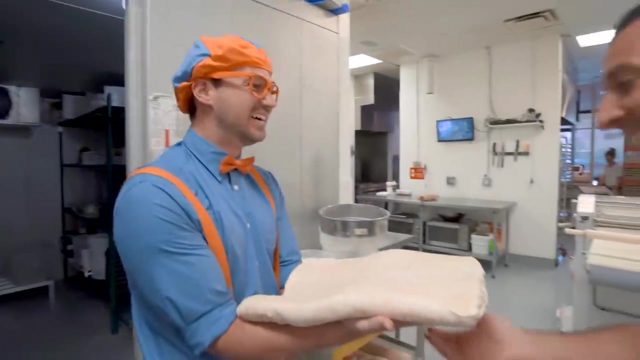 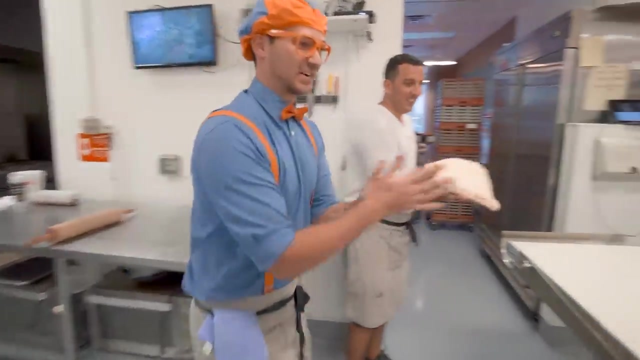 I love making music with things that I find like around your house, around your house Or even at the bakery. Here you go. what do I do? Come okay, Okay. Okay, here's the dough. Okay, I'm gonna throw some flour right here first. 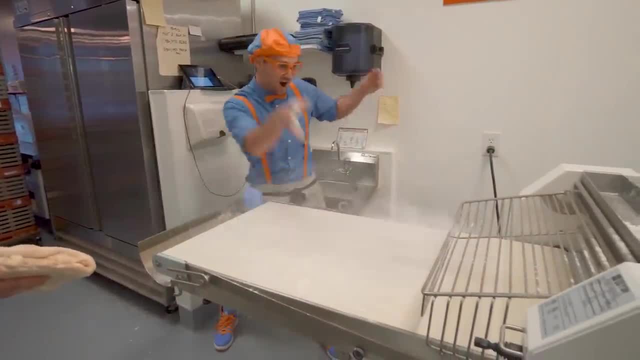 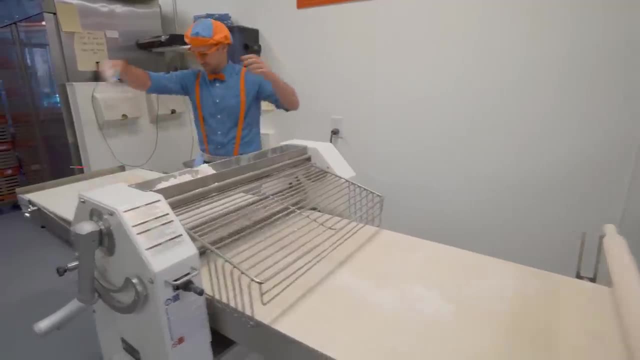 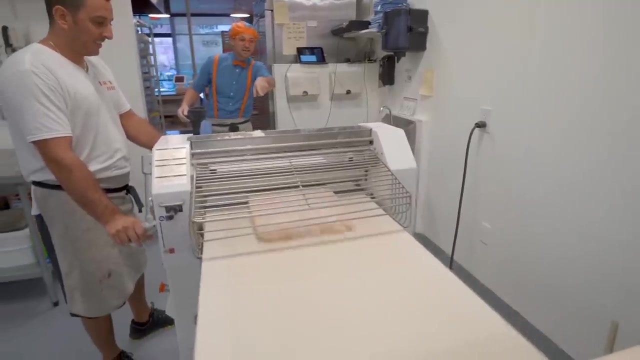 Alright, here we go. Is that enough? Okay, put a little bit more here. Where You ready to rock and roll, Yep, ready to rock and roll? Whoa, look at it. go through that thing. It's flattening out Really. 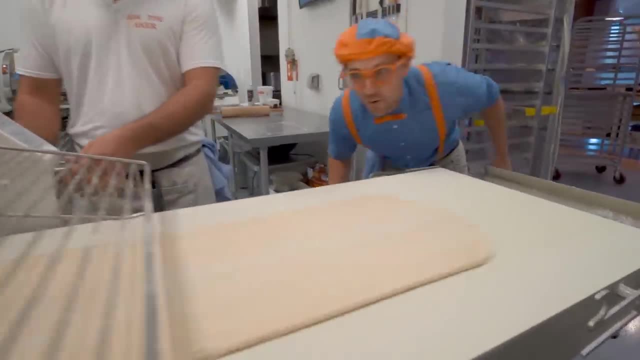 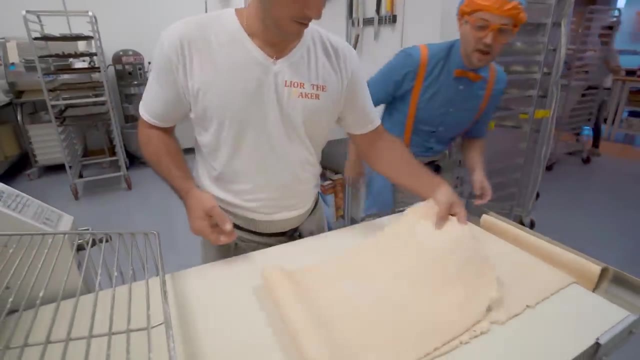 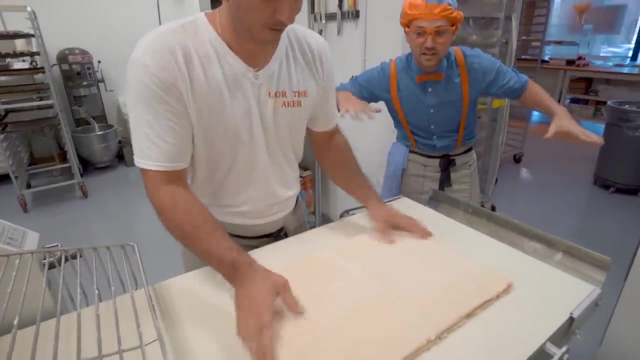 Really smooth. Look at how big it's getting. Whoa, Look at how big it got, Because it used to be really tall, But now it's really small. But then it got really long And he's folding it On top of each other And it goes back through. 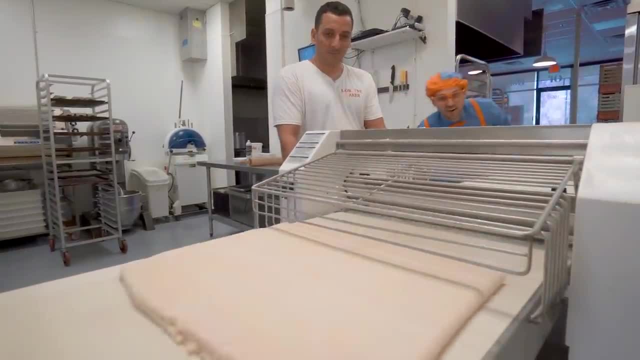 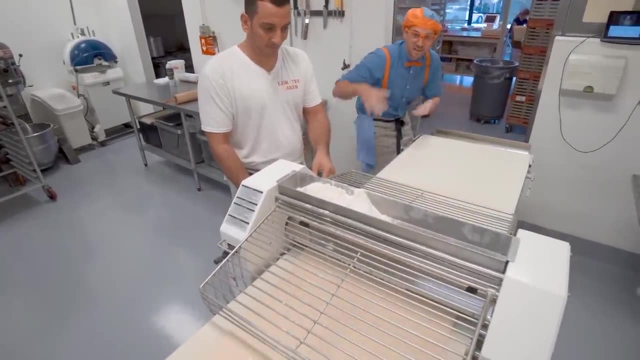 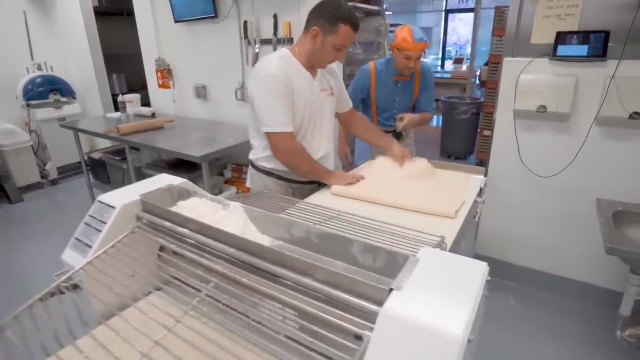 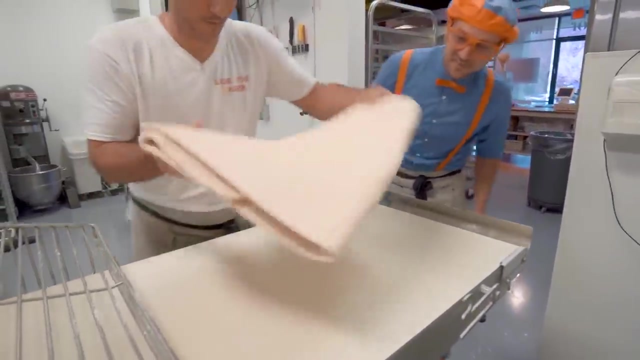 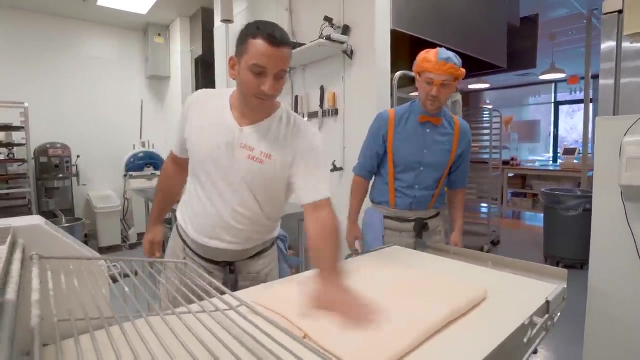 Whoa, Whoa, Whoa. It's getting bigger Because it keeps getting squished down. Because it keeps getting squished down, Whoa, Okay, another time to fold. Whoa, Whoa, That looks so cool. Huh, okay, A little bit more flour. Good job. 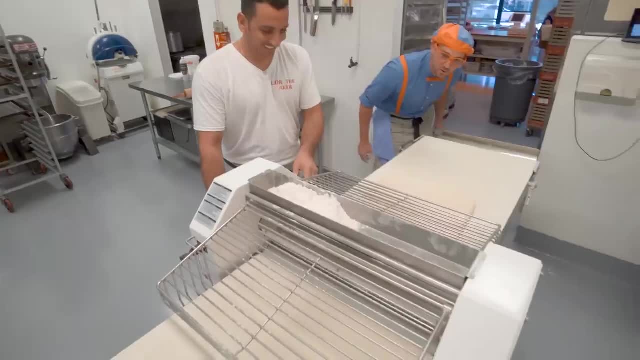 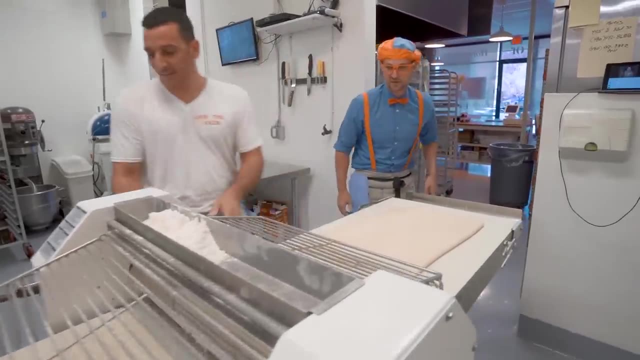 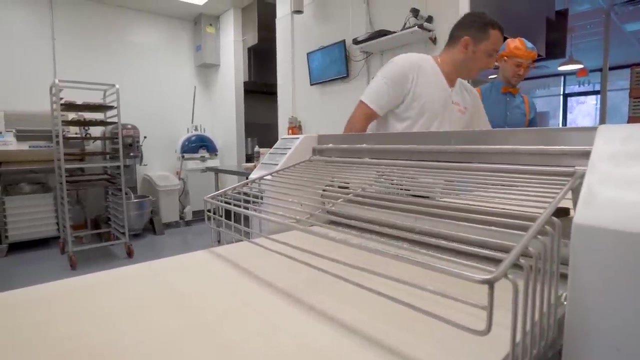 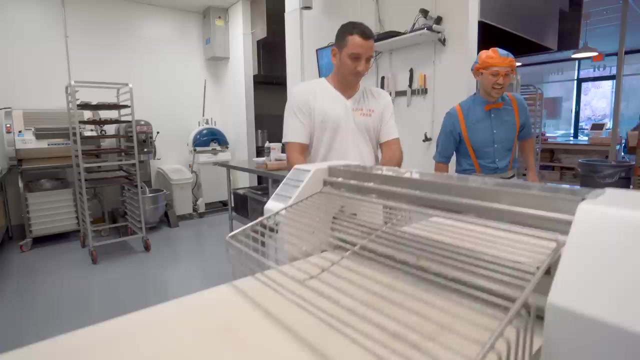 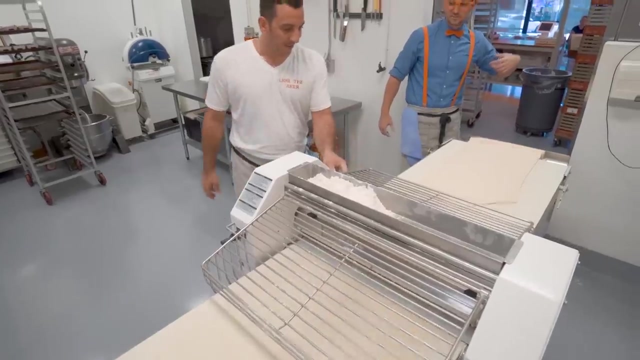 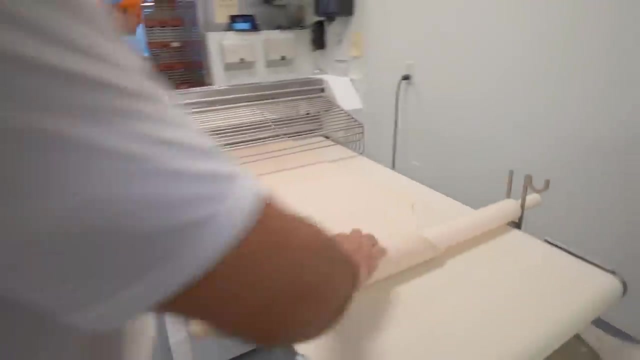 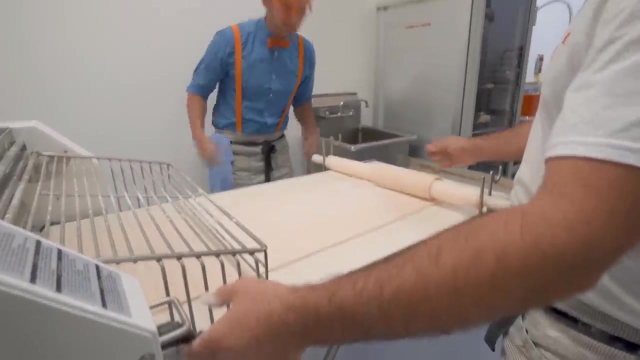 Thank you, Thank you, Thank you, Okay, Okay, Perfect, Perfect, Perfect, Perfect, Perfect, Whoa, Whoa, Whoa, Whoa, Whoa, Ready, You want to help me? Blippi, Yep. Okay, Check this part out. One, two, three, Check this out. 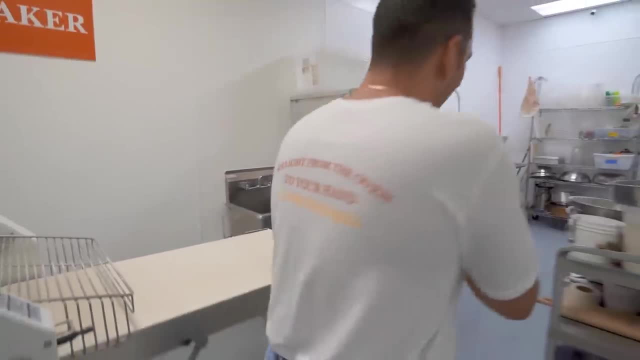 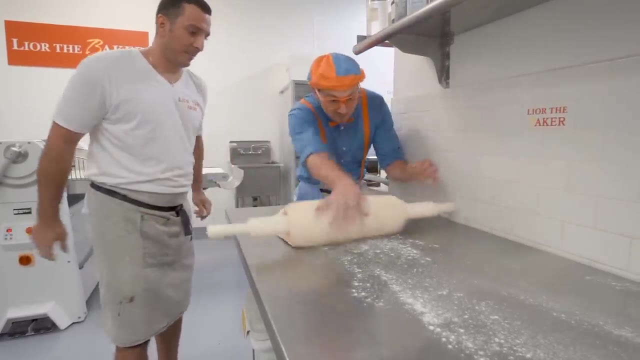 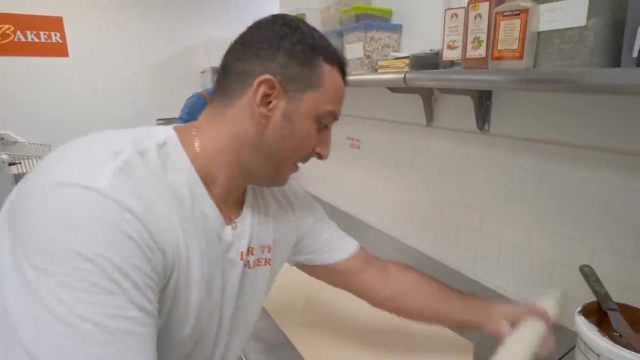 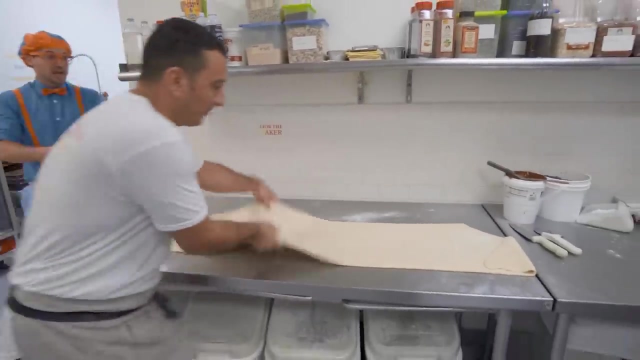 Look at it. Okay, Alright, Here you go. Whoa, Wee, Whoa. Look at how long it got. Whoa, Remember it used to be about this big, But now it's that big. That is a really long piece of dough. 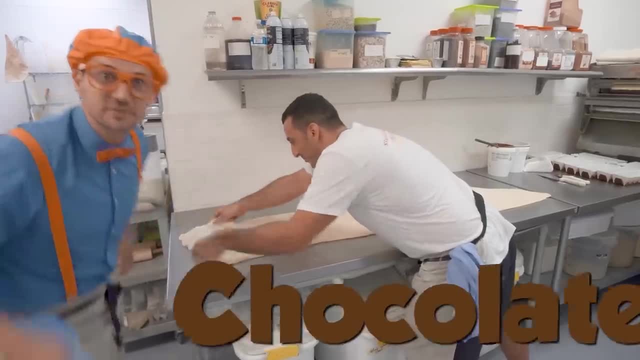 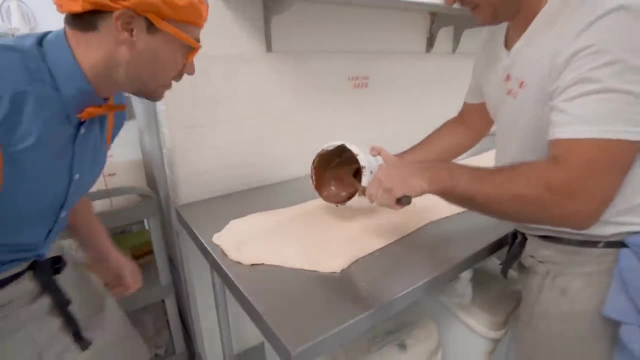 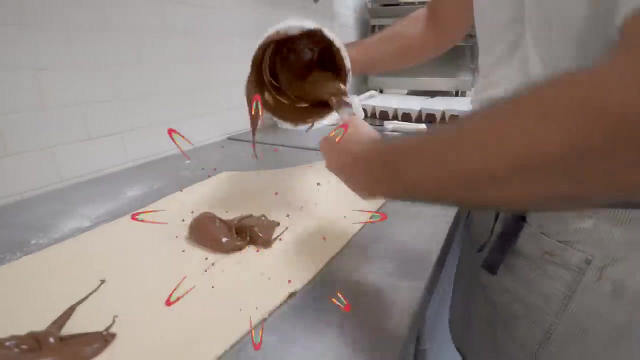 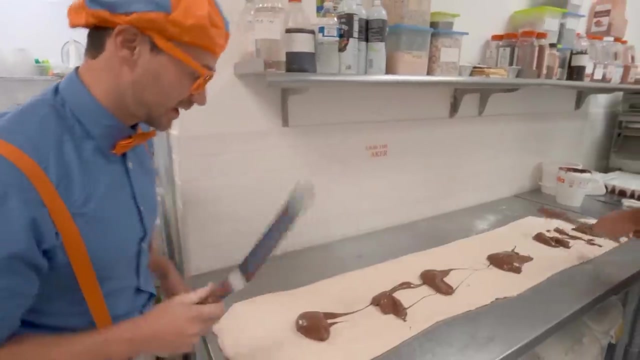 Blippi, you love chocolate, Yeah, I love chocolate. Do you love chocolate? Yum, Okay, Yum, Wow, Check it out. Ooh, That looks tasty. Blippi's crazy. Ooh, Okay, Let's spread it around. 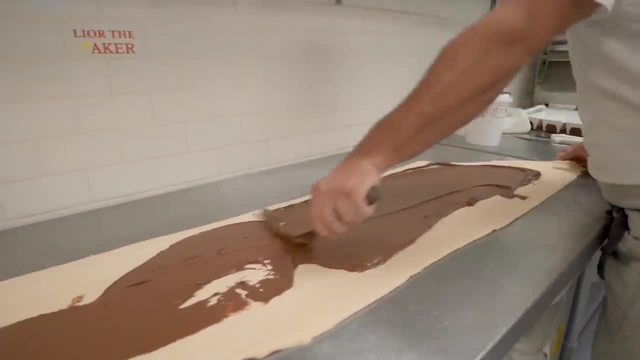 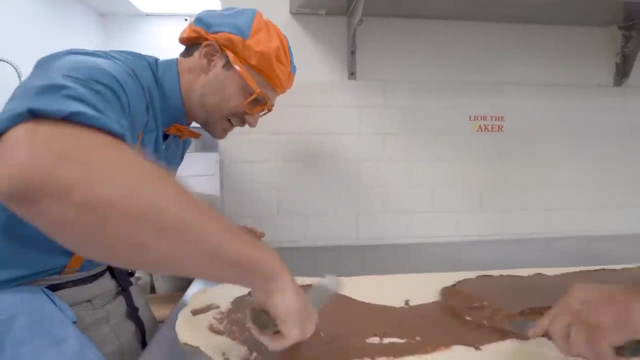 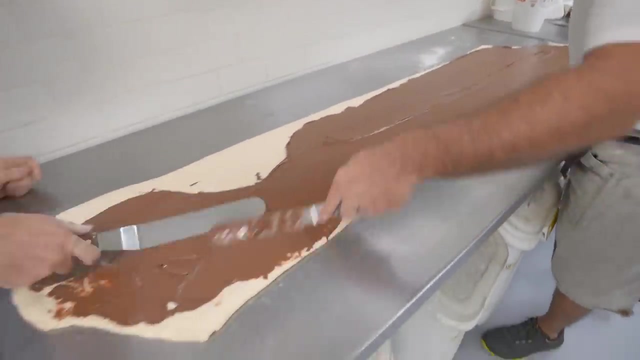 Here we go. Whoa, This is so much fun. It's kind of like an art project. Wee, You have to get it all the way to the edges, or almost to the edges. Okay, Whoa, That looks tasty. 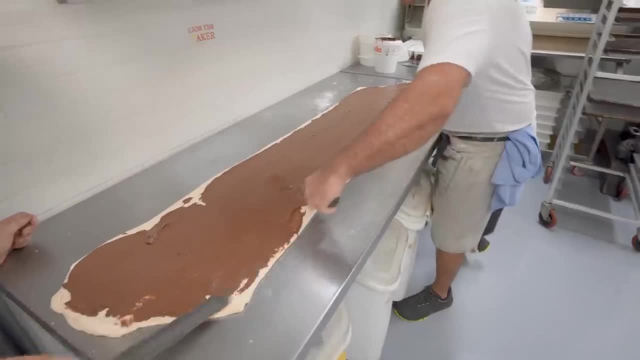 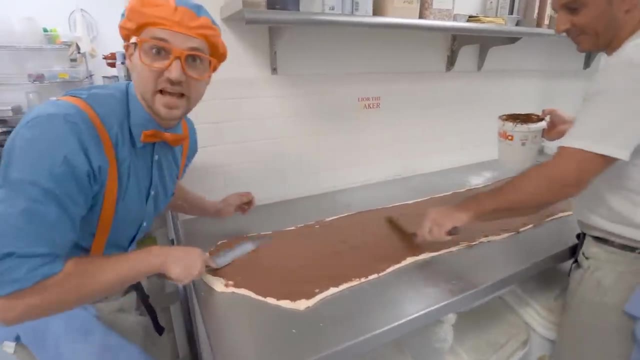 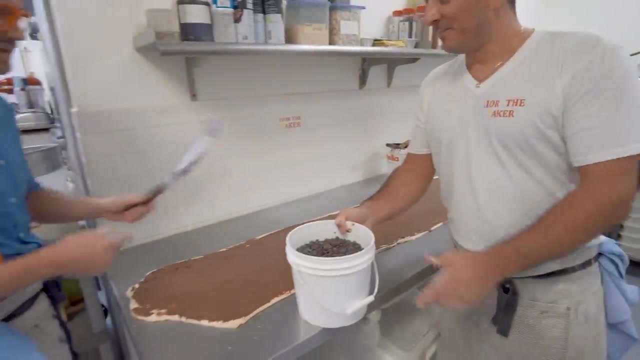 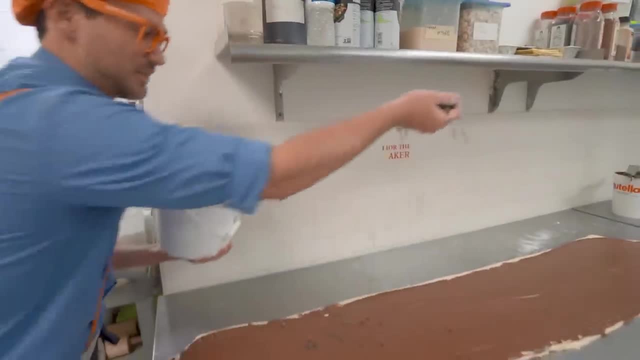 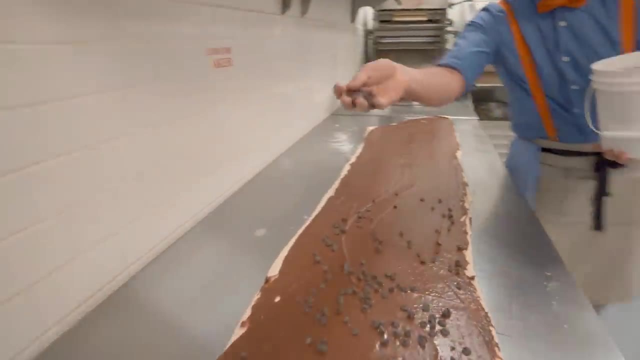 Chocolate chips time. Okay, Grab a big handful and start sprinkling. Woohoo, Whoa. Okay, That looks real good. Whoa Ha, ha, Put a lot right there. Okay, I don't know how much to do. 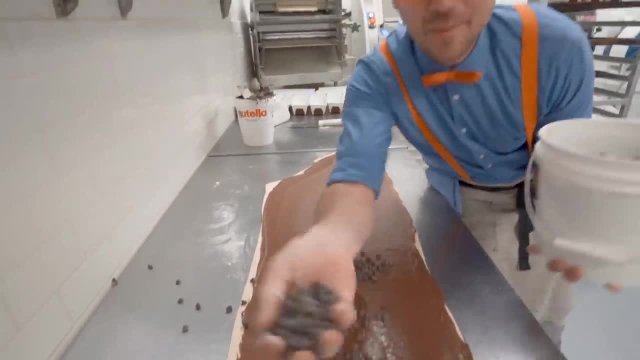 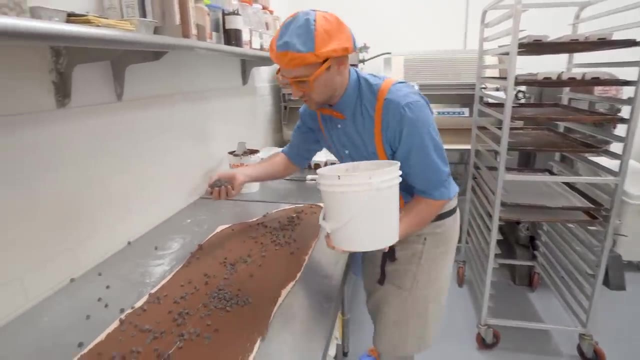 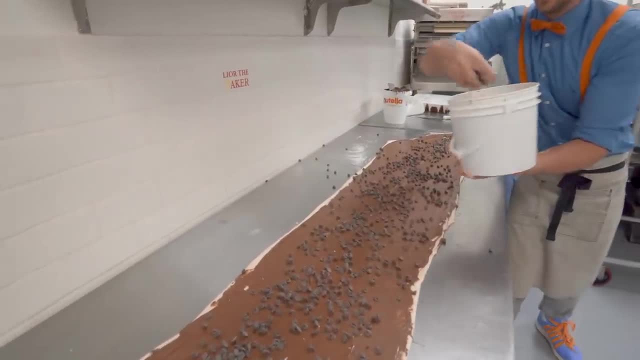 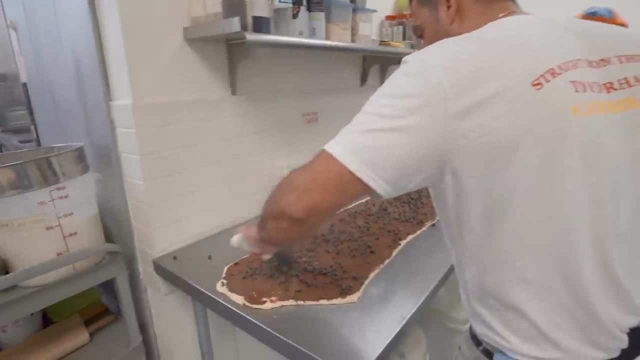 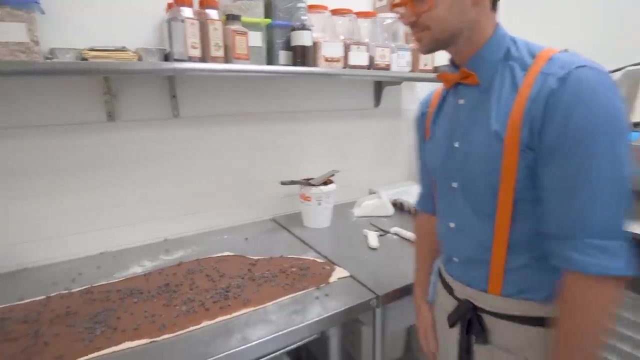 Me too. whoa, That's enough. Okay, a little bit more down here and then we're good to go. Here. we go Nice, straight line, Okay. okay, you ready to roll this? Yep, One, two, three, we're gonna roll this Slowly, slowly, tight. 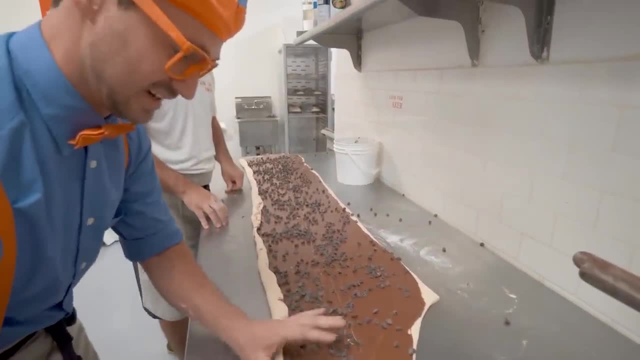 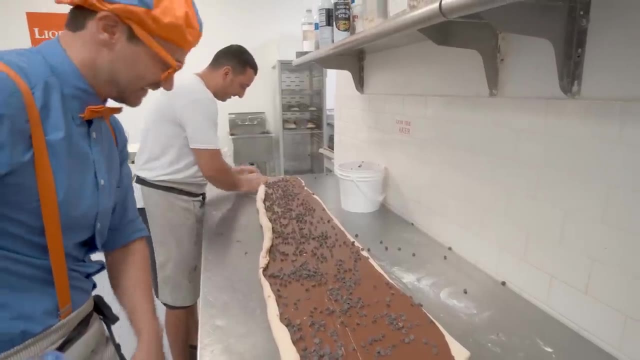 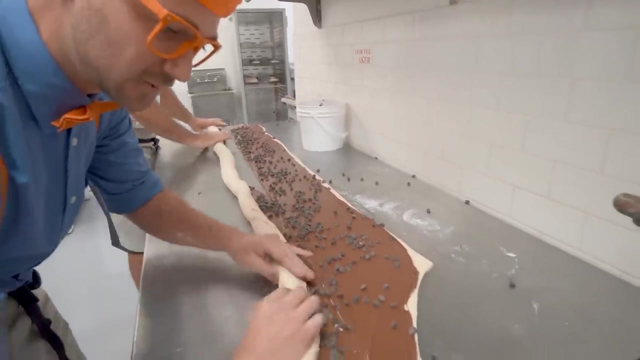 Whoa, You sure you don't do this before You look professional, Nope, first time. Yep, whoa, I'm getting dirty. Oh, oh, I guess we roll all the way. Okay, roll, roll, roll. 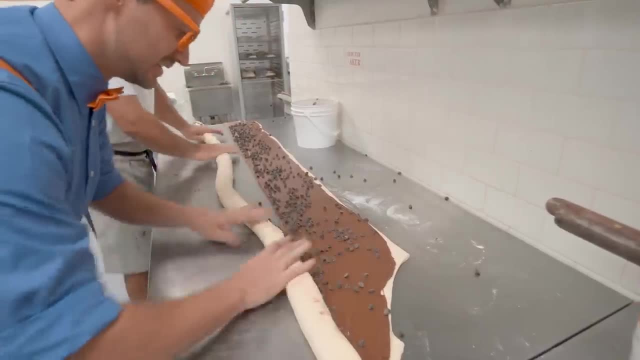 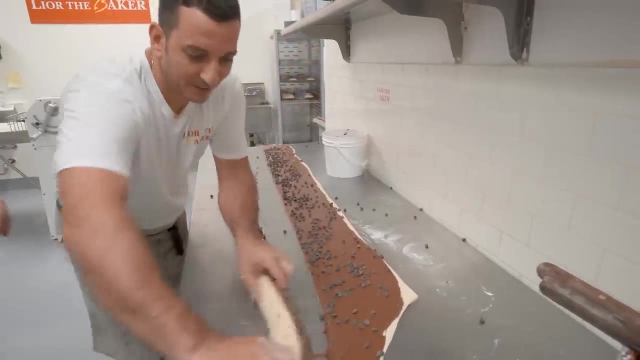 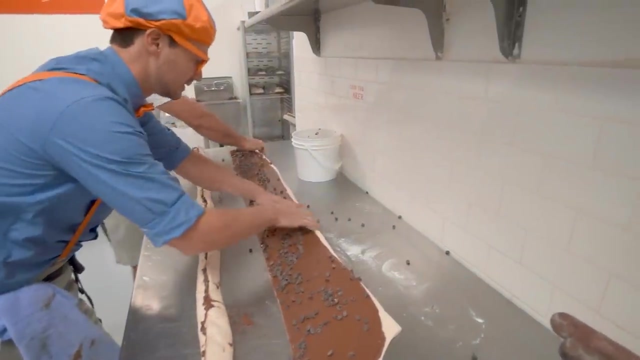 Maybe you could make something at home just like this. Haha, it's pretty hard though. Okay, how's that look? Looks perfect. Okay, let me just take it. Gonna roll it Outside inside, ready. Okay. 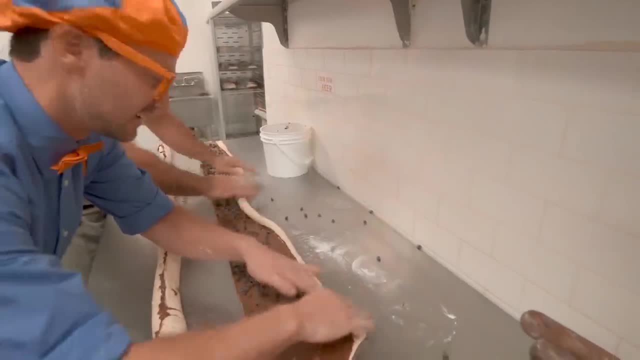 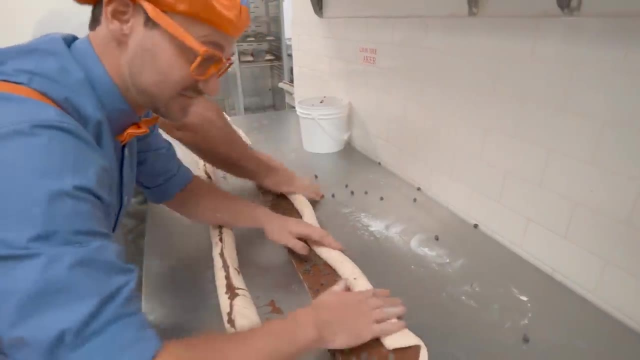 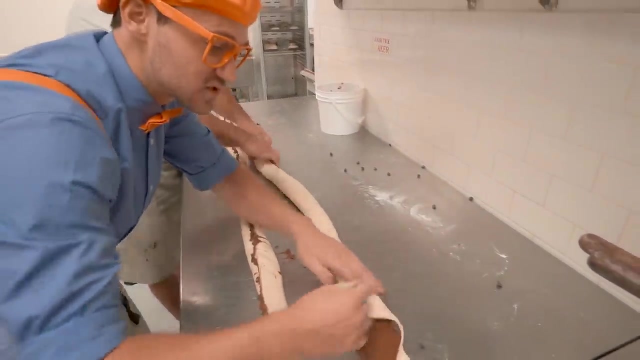 Okay, roll the outside inside. Okay, How does that look? Does it look good? Yeah, it does. Okay, It's so cool how we created this All from scratch. You know, It started out with just a few ingredients. 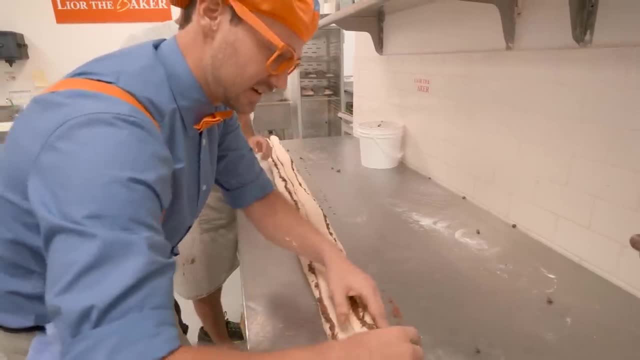 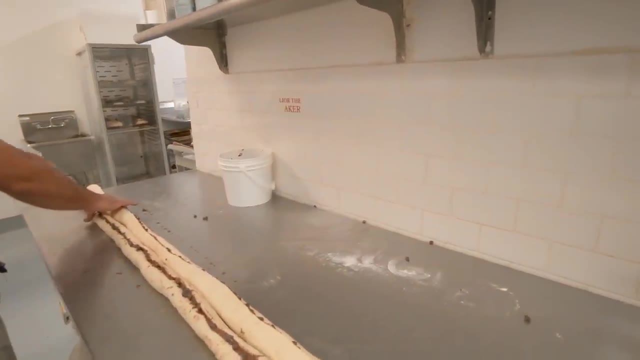 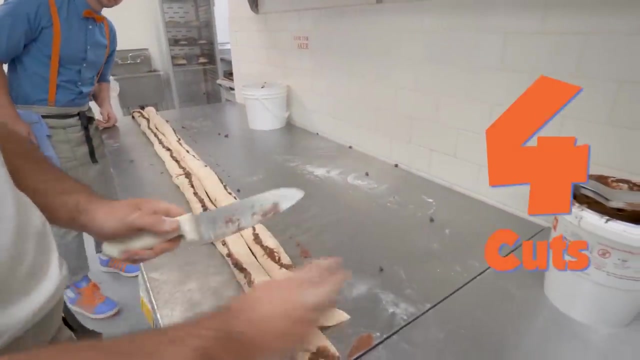 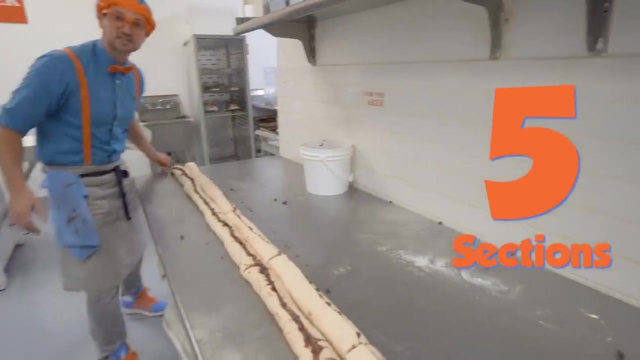 And now Looks amazing, Looks like a masterpiece. Are we going to divide these? Okay, Okay, One, Two, Three, Four, Four cuts, which makes One, Two, Three, Four, Five sections. Okay, open them. 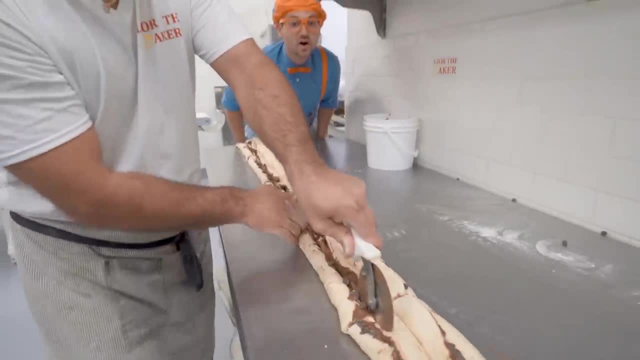 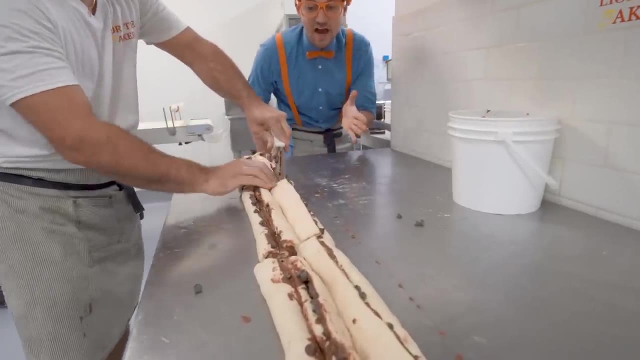 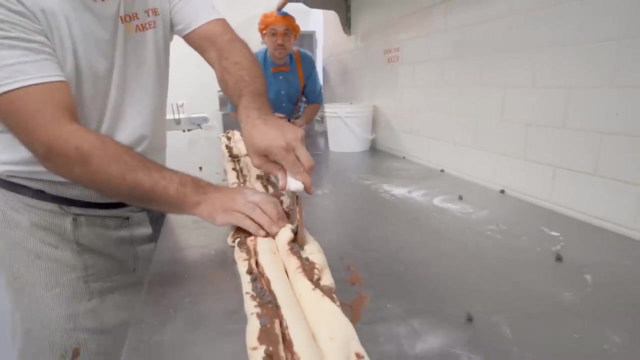 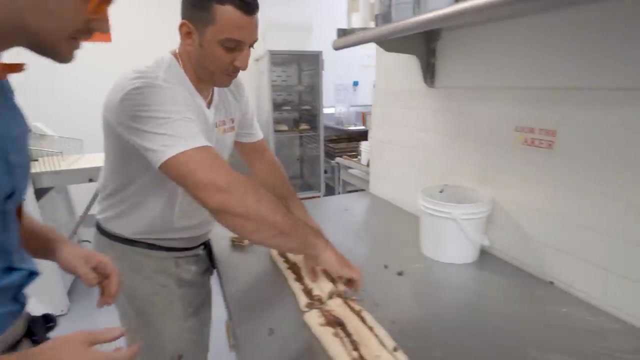 Wow, Look at it, go. Okay, He's cutting it in half The long ways. You know There's a short way and a long way. Perfect, Woo, Okay. Now The fun part: Okay, Open them Okay. 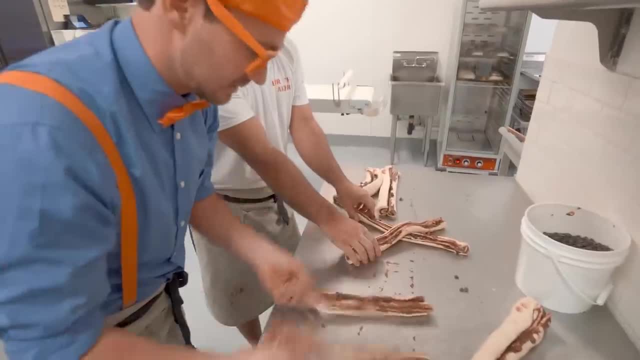 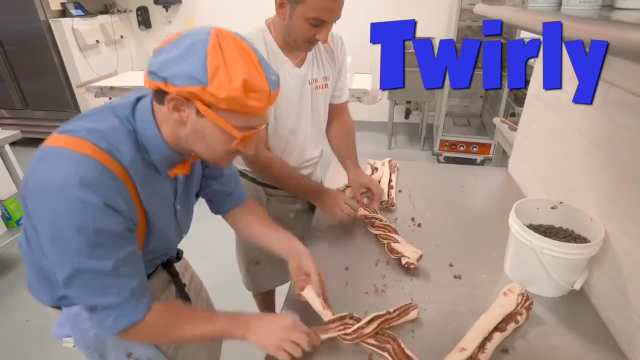 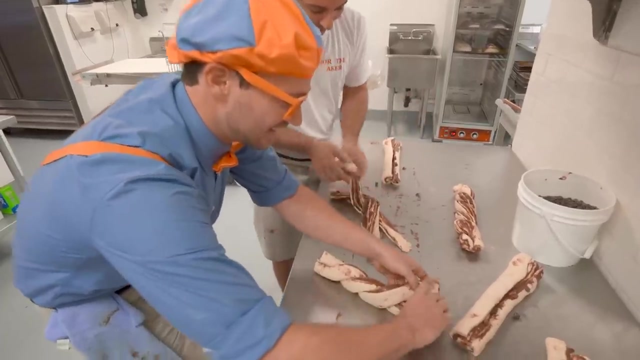 Open them, Make X- Okay And X. Then you do a little twirly. Whoa, This is so fun, This is something or what. Yeah, It's pretty messy, But Good messy, Sweet messy Yum. 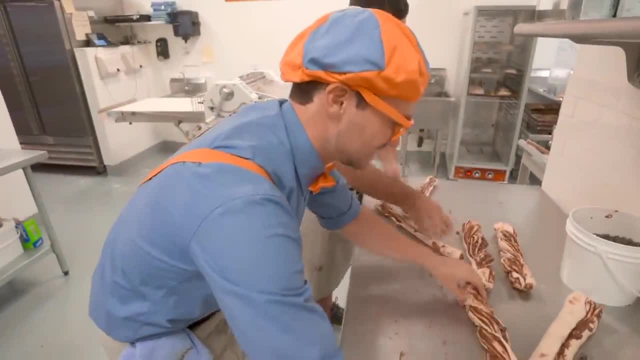 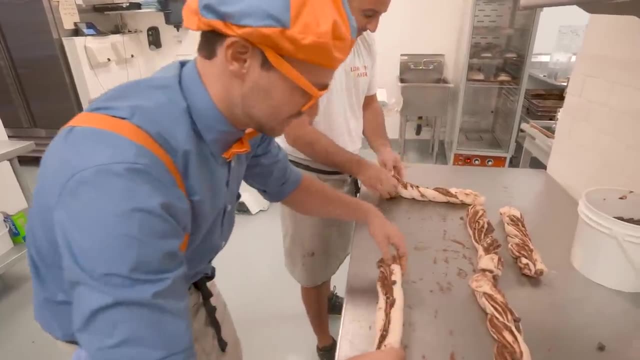 Does that look tasty? Okay, There we go, Woo. Okay, Just a few more. I'll let you do some more. Thank you, He's a lot better than me. Let's do this one. Okay, Divide them by two. 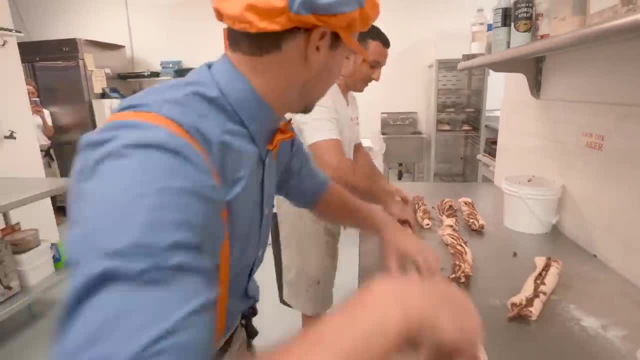 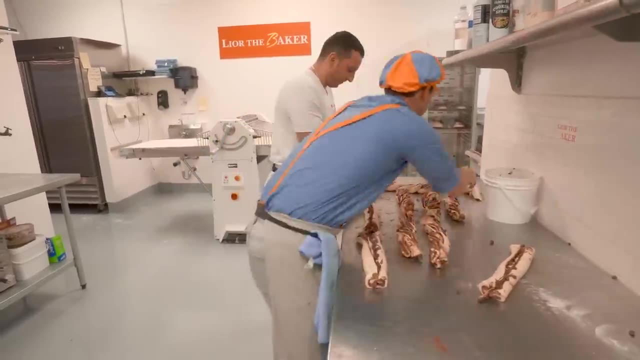 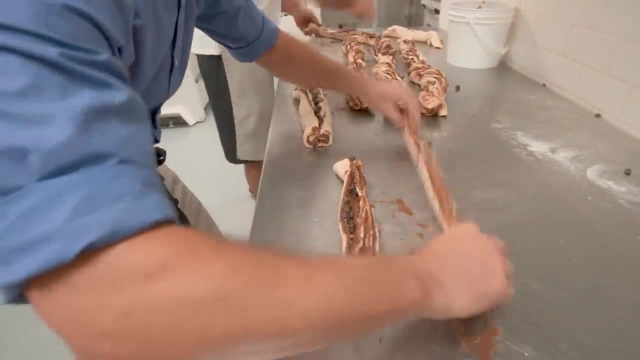 And then Do a cross. Okay, One, Two, Three, Four, Five, Six, Seven, Eight, Nine, Ten, Eleven, Twelve, Thirteen, Thirteen, Fifteen, Fifteen, Fifteen lements. Do a cross. 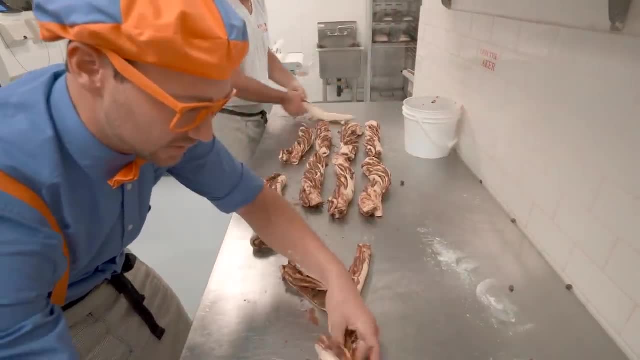 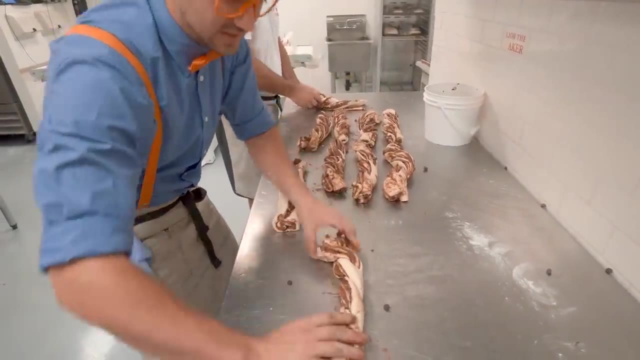 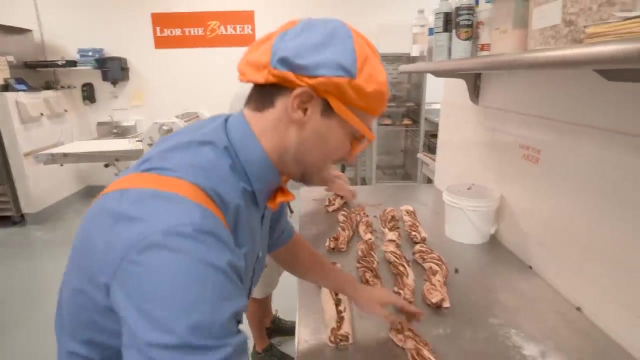 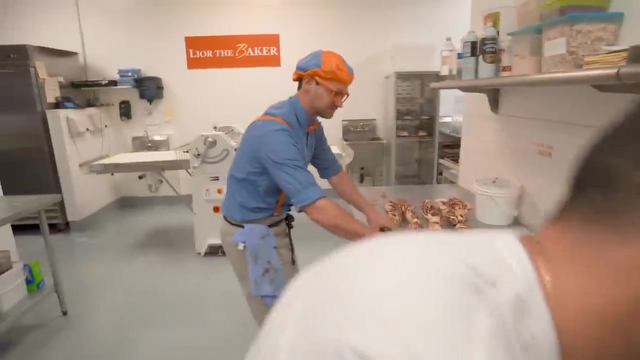 Kind of like an X, And then do a little twisty, And then do a little twisty And there you go. Look at that, Yum, Whoa. Okay, Here's another one. I'll do the last one. 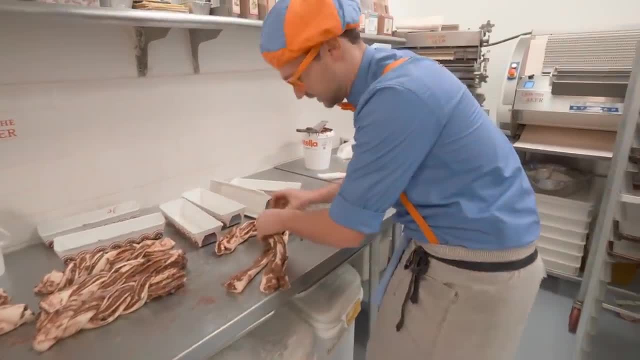 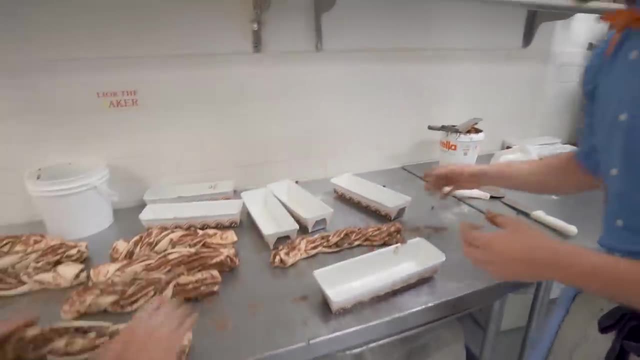 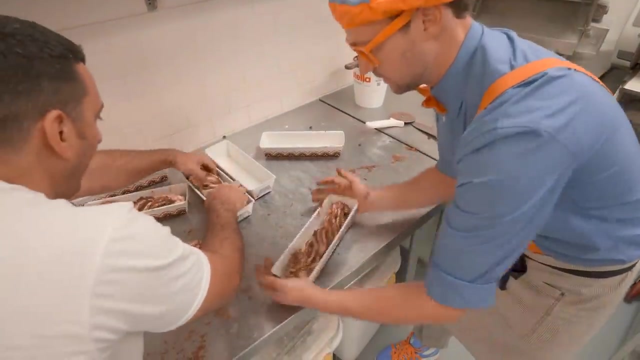 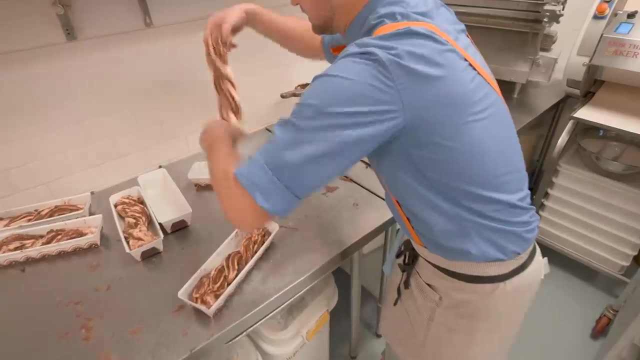 So it looks like we're putting them in those boxes. Okay, so here's the box and we put this inside. inside, let's get roofing. whoa, look at that. wow, whoa, oh, thank you. okay, whoa, and there's. 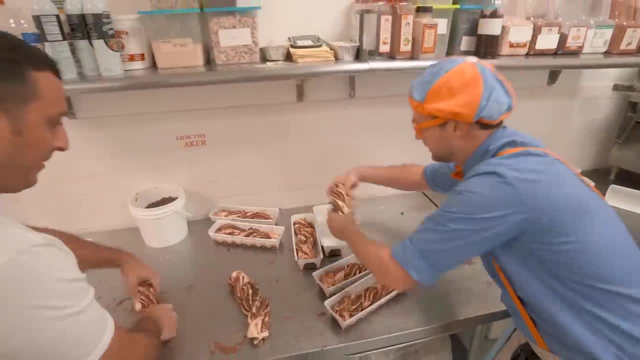 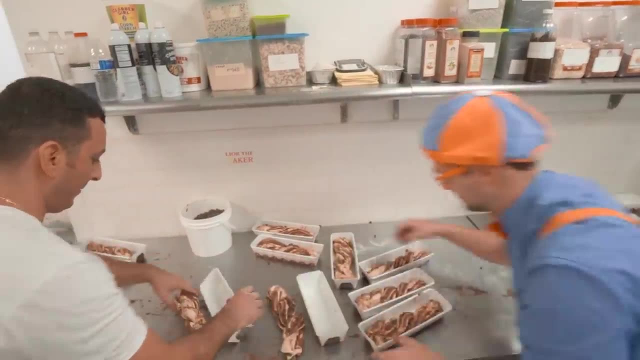 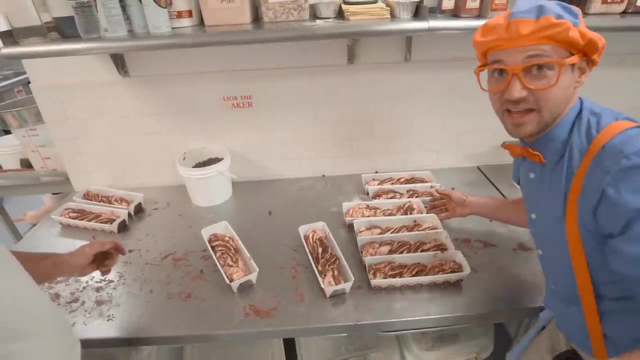 another one. yum oh, thank you, whoa. oh, okay, two more boxes. wow, look at how tasty these look. okay, now we need the proof and then we can bake them. good job, whoa, doesn't. 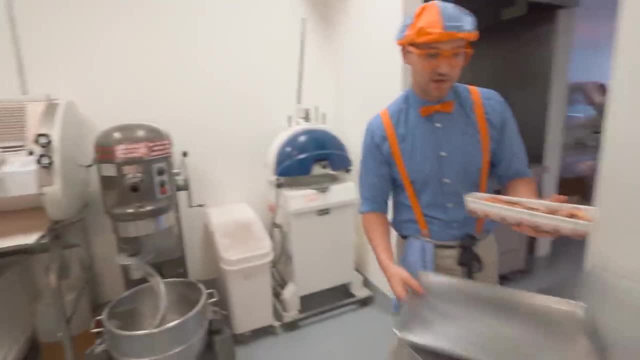 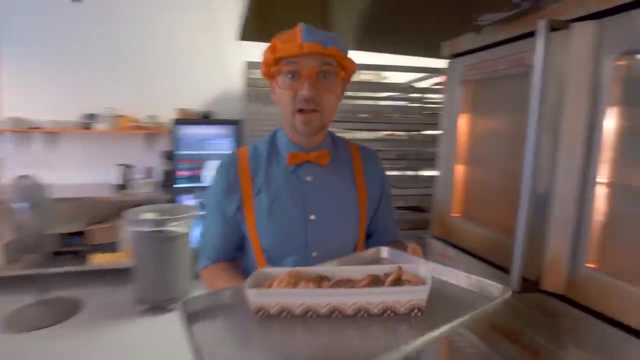 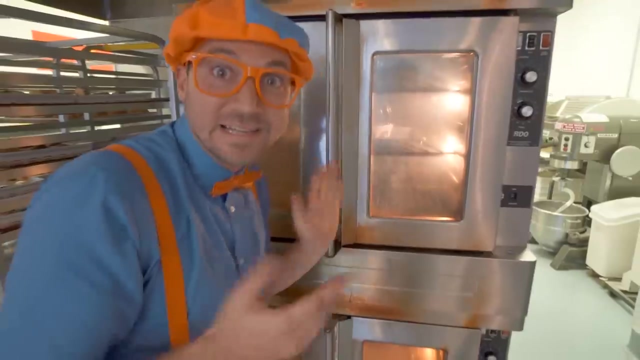 that look good. okay, let's put it on the tray right here and then let's put it in the oven. Whoa, all right, here we go. it's nice and hot in there. whoa, now we get a weight. yeah. 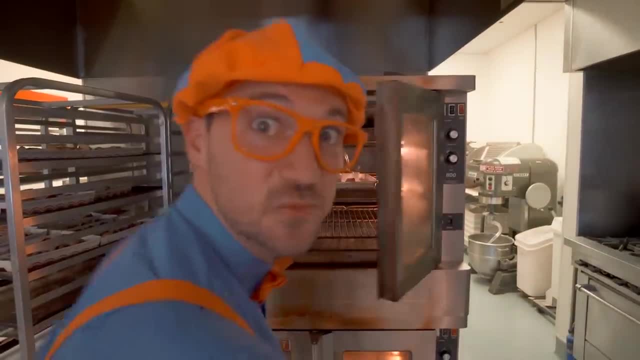 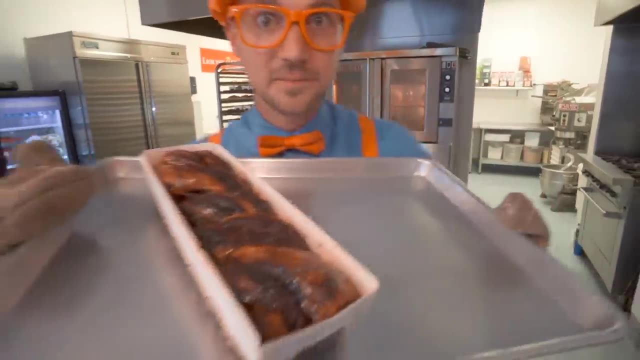 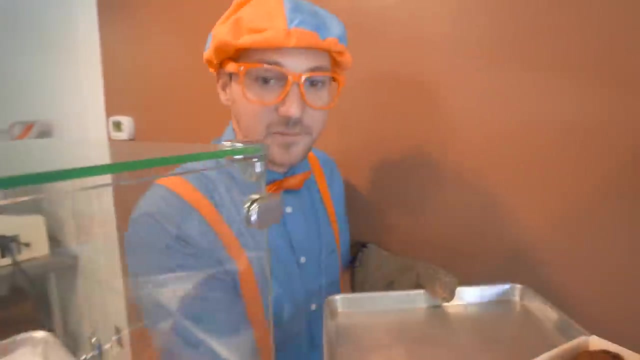 whoa, it's ready. whoa, yum, look at it. yum, yum, yum. okay, let's go to the front, so then we can eat some. okay, here we go, Here we go. whoo, ooh, you want some chocolate babka. 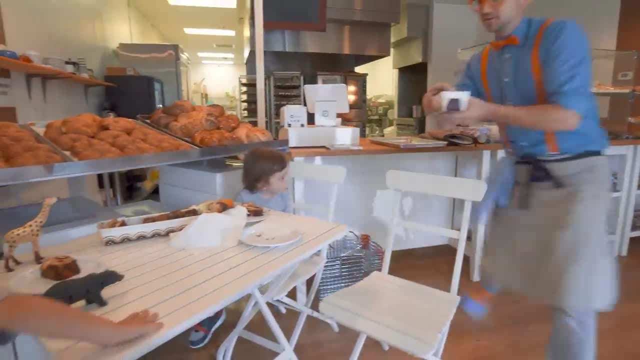 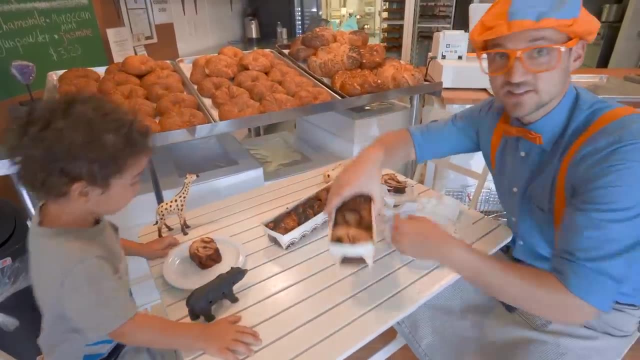 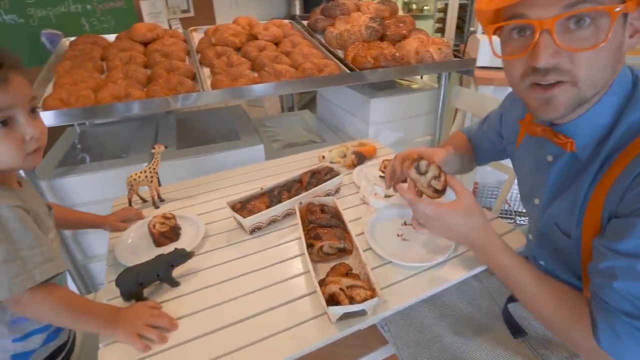 Yeah, Okay, here we go, all right, yum, yum, Can I have a piece? Okay, let's try some. okay, mmm, oh, it smells so good. Mmm, mmm, Whoa, oh. 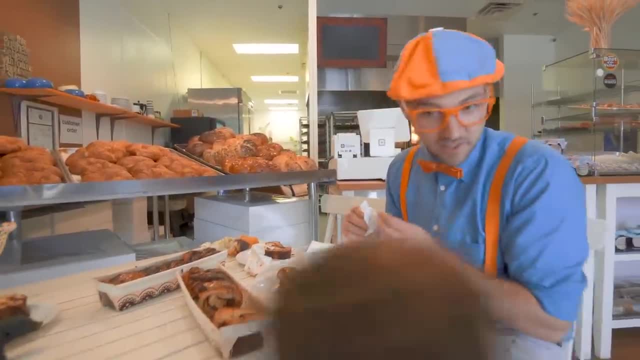 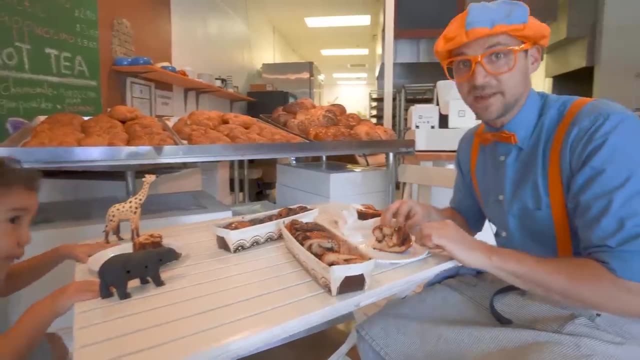 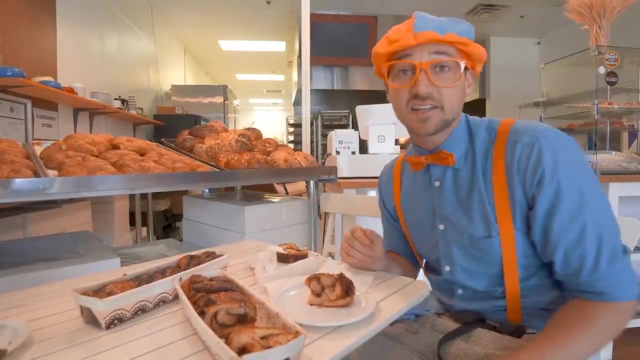 Mm-hmm tastes really good too. Hey, do you like yours? Oh, It was so much fun baking all these goods with you today at Leor the Baker's place in Scottsdale's, Arizona. Well, this is the end of this video. 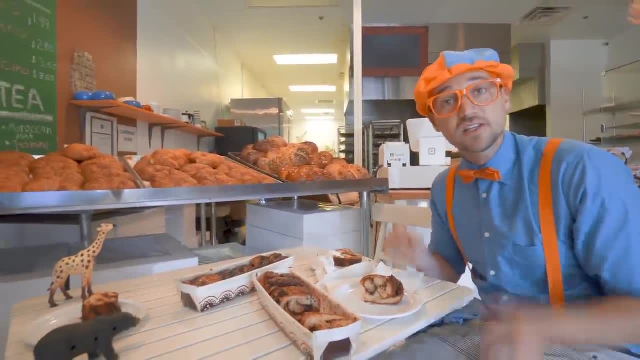 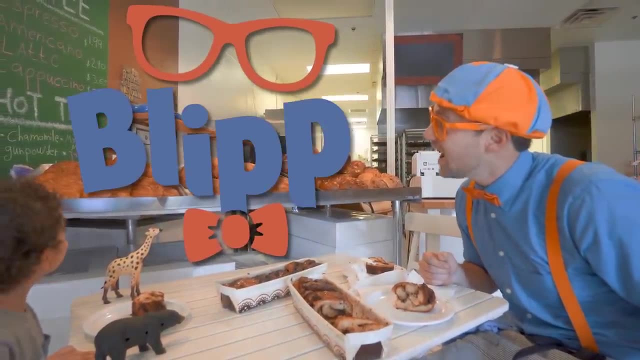 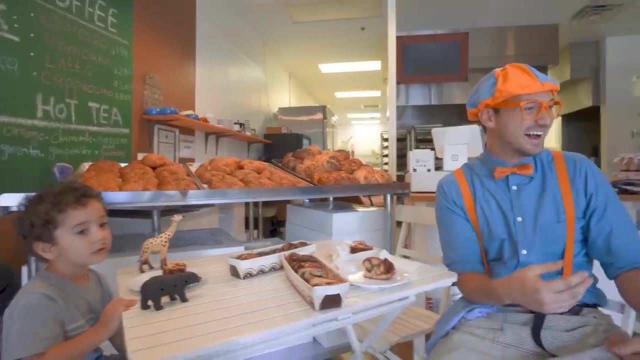 But if you want to watch more of my videos, all you have to do is search for my name. Will you spell my name with me? B Li P P I Blippi. good job, Well, see you soon, Bye, Bye, See you later. 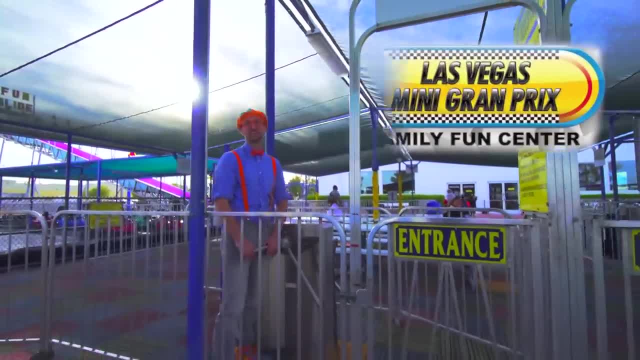 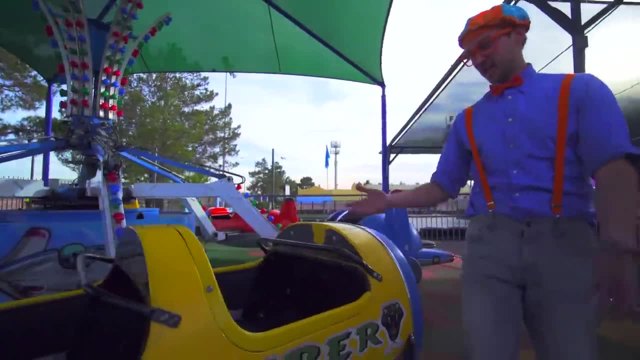 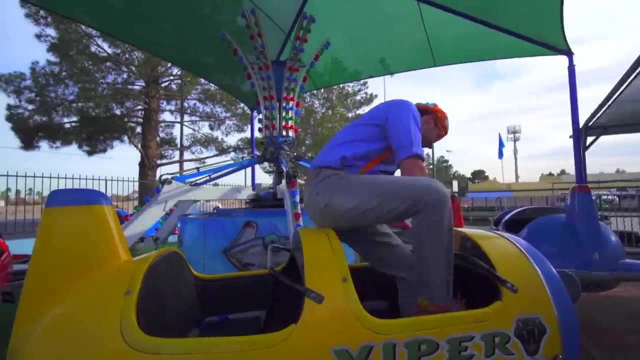 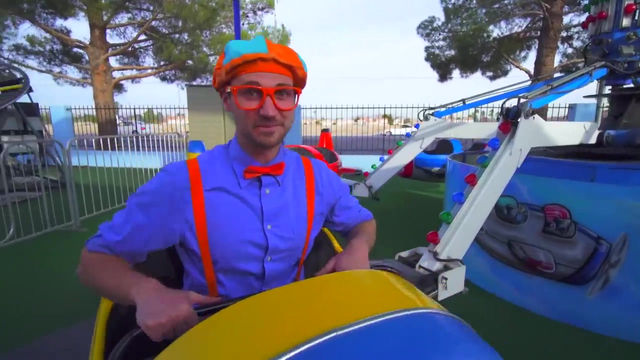 And today we're at Las Vegas mini Grand Prix, and the great thing about this place is it has rides Like this. This is the airplane ride. I think you and I should ride it. Here we go. Once you're in the airplane, you need to buckle up. once you're buckled up, you're ready to ride. 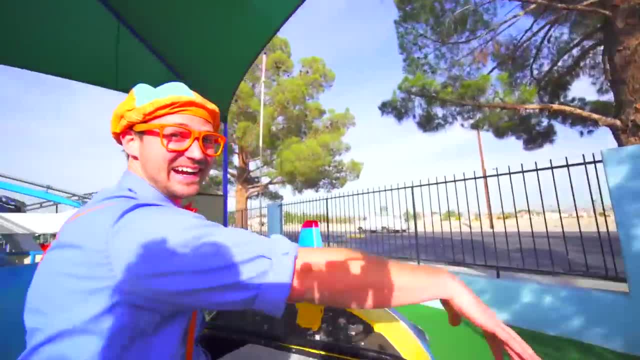 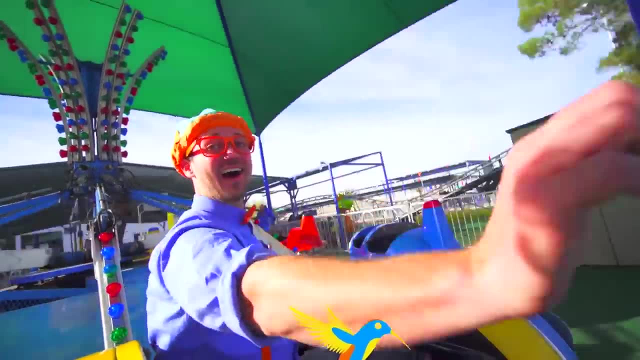 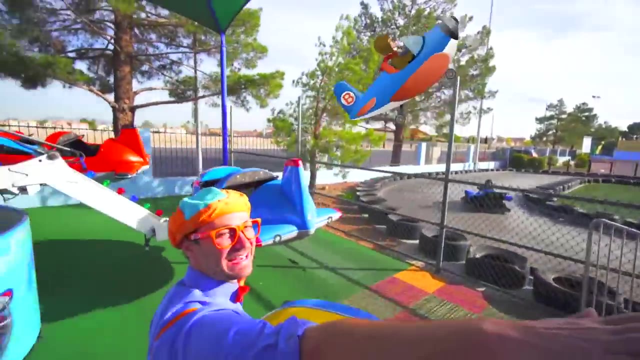 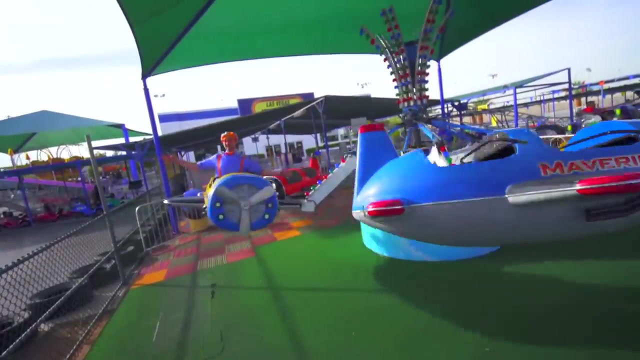 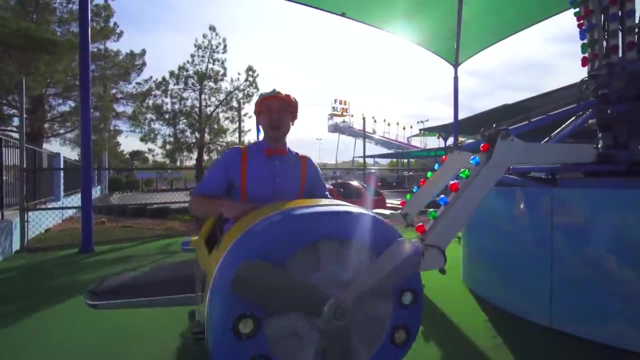 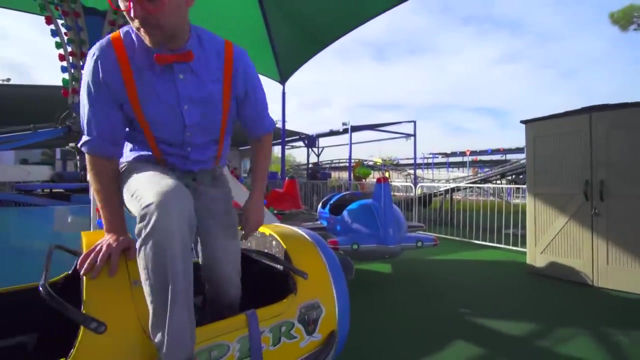 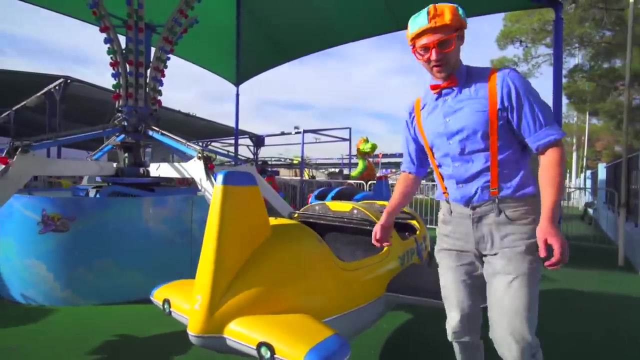 Yeah, like we're flying in the air, I'm a bird. Wait a second. I'm not a bird, I'm a plane. That was so much fun Riding this airplane ride. Yeah, this airplane that we just rode. This was the color yellow. See what other ones there are. 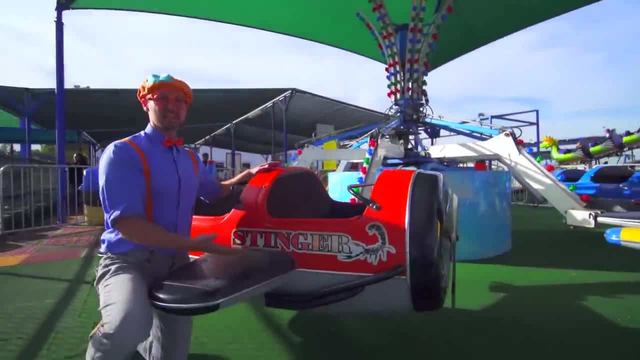 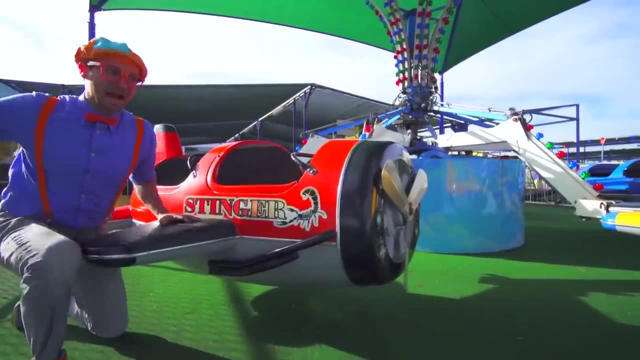 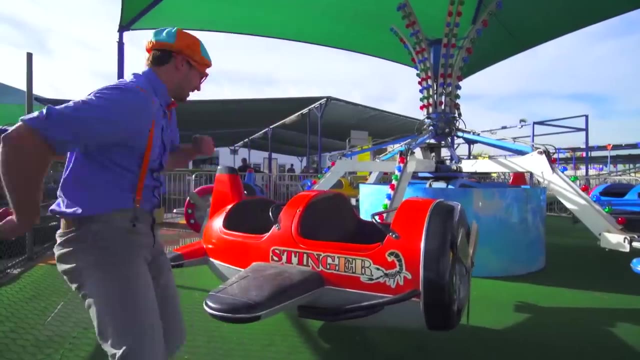 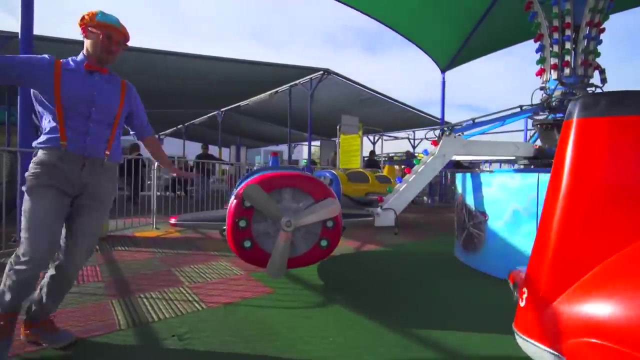 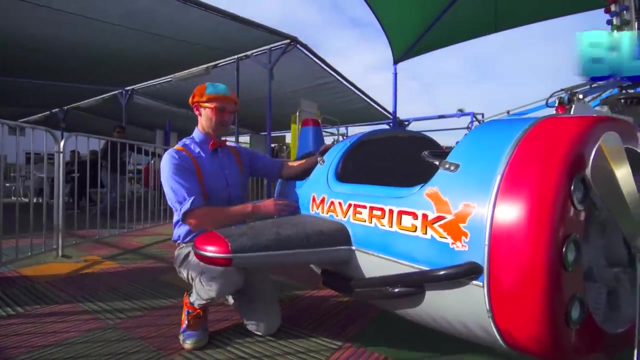 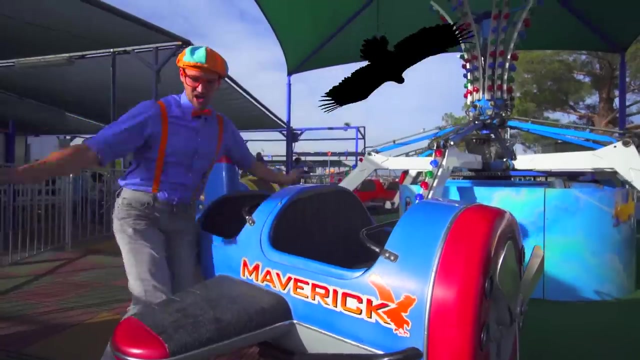 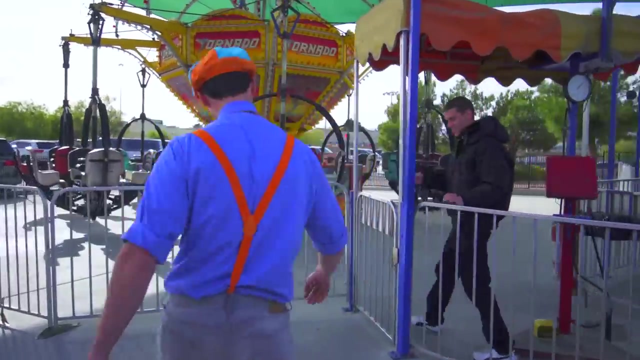 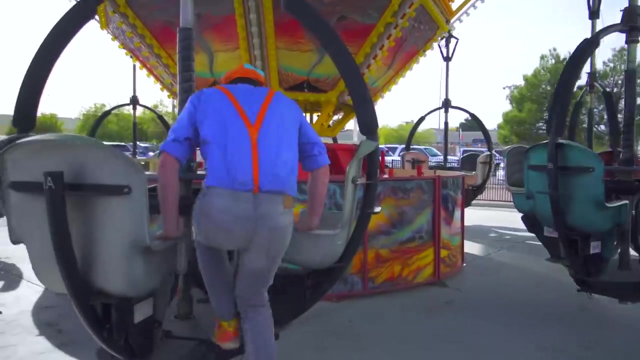 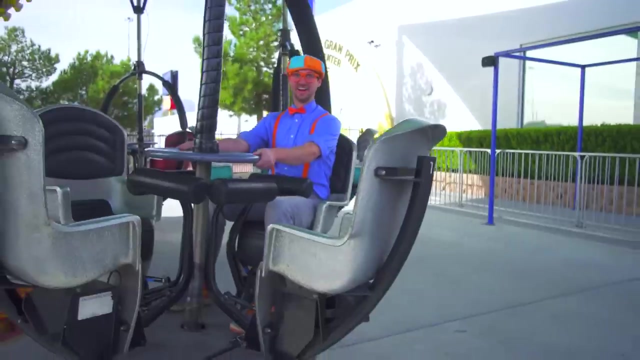 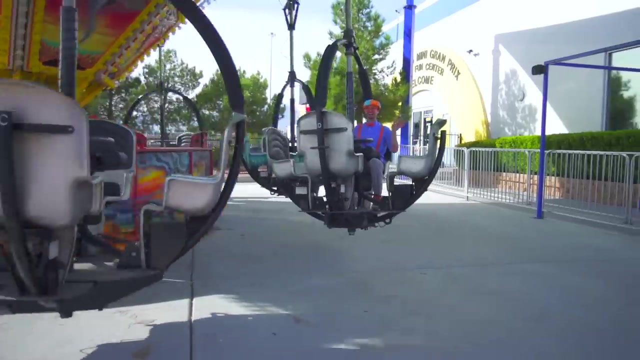 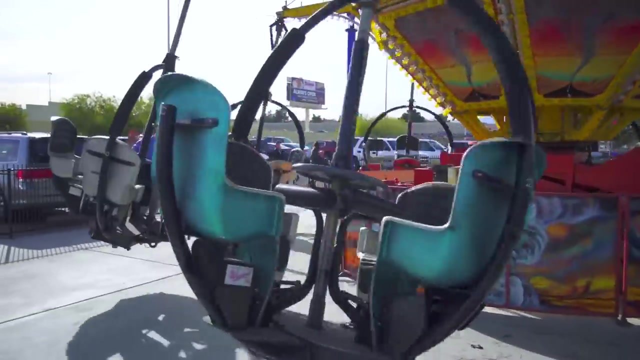 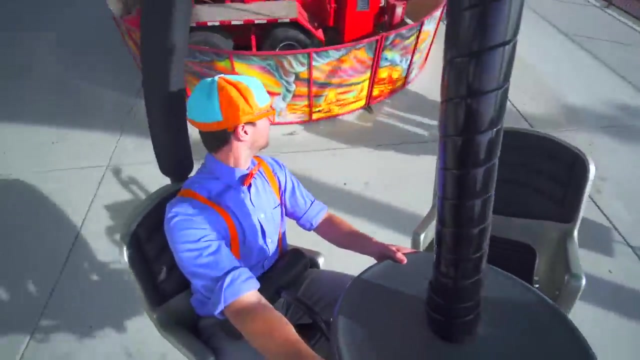 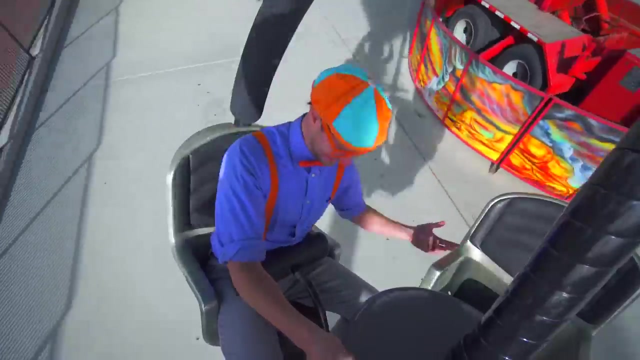 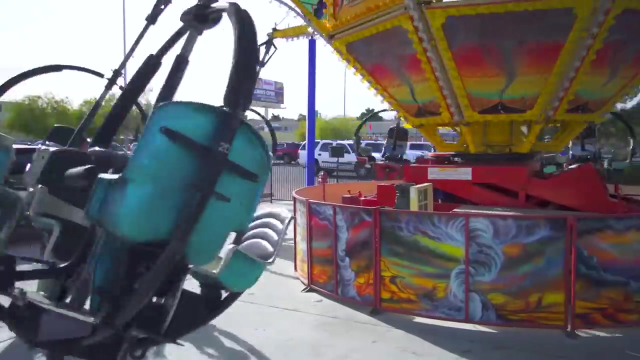 Look at this airplane. This airplane is the color orange. It's name is stinger- like a scorpion, you. This airplane is the color blue, It's favorite, yes, like a bird. and Oh, I wonder what this ride does. Whoa, we're spinning so fast and going around. whoa, whoa, whoa, whee, hello. 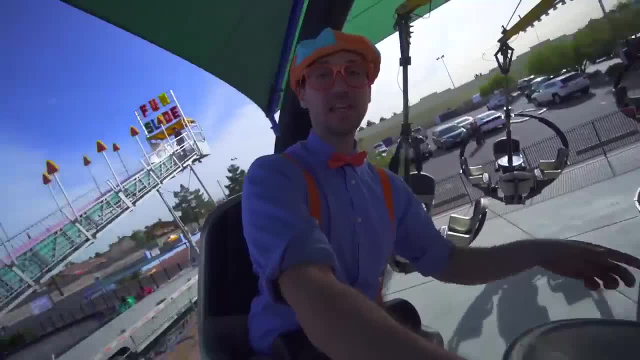 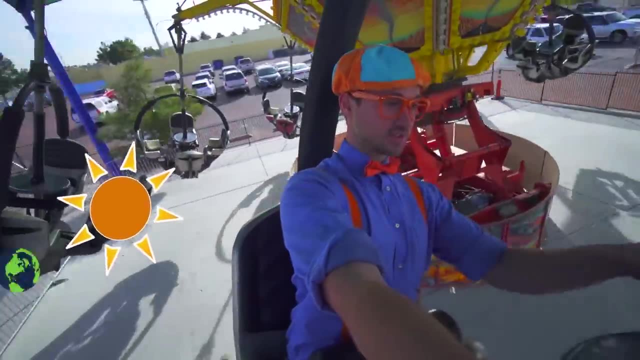 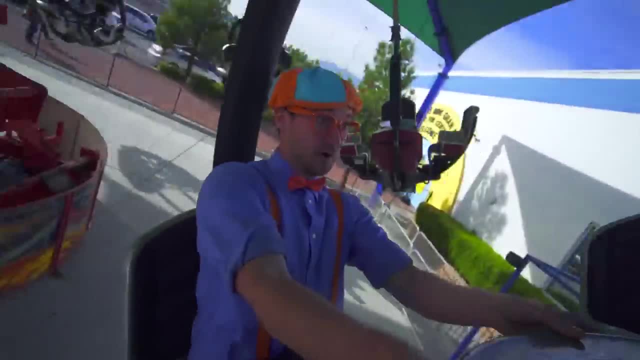 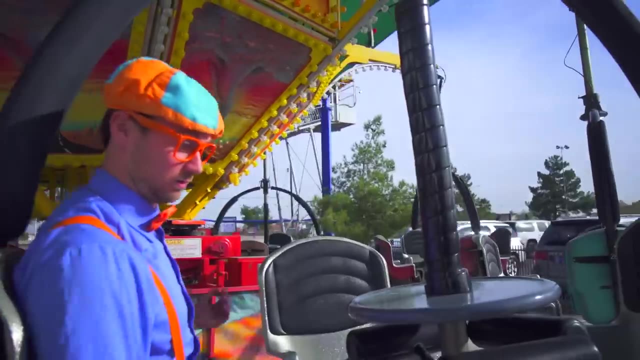 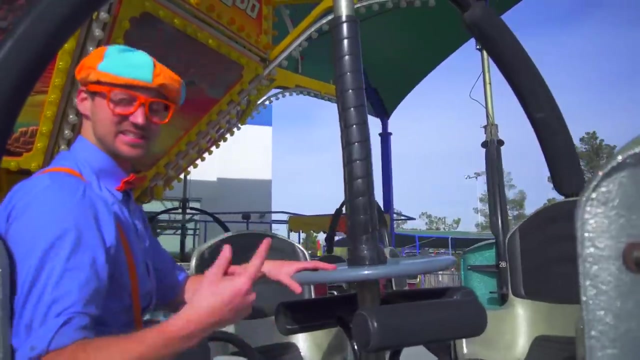 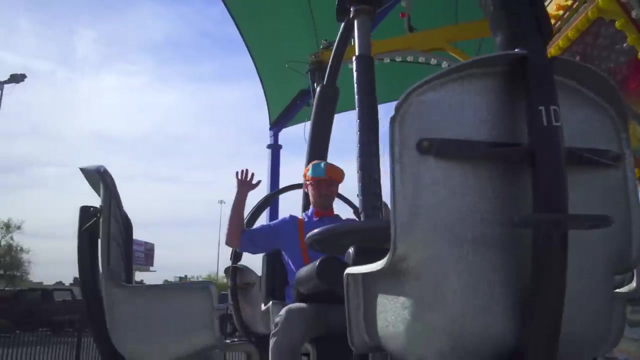 Whoa, whoa, whoa Wow. I am really dizzy now. That was so much fun riding that ride that just kept spinning around and going in the air. Whoo Wow. thank you so much for riding it with me. 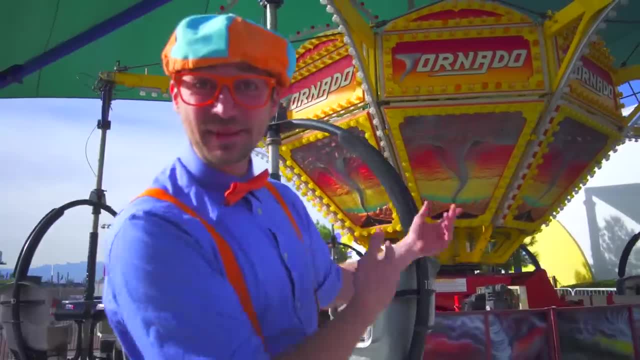 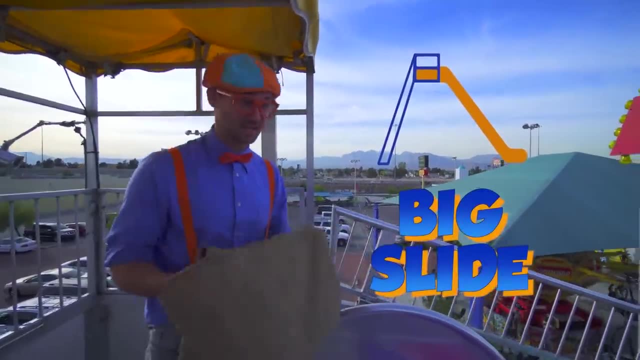 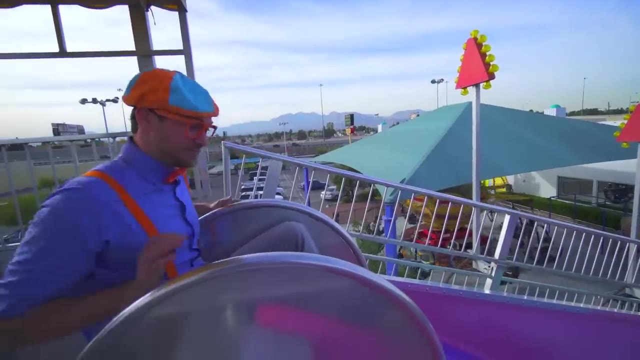 Let's go ride another ride. Whoo, now we're at the top of the big slide. So to go down you have to put your back down right here. then you sit down, put your feet in the hole and whenever you're ready, you go. 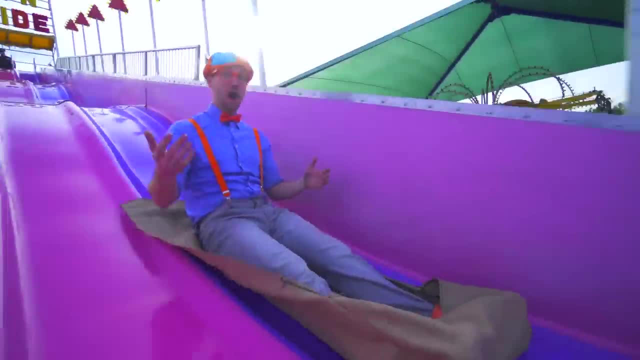 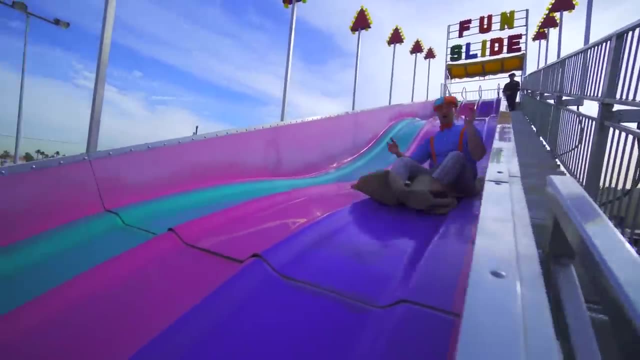 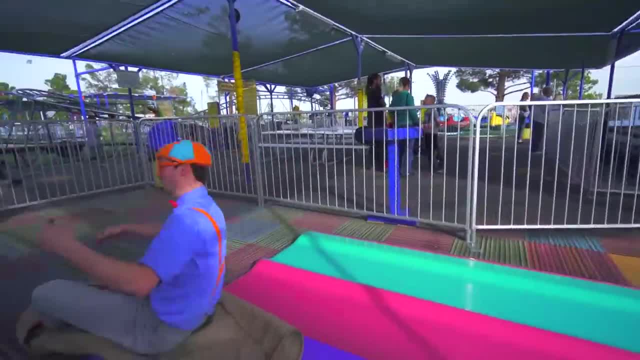 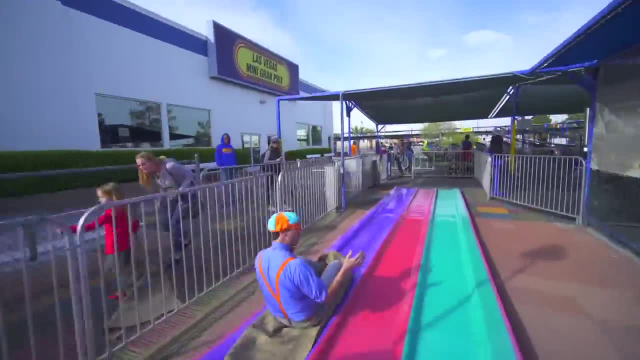 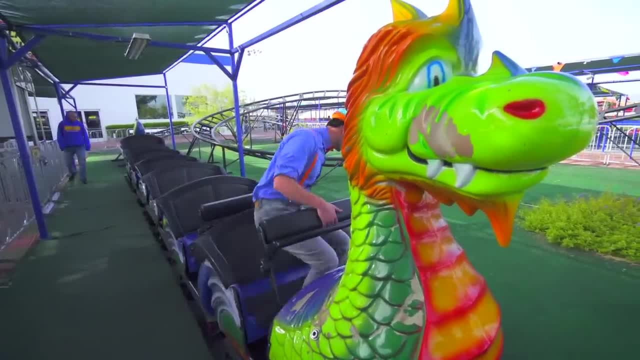 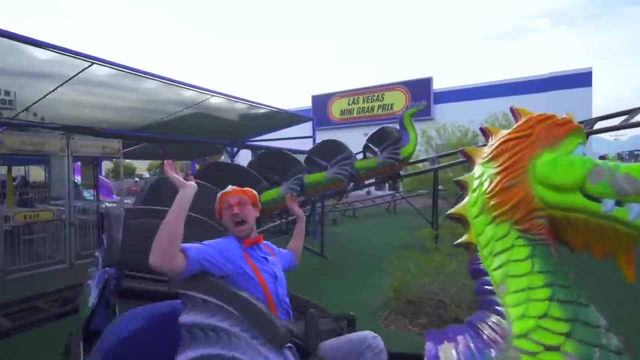 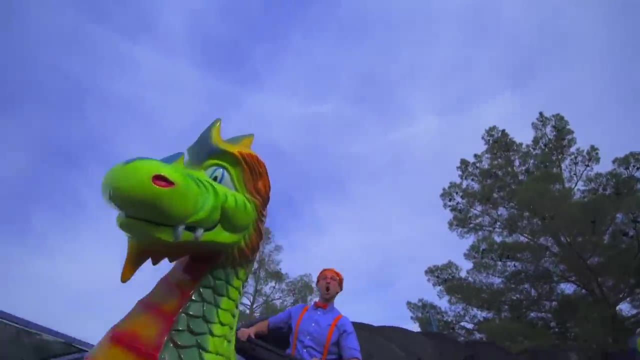 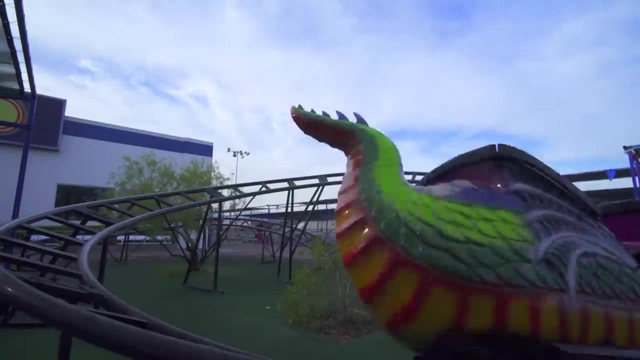 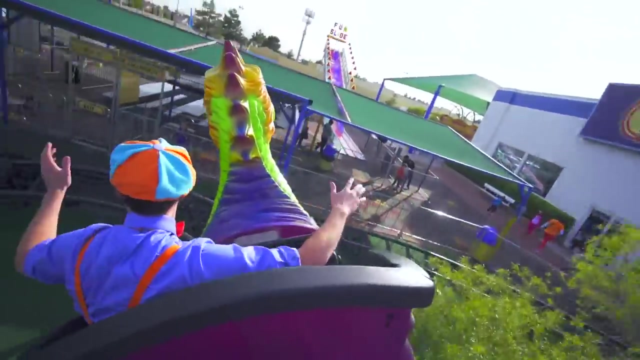 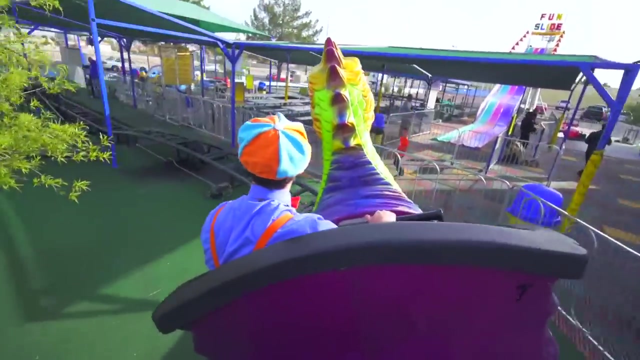 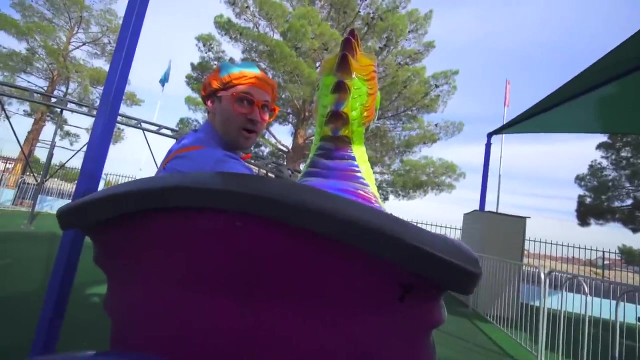 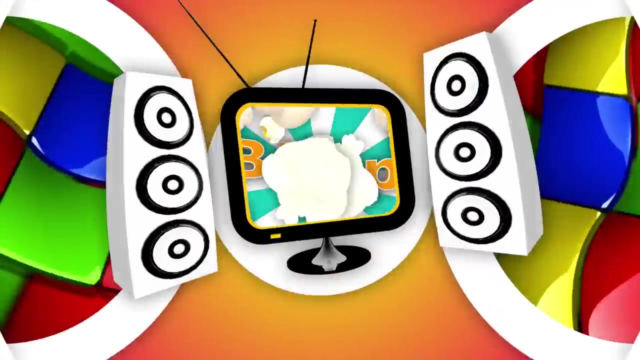 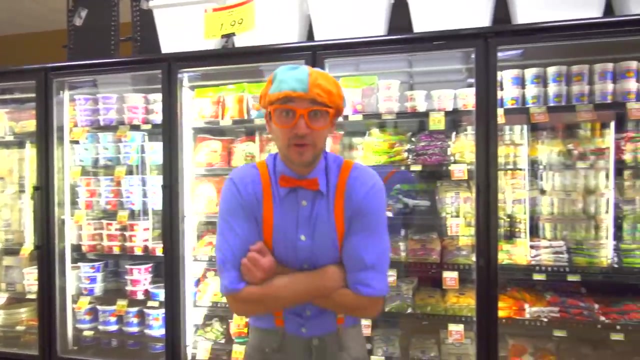 Whoa, Whoa, Whoa, Whoa, Whoa, Whoa. Yeah, Good job, That was so much fun. Here we go. That was really fun riding that dragon coaster. Wow, Look at where we are. We're in the frozen food aisle in the grocery store. 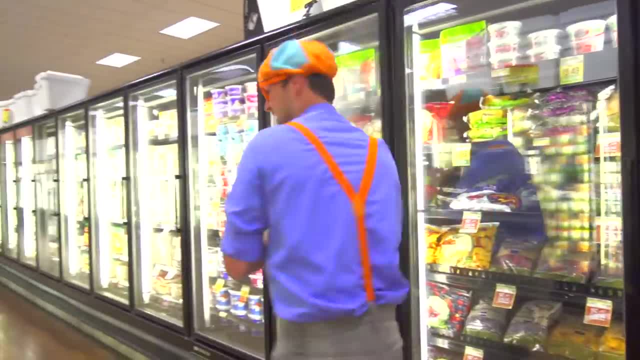 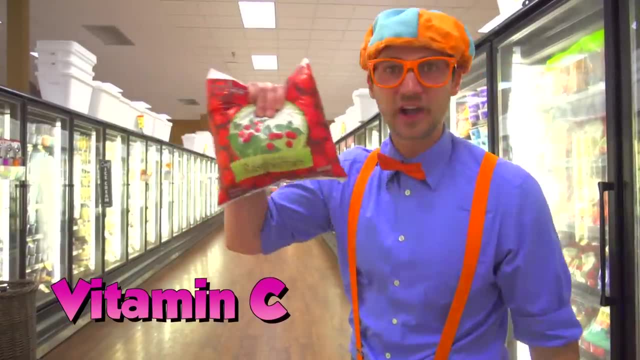 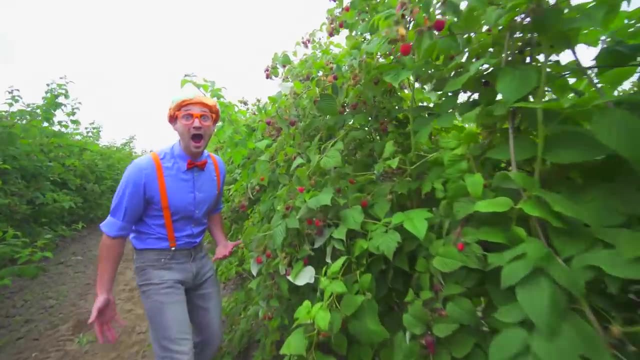 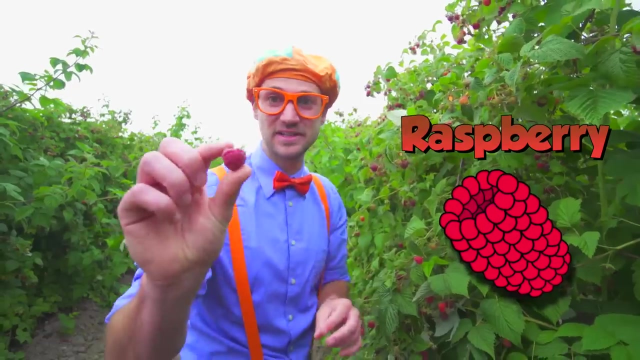 But look at what it is. Yeah, Frozen raspberries. They're so sweet and high in vitamin C I wonder how these raspberries got here. Wow, Look at all of these raspberry bushes, And all of these raspberry bushes have raspberries on them. 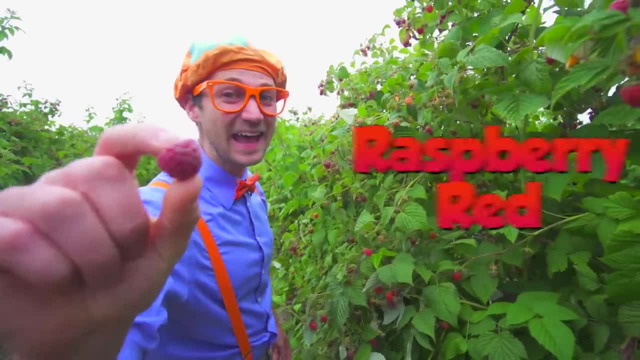 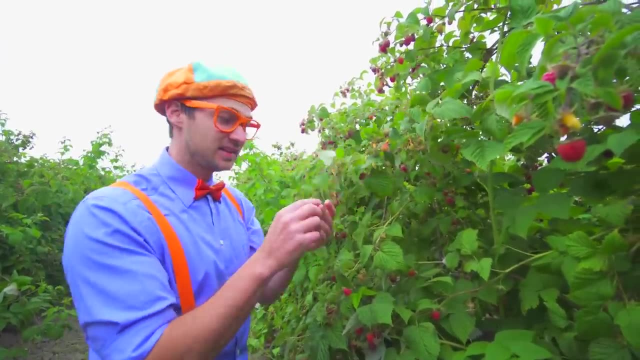 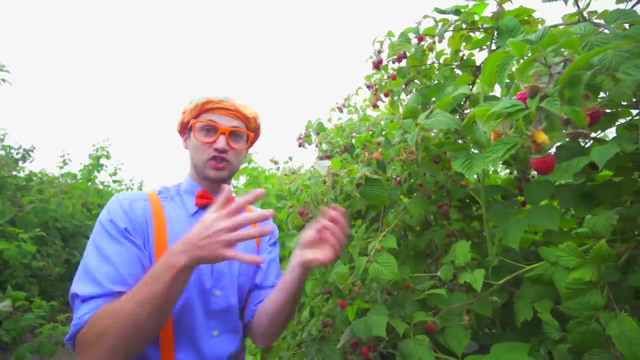 And this is the color- raspberry red, And it's so tasty. Well, since we're picking these to be frozen, we pick them at the perfect ripeness And actually we don't pick them, we shake them off with the harvester. 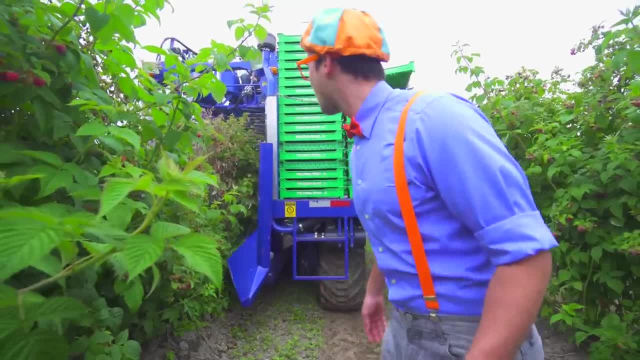 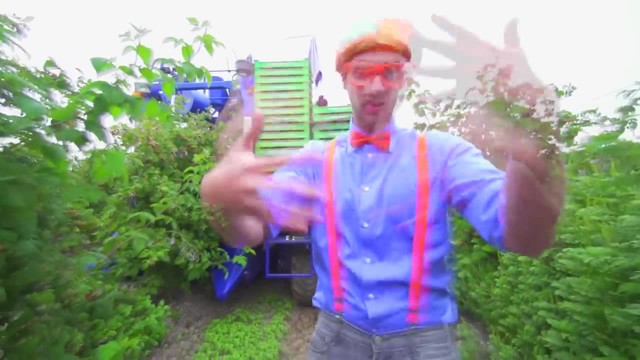 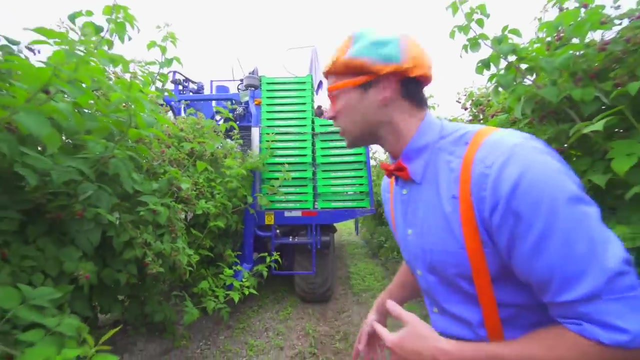 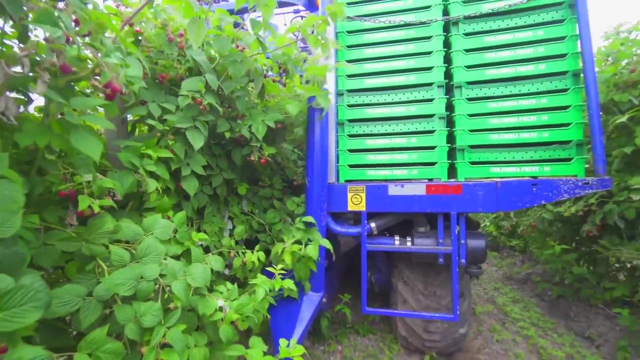 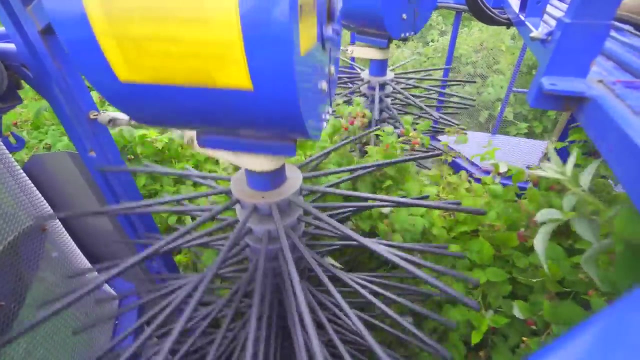 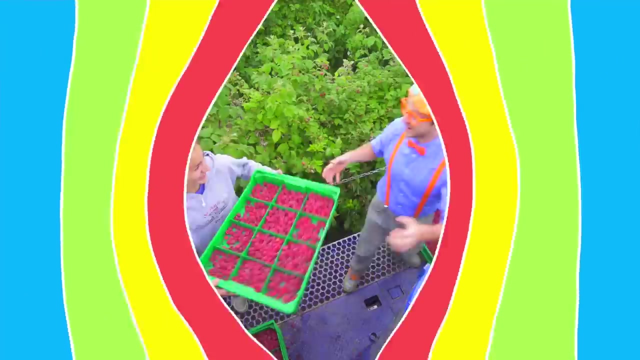 Wow, We're in front of the harvester, See, And deep in there it's shaking these bars like this, And so then the really ripe raspberries fall off into the harvester. Look, So now we're on the harvester. 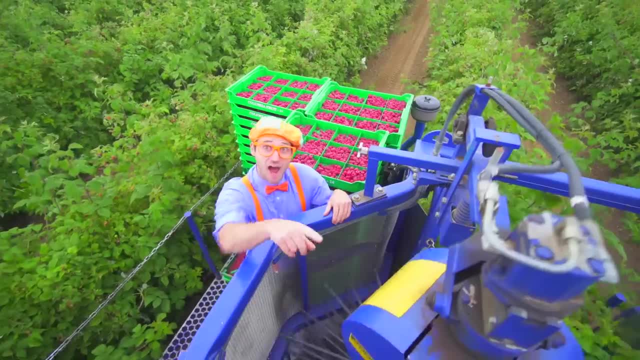 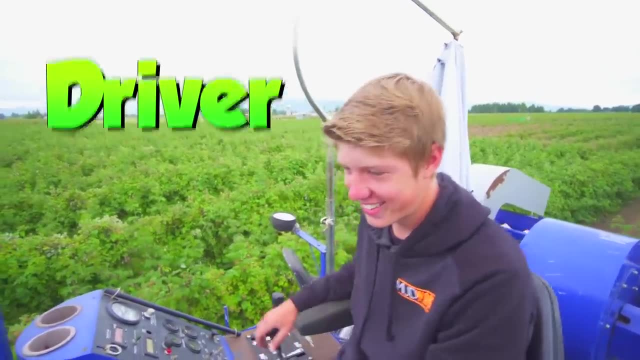 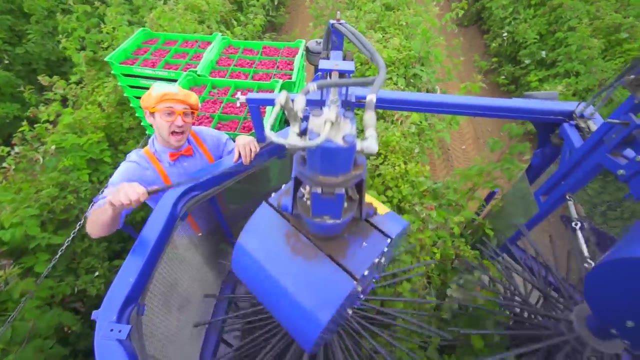 This is the machine that gets the raspberries off of the bush. And look at the driver. Hey guys, I'm the driver, See, And the driver operates the harvester And these things- yeah, they're plastic bars that go up and down real quick. 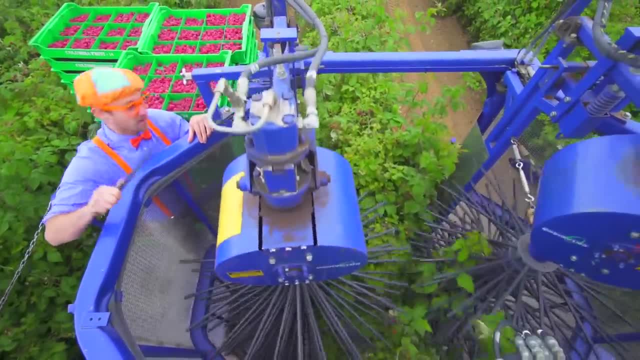 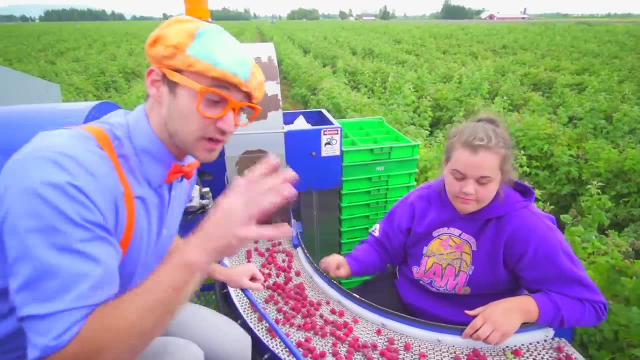 and shakes the raspberries off of the bush. Okay, now that the raspberries were shaking off the bushes, they arrive on these conveyor belts. So what do you do? I look at all the raspberries and pick off the bad ones. 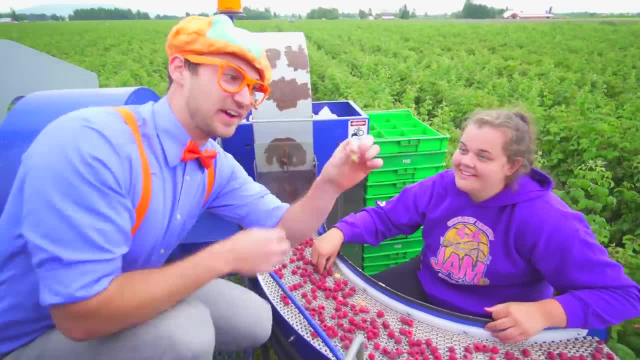 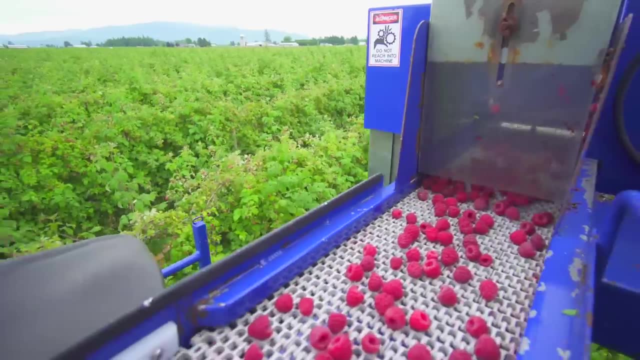 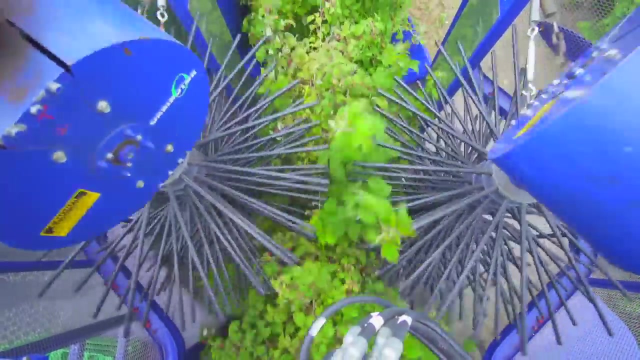 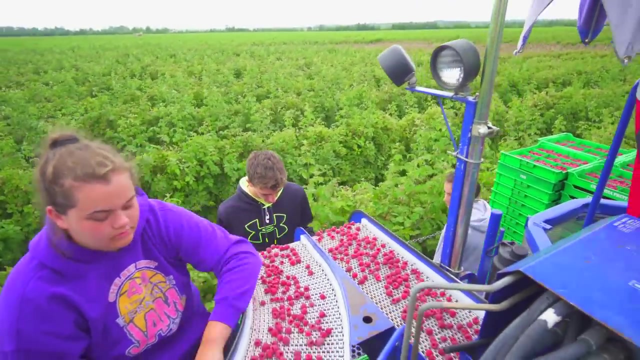 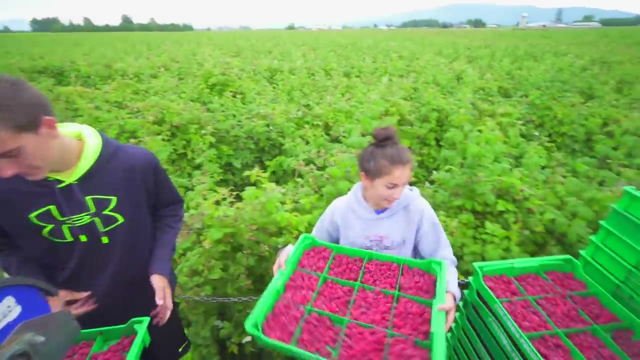 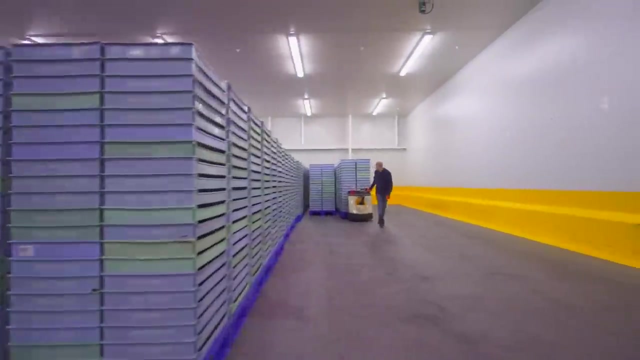 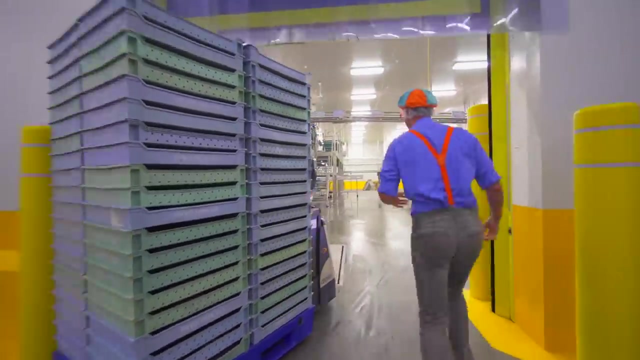 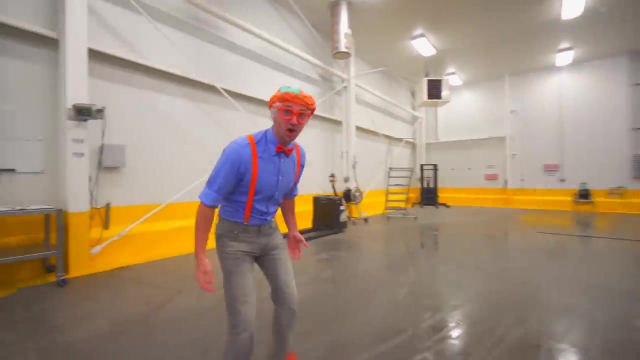 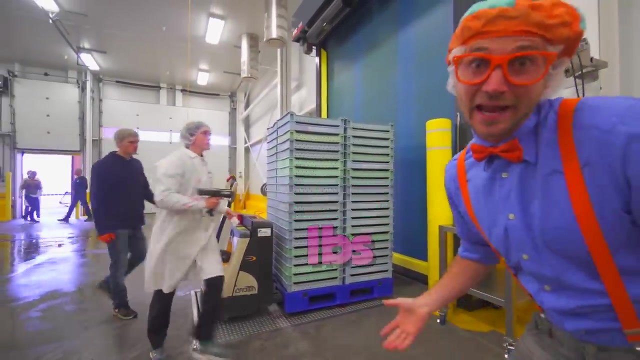 Oh, okay, so, Oh, like this one, Whoa, Buh-bye, Buh-bye. So what we're doing right here is we're taking a weight of these raspberries, See, Okay, now that we have them all weighed up. 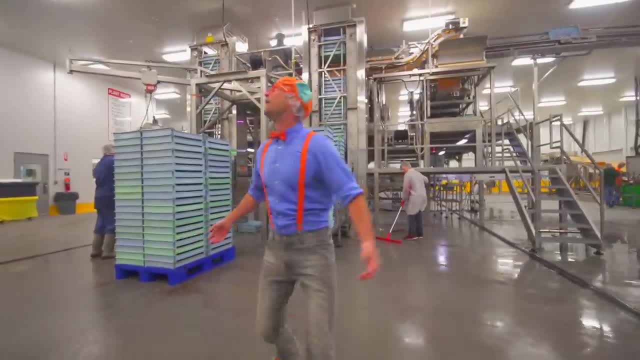 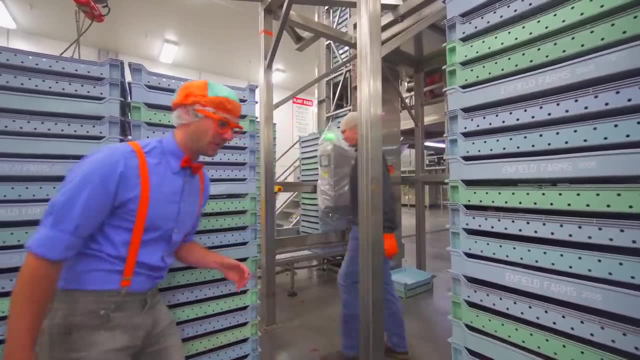 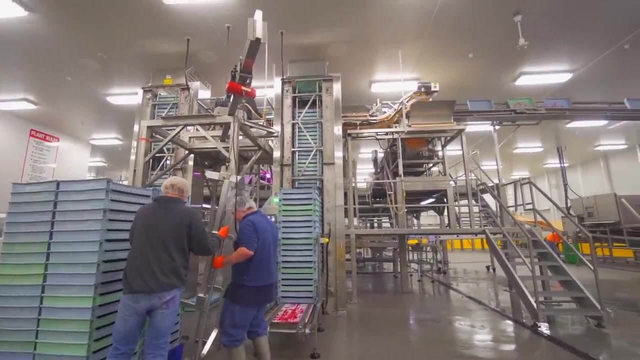 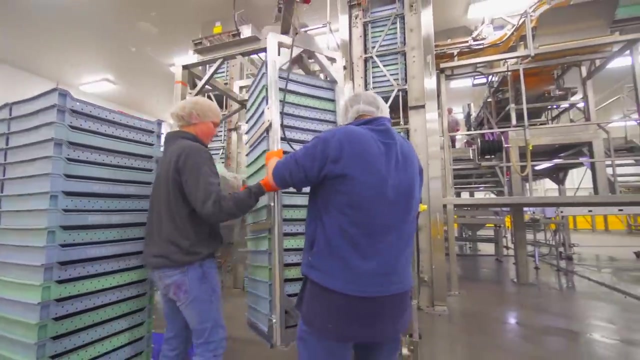 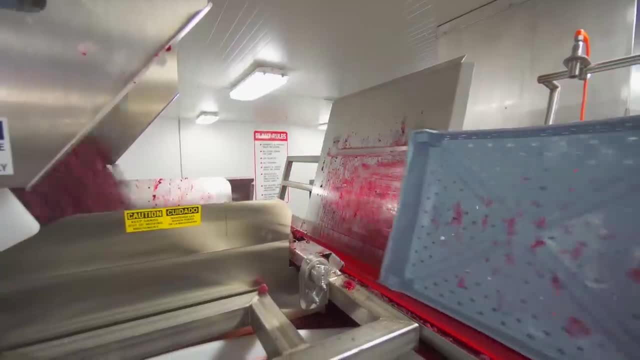 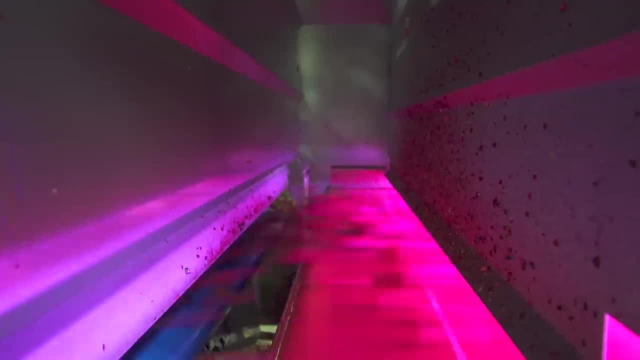 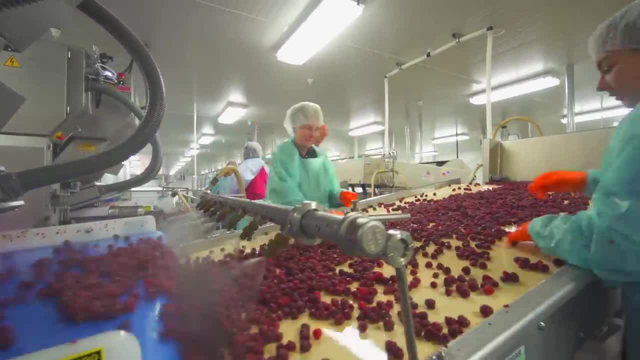 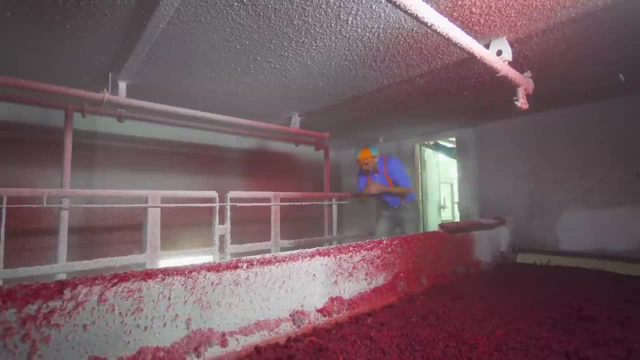 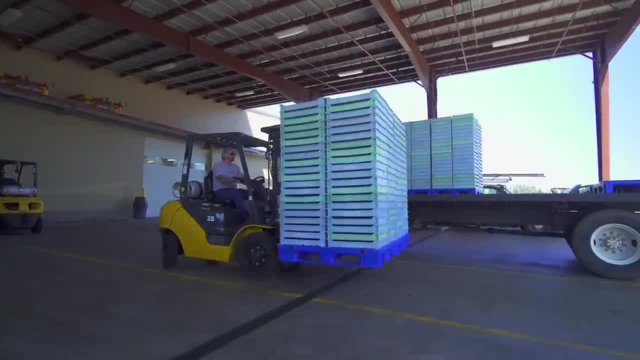 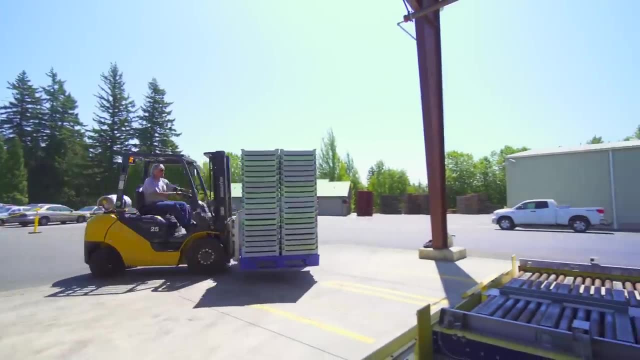 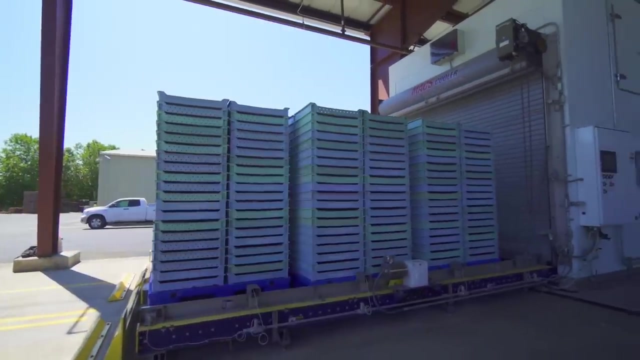 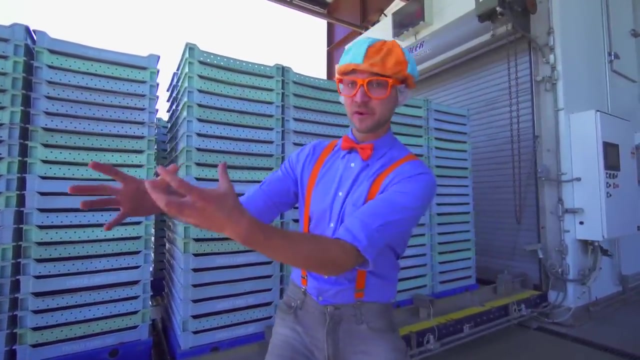 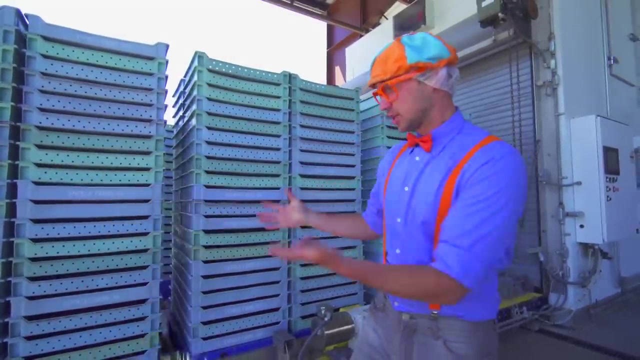 Whoa, Whoa, Whoa, Yay. Okay, so the raspberries came from the farm and got transported from the truck truck, And then a forklift pulled it off of the truck and loaded it up right here. And so now. 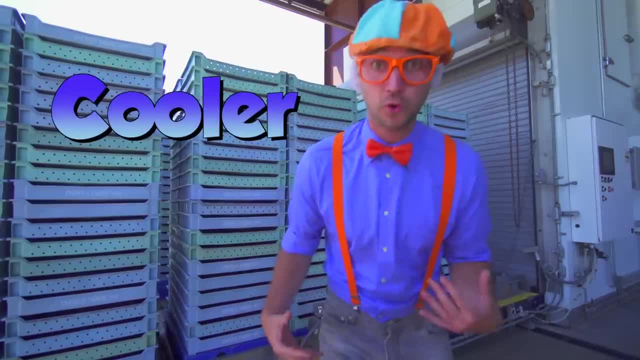 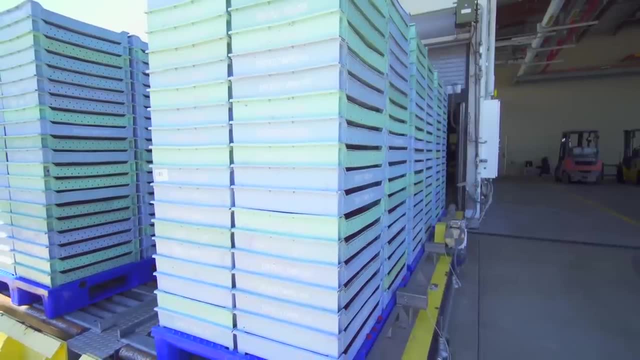 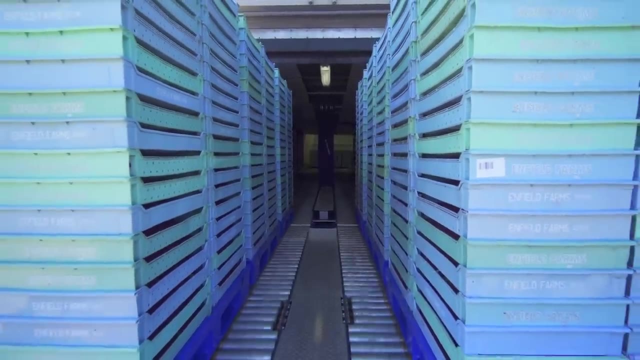 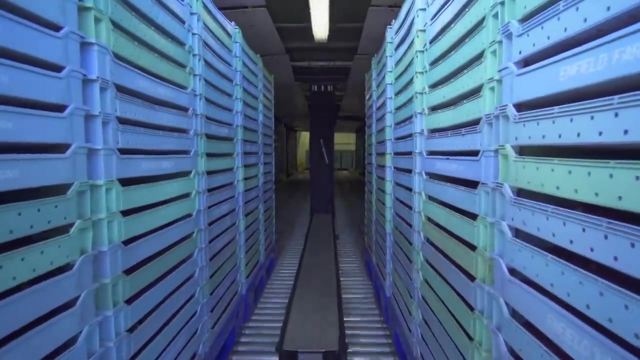 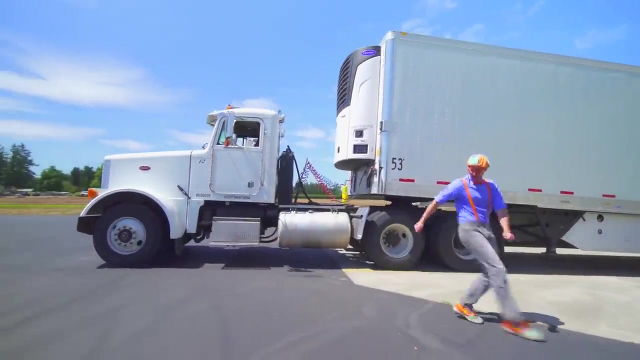 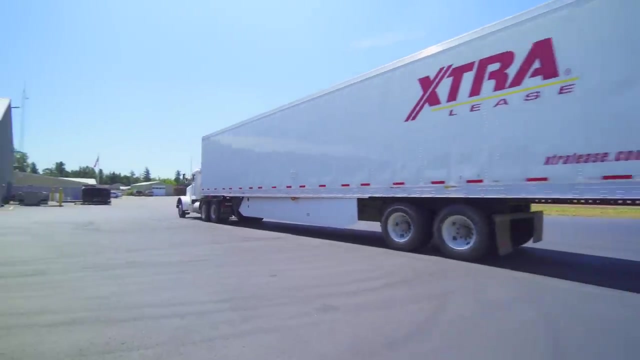 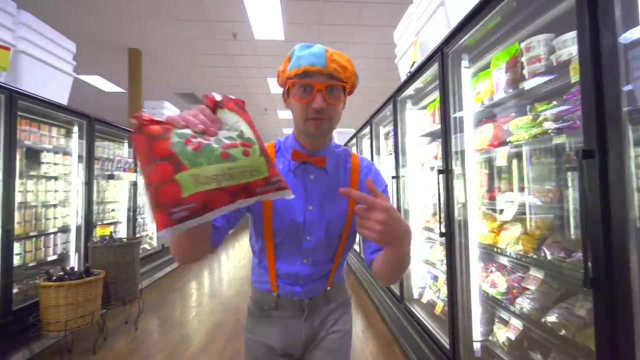 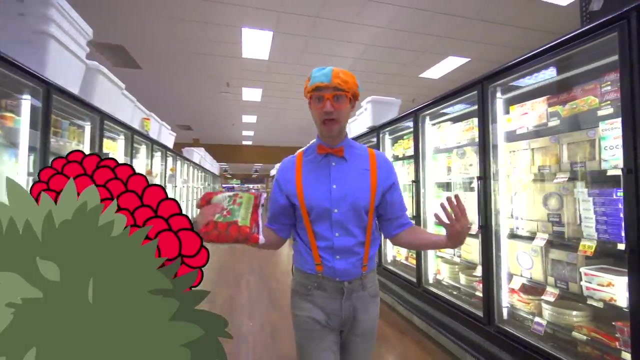 all of these raspberries are gonna go into this cooler Watch this. So that's how the frozen raspberries got all the way to the grocery store. They grew on the bushes really big, And then the harvester drove down the aisles of bushes. 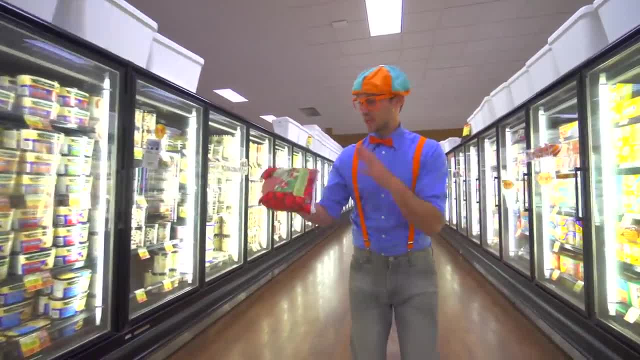 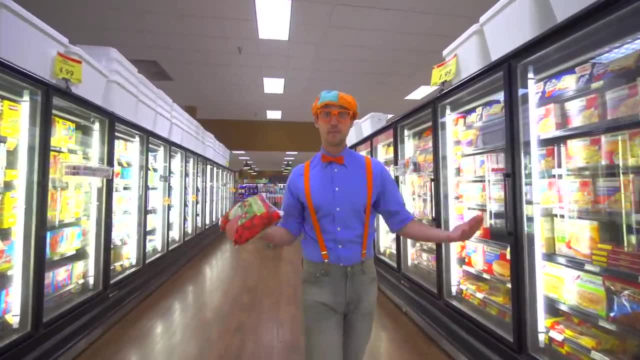 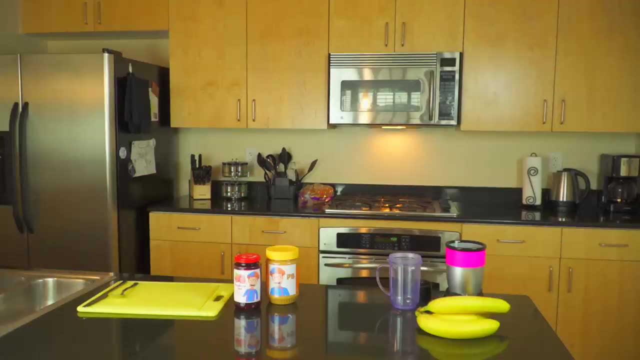 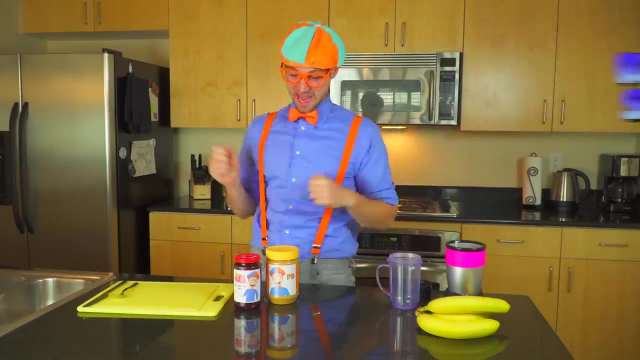 and shook them off, And then they got packaged up in these plastic bags. And then they arrived here. Hey, I think we should go make a frozen raspberry smoothie together. Alright, now it's time to make a Raspberry Smoothie and a raspberry sandwich. Yum, Alright, so let's make a sandwich first. 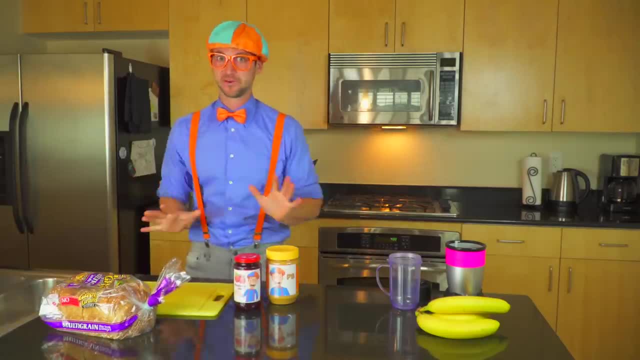 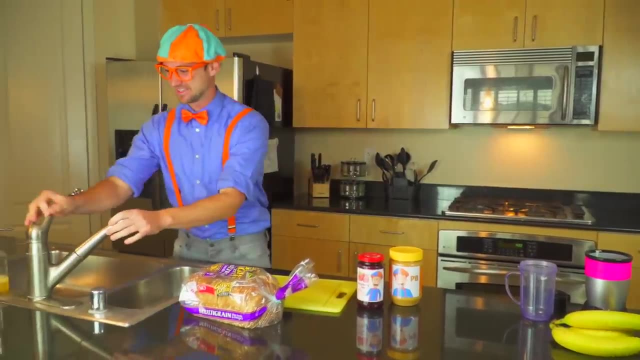 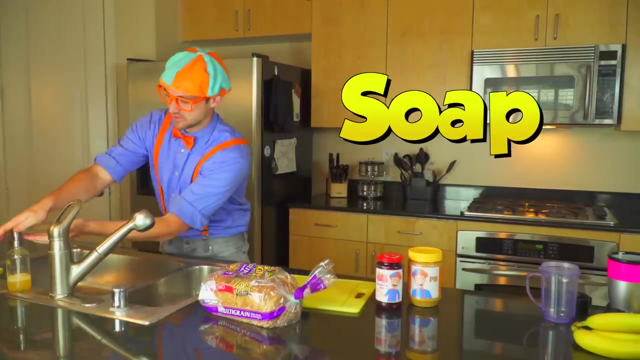 Alright, Whoa, whoa, before you touch food, you have to wash your hands. Let's go wash your hands. Alright, here we go get your hands nice and moist. Okay, whoa, Now you have to put soap on your hands and then you scrub it up. 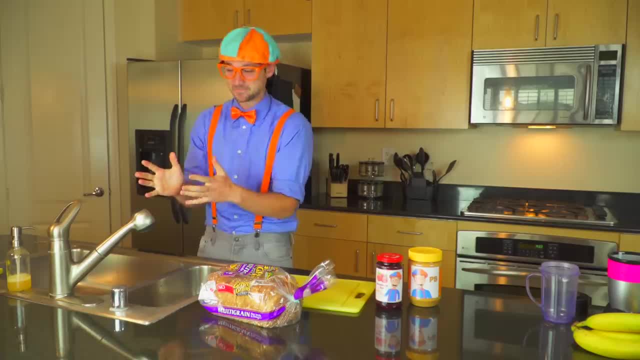 Dub, dub, but I'll tell you the correct amount of time. all right, You have to say blippy, blippy, blippy, and then you keep going faster and faster until you can't say it anymore. all right, Ready. 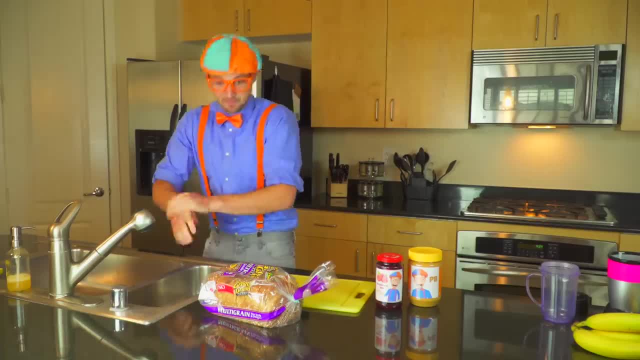 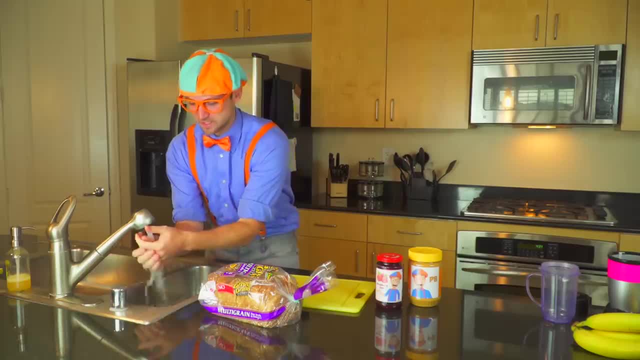 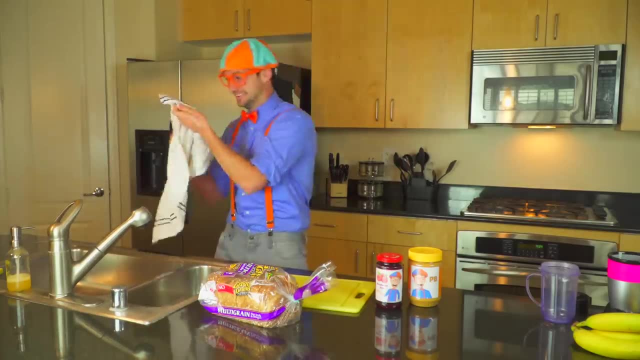 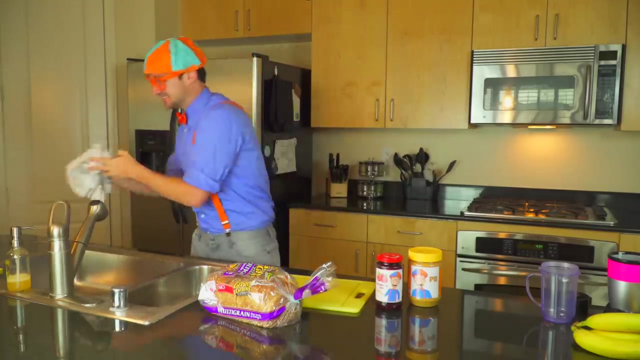 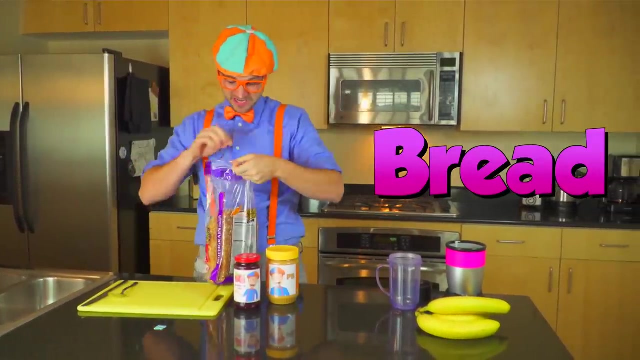 All right, whoa, Now you rinse the soap off your hands. All right, Dry off your hands. I am so excited for the food that we're gonna make together. All right, here we go. All right, let's get some bread for our sandwich. 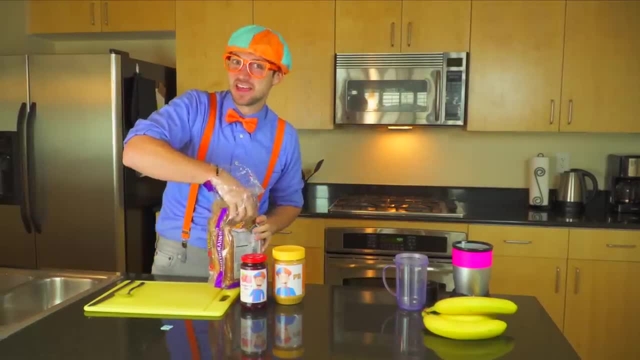 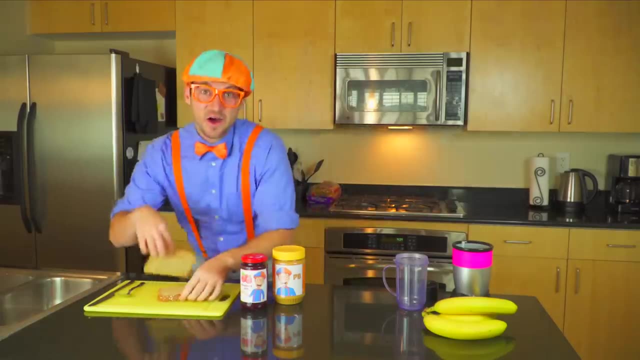 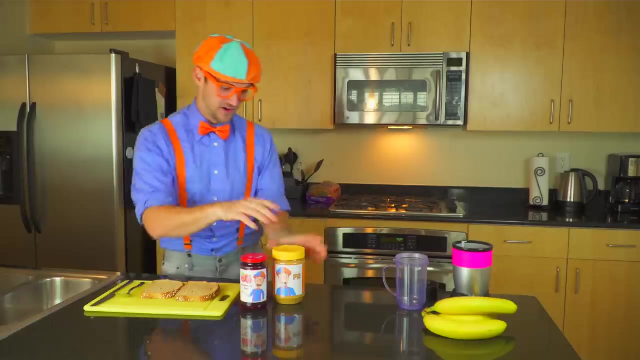 Ooh the heel. yum, I'll save that one for someone else, though. All right, there we go. One slice of bread. two slices of bread, All right, there you go. All right, let's start out with some peanut butter. 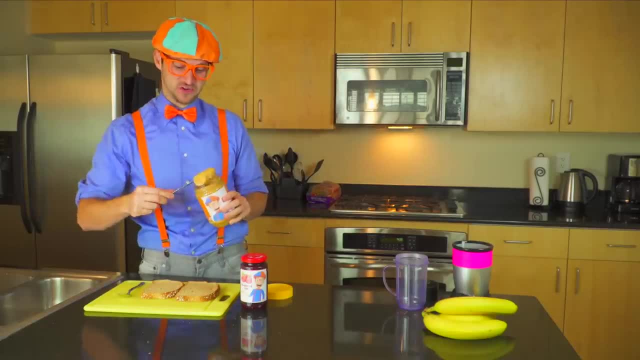 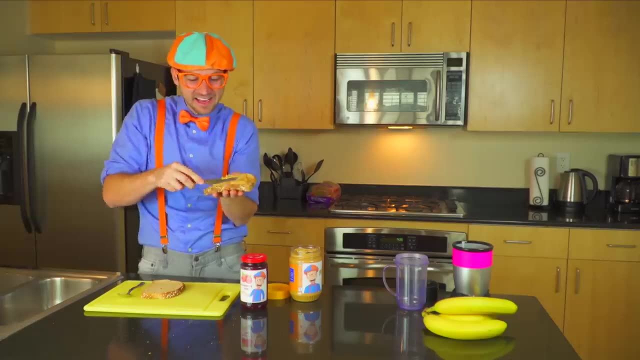 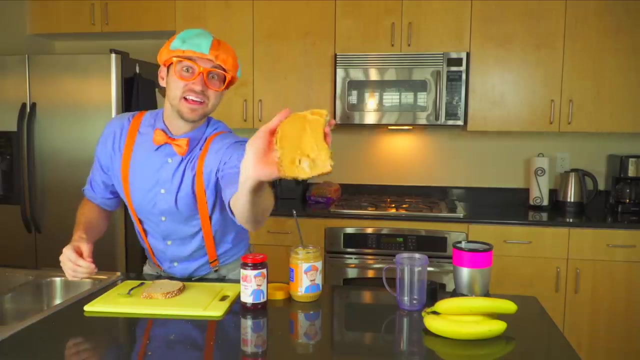 Yum, Take a big scoop. I love peanut butter. Okay, Okay, slop it around. Ooh, yeah, Look at that. Yum, Yum, Okay. and on this other side, we are gonna put some raspberry jam. 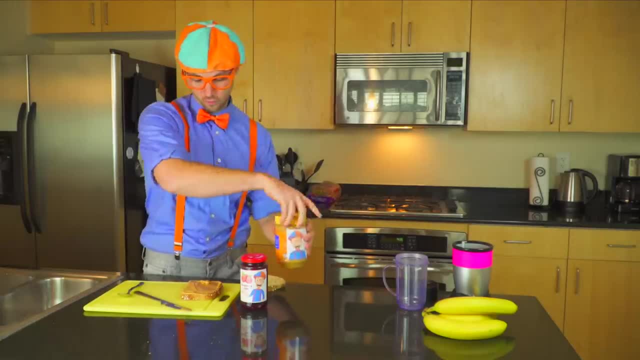 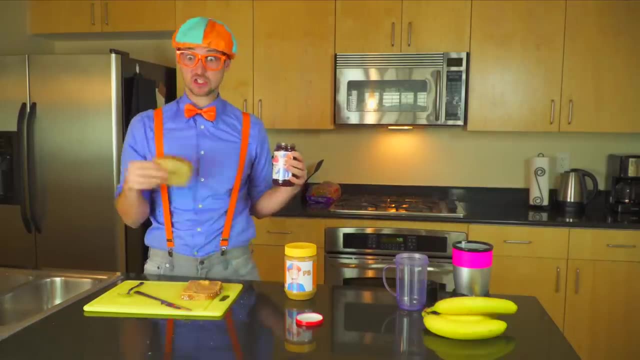 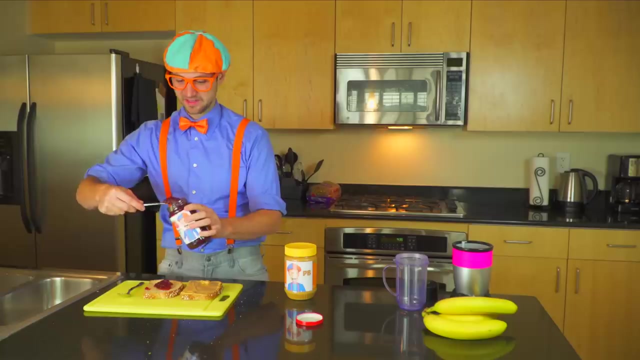 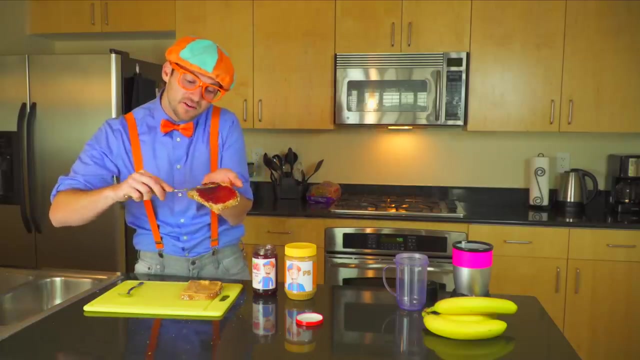 This sandwich is gonna taste so good. All right, take a big scoop of raspberry jam, Plop it right there. All right, Splash, Spread it around. Oh yum, Yum. All right, Put it down Boop-boop-boop-boop-boop-boop-boop. 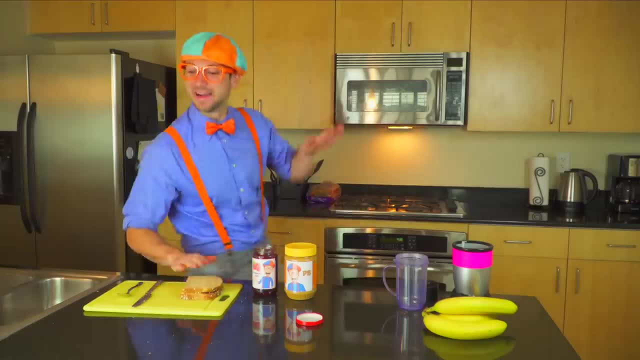 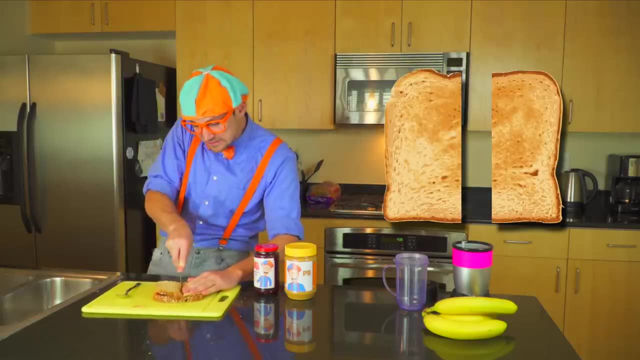 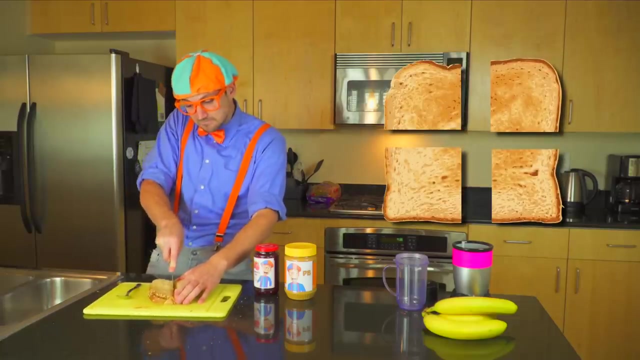 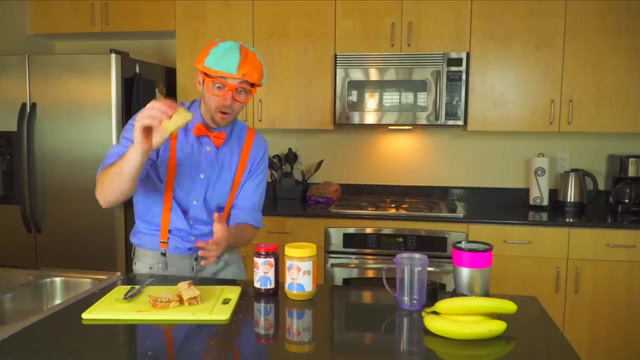 Put the lid back on. All right, here we go. Let's cut it in half, All right, and let's cut it into quarters. Oh yum, Yum, Yum. look at that. Whoa, All right, let's put this on a plate. 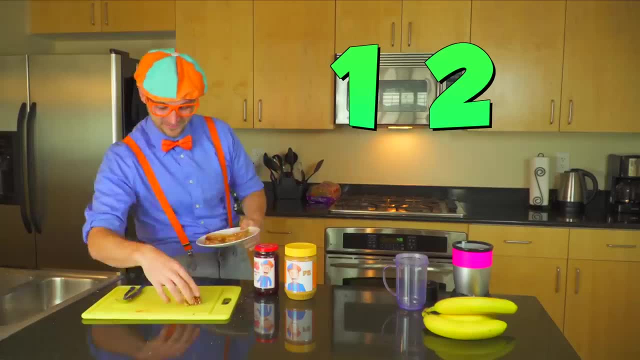 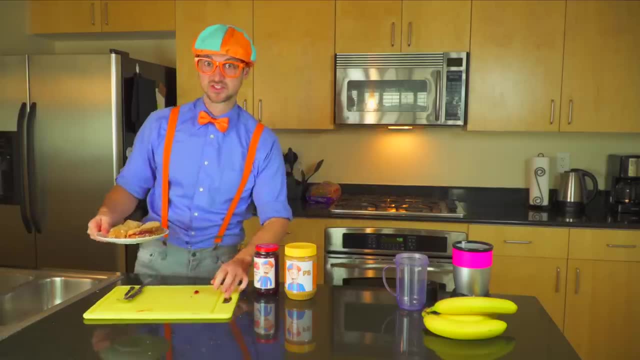 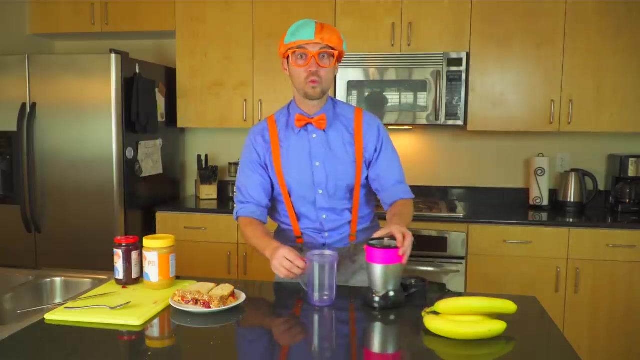 All right, One, two, three, four, Yum, All right. you know what Beverage would be so tasty with this raspberry sandwich? Yeah, a raspberry smoothie. Okay, now I'm gonna teach you how to make one. 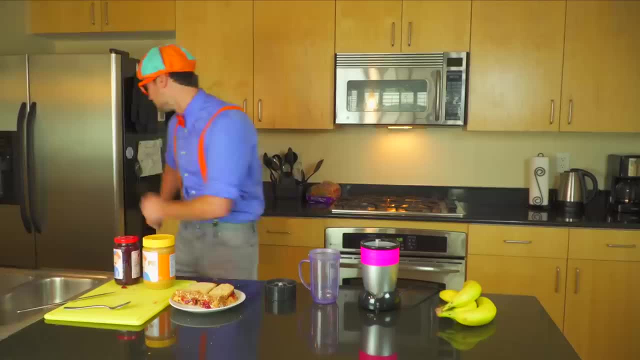 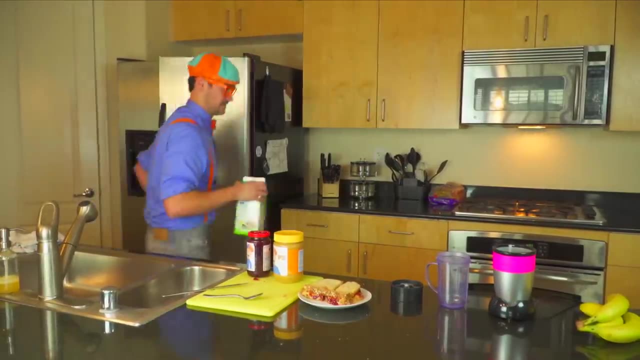 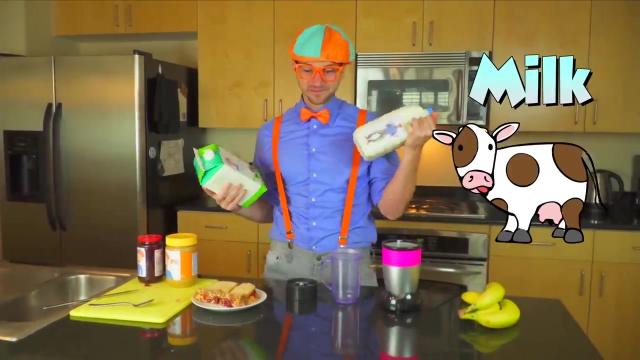 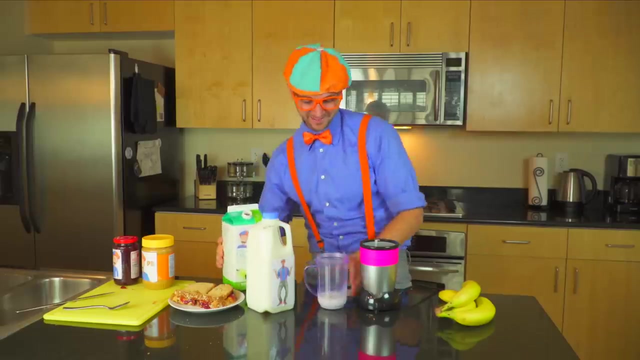 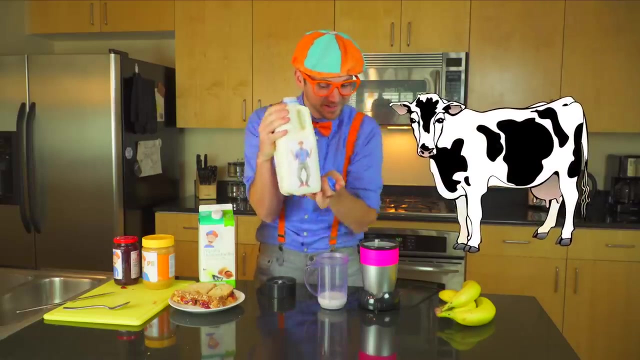 First we need to go get our milk, Hold on. Okay, so I have almond milk and normal milk, So let's put a little bit of almond milk in here. Perfect, that looks great. And let's put a little bit of normal milk in here. 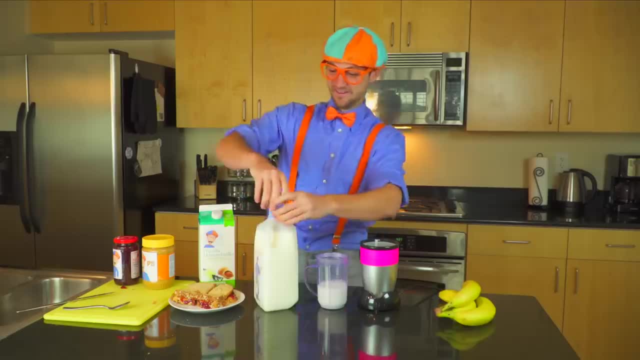 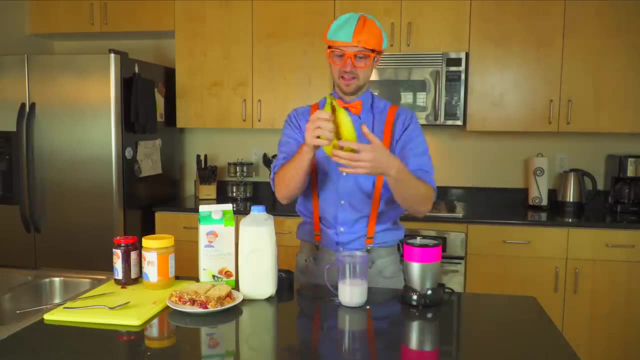 Whoa, okay, perfect, I spilled a little. Look, that's okay, we'll clean it up after All. right, and let's take a banana. Let's actually cut it in half, because you know I don't want to spill it. 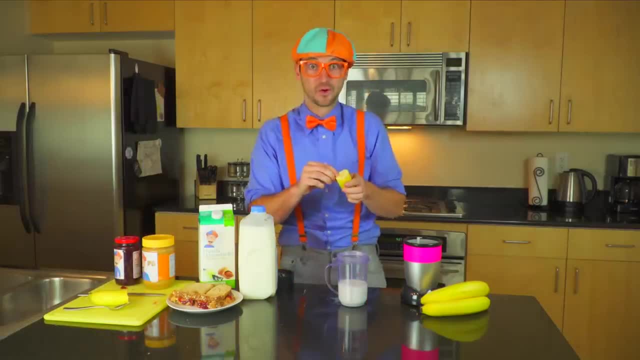 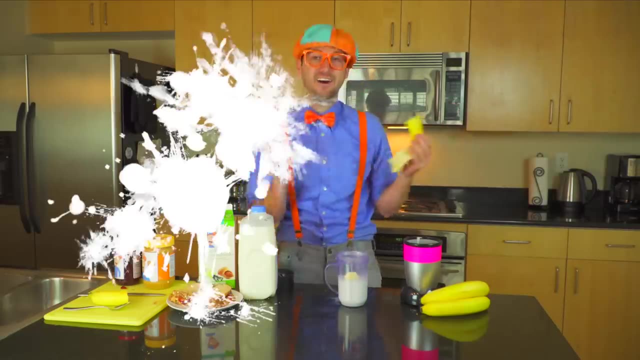 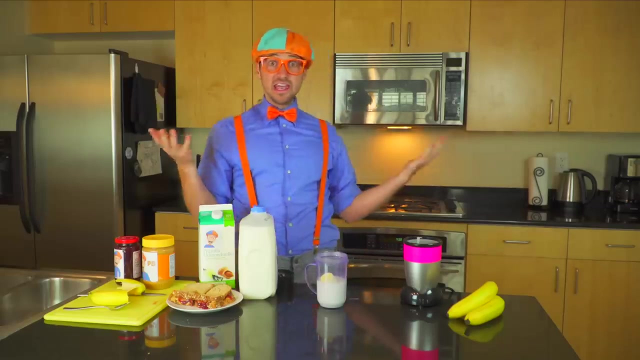 I don't want to spill it. That's a lot of banana. I want more raspberries than banana, But I still do like banana Bombs away. All right and wait. what are we missing here? Yeah, raspberries. 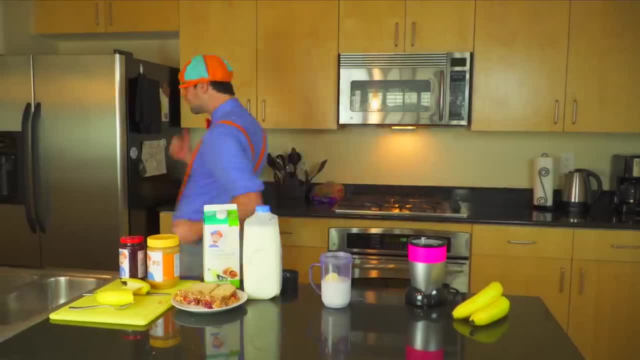 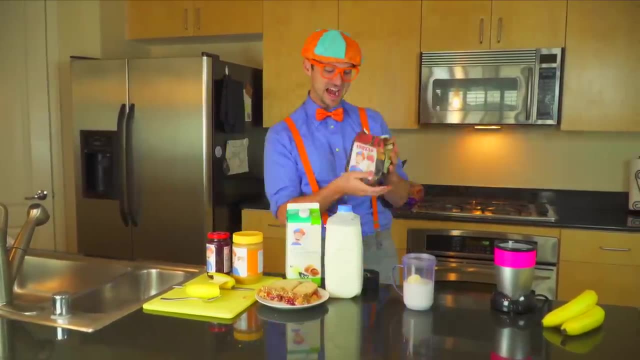 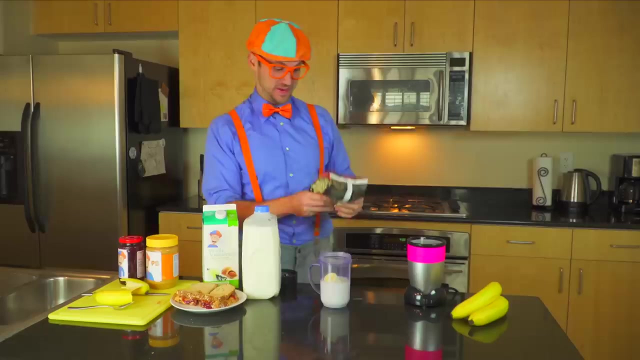 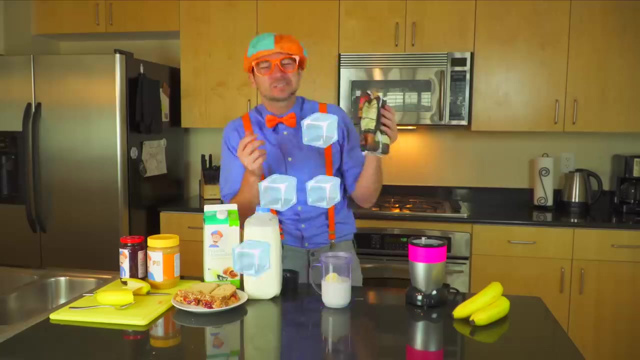 Okay, I need to go get them from the freezer. Woo Yeah, frozen raspberries. I use frozen raspberries because they're really good in here, because then it makes it nice and cold and then it feels like little ice chunks. All right, how do we open this? 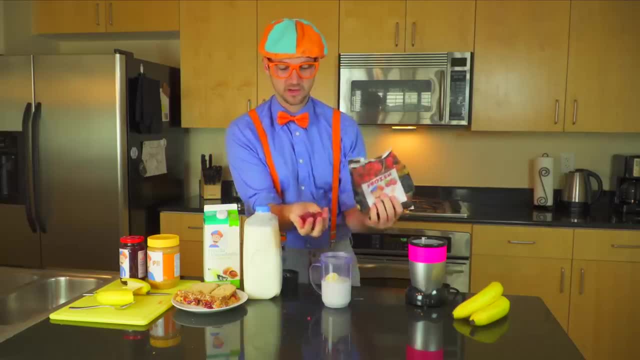 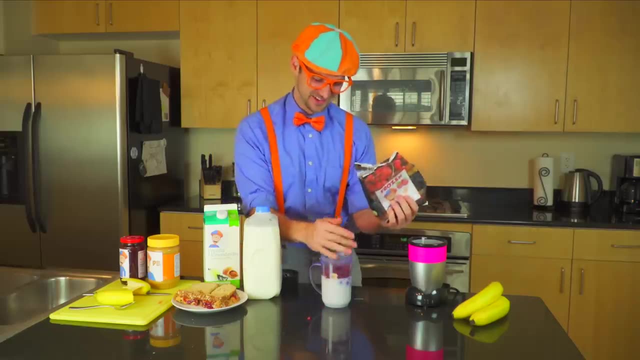 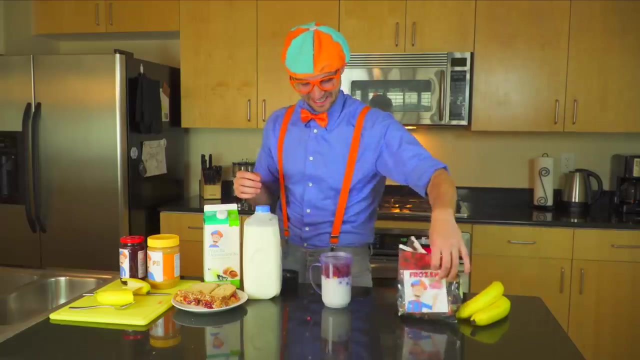 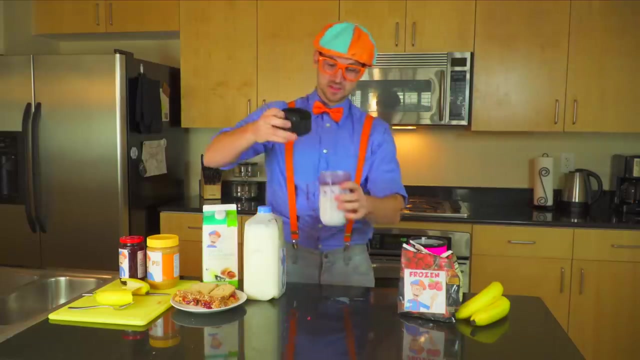 There we go. All right, the correct amount is one handful. No, it's two handfuls. Yeah, there we go. Yeah, Okay, there we go, And let's add a little bit of extra almond milk. Perfect, All right, let's put the lid on. 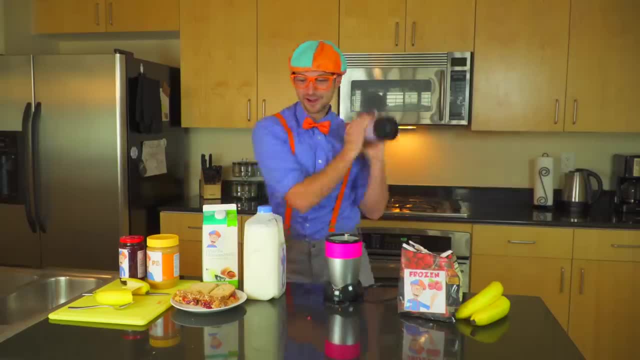 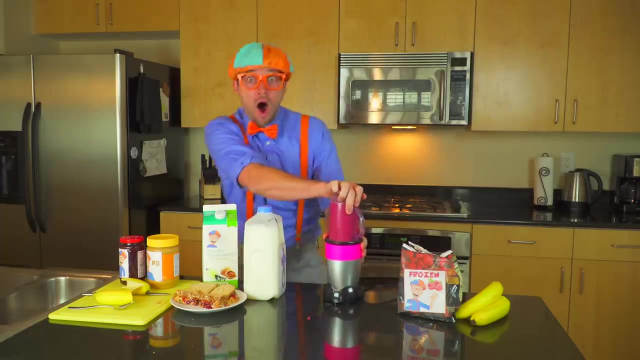 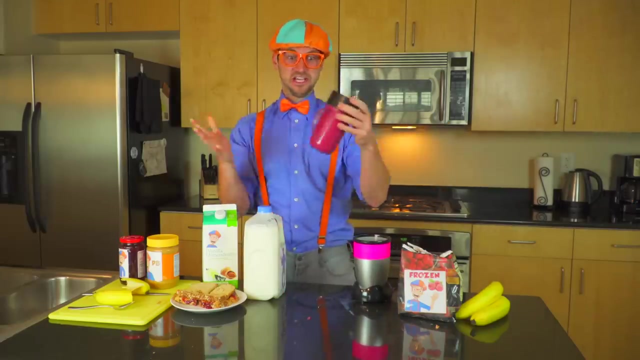 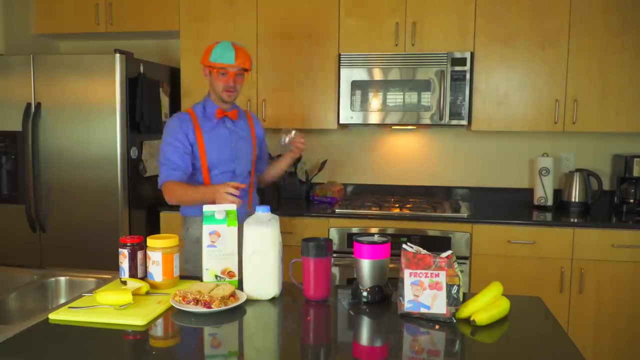 Give it a little shake. Yeah, All right, now let's blend it on up. Woo Woo, Wow Yum. That looks so tasty. Okay, I'm gonna get a glass Perfect Yum. All right, I'm gonna pour a smoothie. 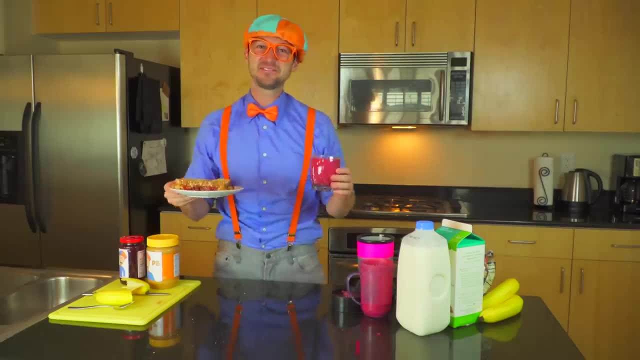 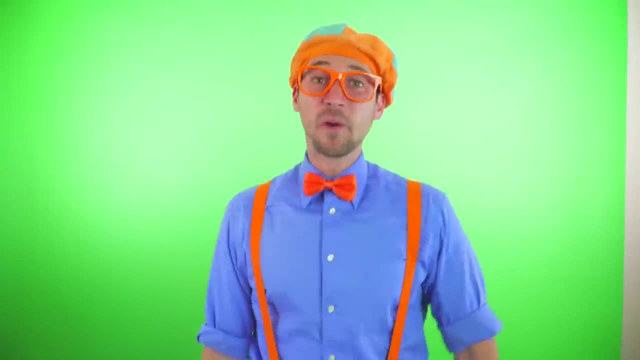 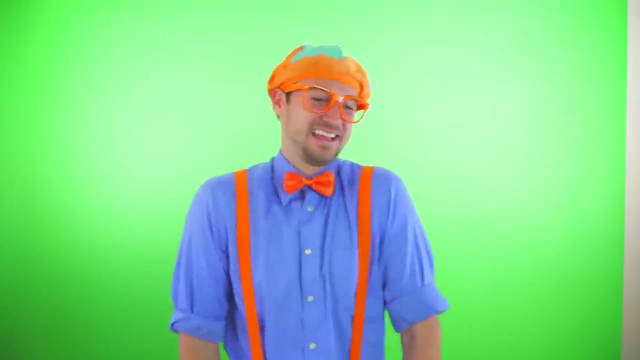 Yum. All right, now it's time for the raspberry song. Come on, everybody, Sing along with me. Raspberries, I think they're very, very yum. Raspberries are very yum Raspberries. I like them very, very much. 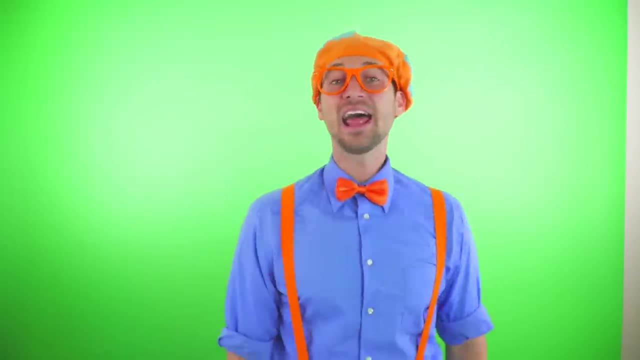 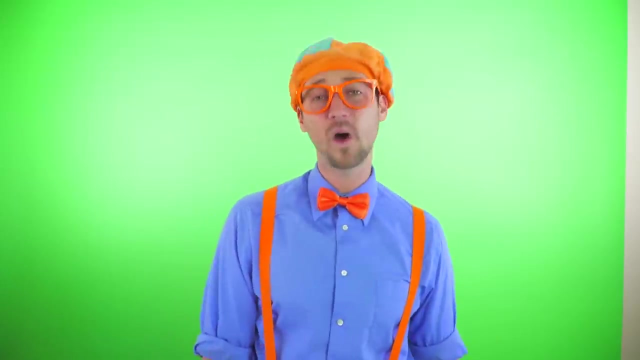 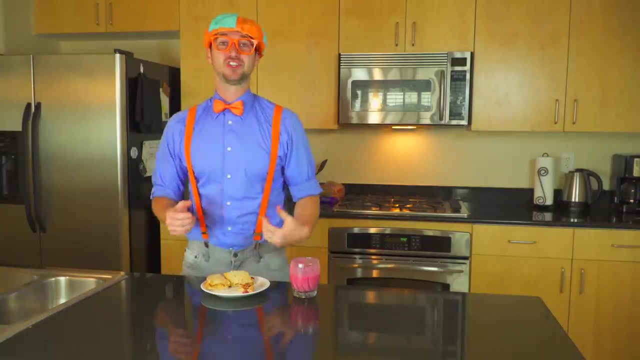 I like them, Raspberries. I like them very, very much, Raspberries. let's spell it one more time: R-A-S-P-B-E-R-R-Y. Yum, This food is so tasty. Well, I sure did have a blast learning with you. 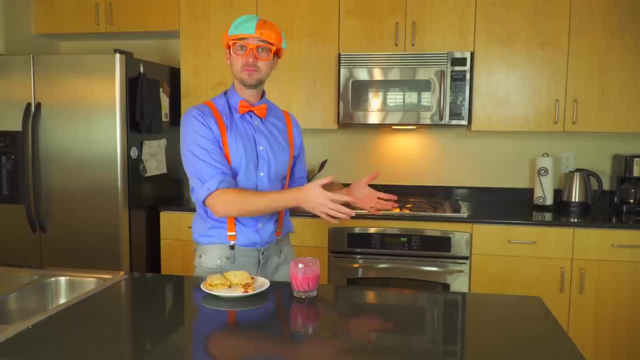 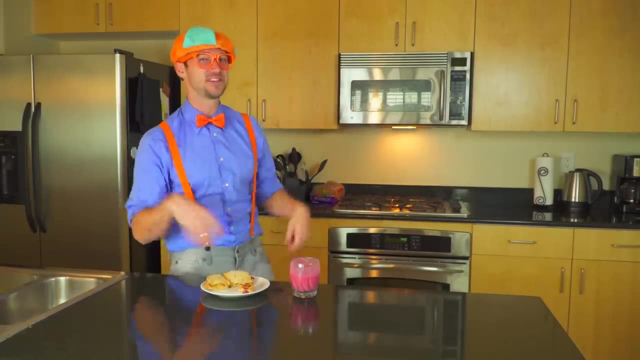 about how raspberries go all the way from the farm to your tummy. Well, if you want to watch more of my videos, all you have to do is click the subscribe button. I'll see you next time, Bye, Bye, Let's do a search for my name.